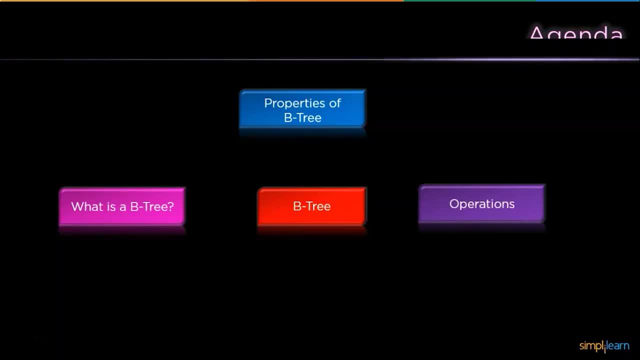 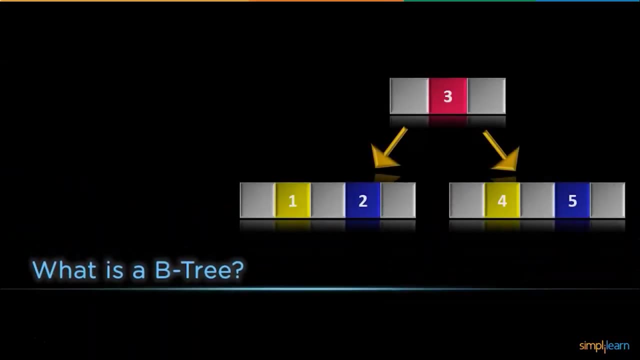 operations on them, like searching, insertion and deletion. Finally, we will sum up what we have learned from this session, But before we begin, make sure you have subscribed to our YouTube channel and clicked on the bell icon below, So you never miss an update from: 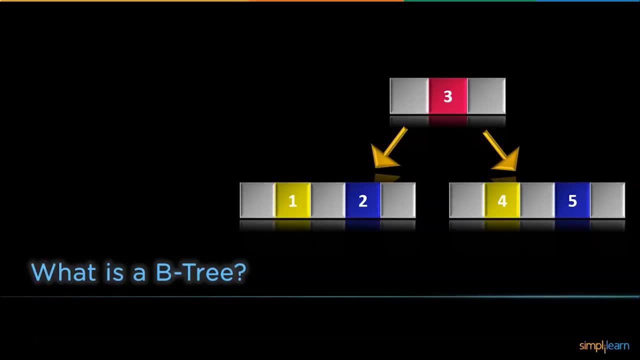 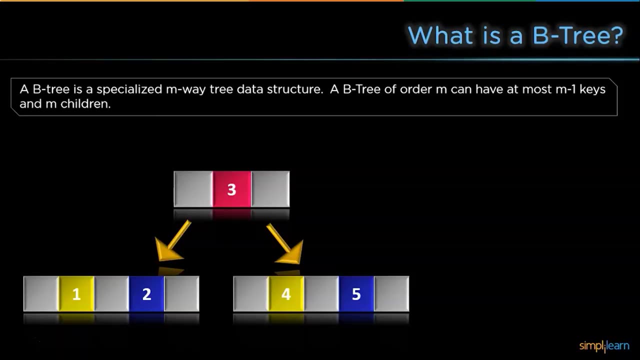 Simply Learns. So, without any further ado, let's get started with what is B-tree? A B-tree is a special M-by-tree data structure. A B-tree of order M can have at most M-by-tree data structure. A B-tree of order M can have at most M-by-tree. 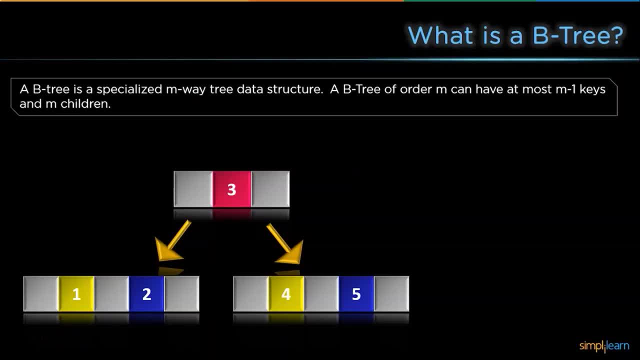 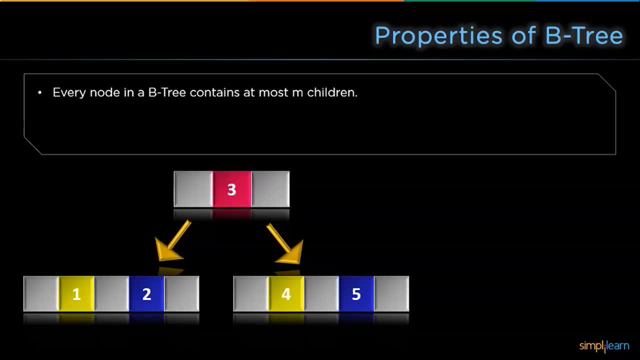 features like Cence2 and Cce1, keys and M children. Now lets discuss some properties of B-trees. First up, every node in a B-tree can have, at most M elements. Next, every node except the root and the leaf node must. 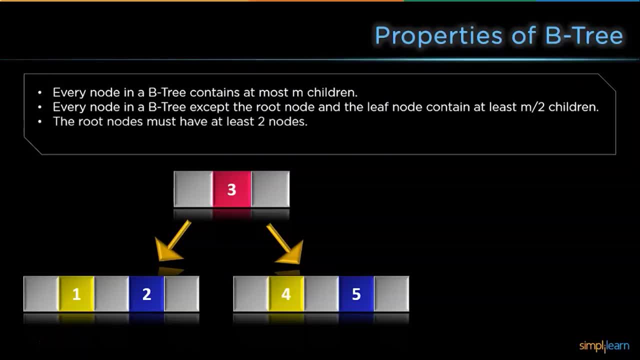 have M by 2 children. Next, a root node must have at least 2 nodes At last. the leaf node must be at the same number of B-tree nodes. Next, a root node must have at least 2 nodes At last. a leaf node must be at the same level. 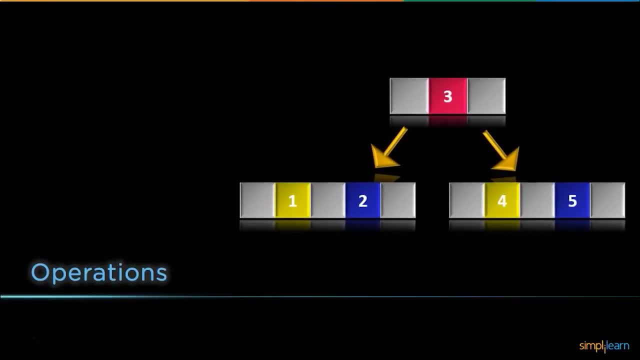 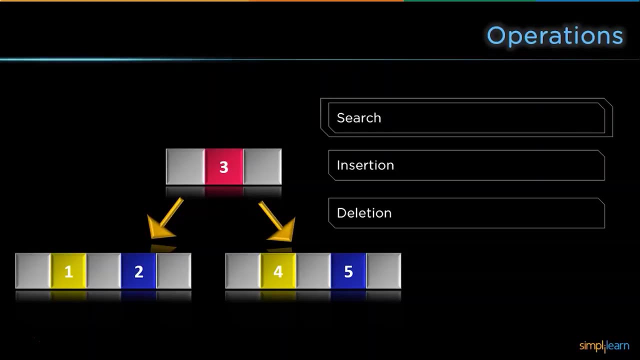 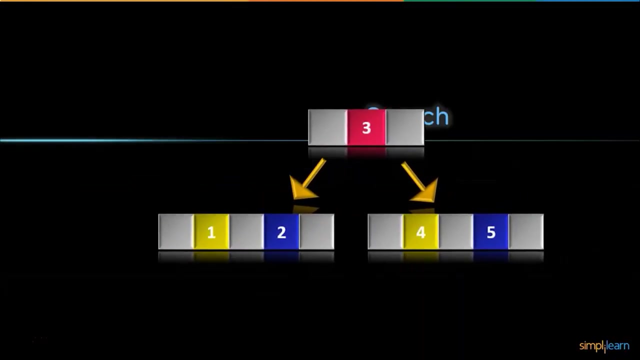 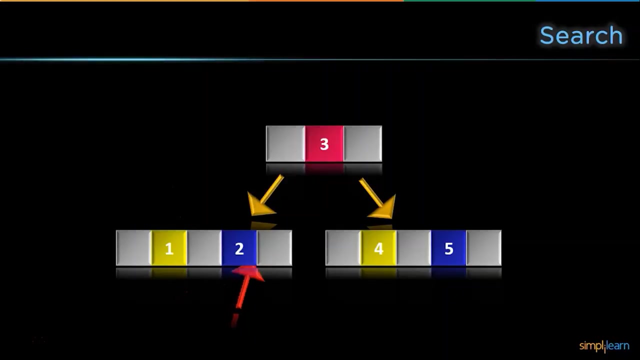 Now let's discuss what are the various operations we can perform on a B-tree. We can perform three operations on a B-tree, ie searching, insertion and deletion. Let's discuss these in detail. First up, searching. In this we will traverse the complete B-tree until we have found a key. 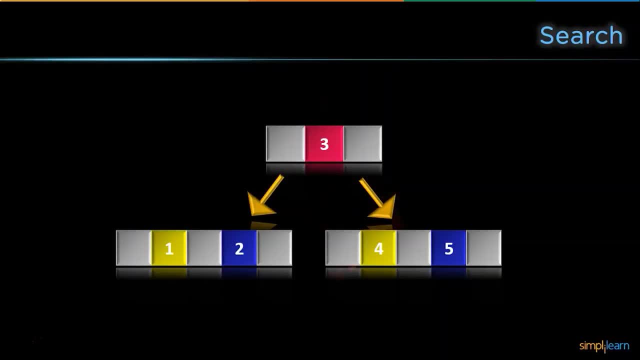 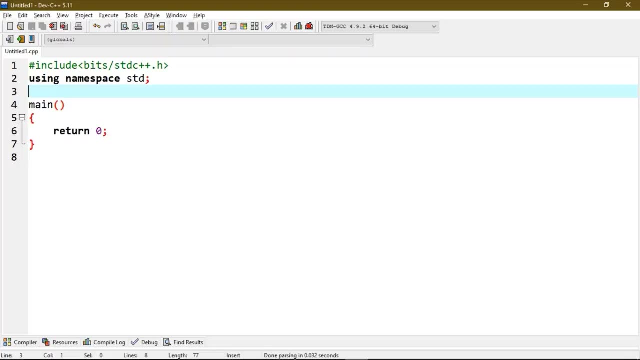 We will start from the left side to go all the way up to the right side. Now let's try this in a code editor. We will first start by creating a B-tree node. To do that, we will use class B-treeNode- int keys. 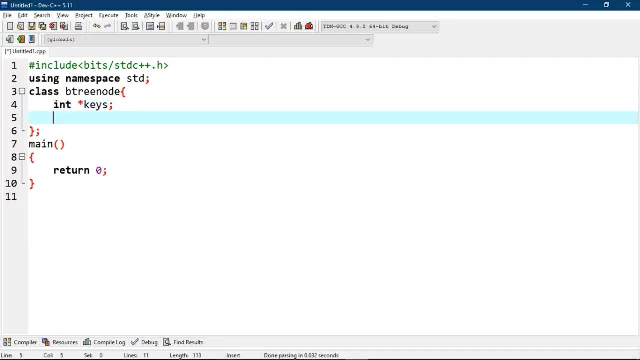 It is an array of keys, Then int t. This will define the range of the number of keys. Then we will create a child pointer, B-treeNode t. It is an array of child pointer, Then int t, Then a variable to check the current number of keys. 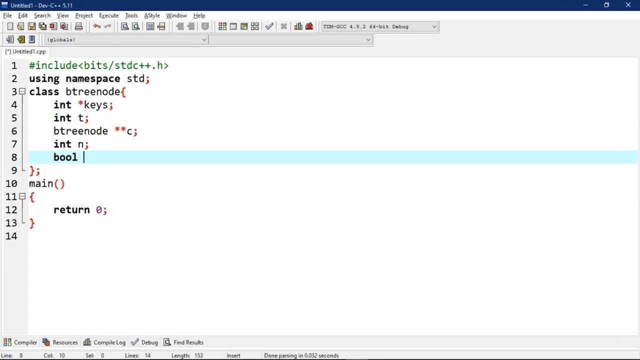 And a boolean variable which will be true when the node is leaf. We start from here. We will start from here, Then int t. Now define some functions in public: First constructor, Then a function to insert a new key in a subtree. 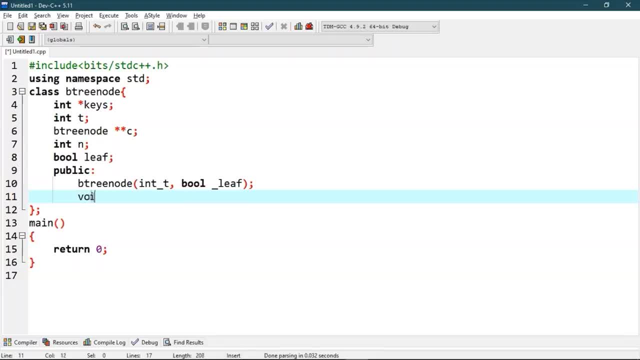 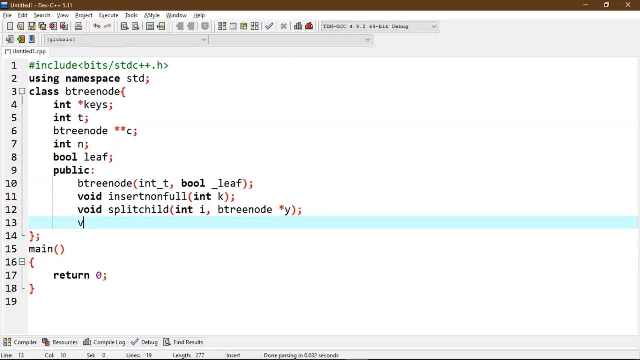 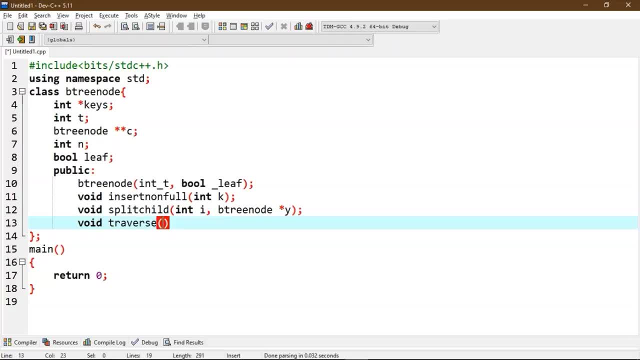 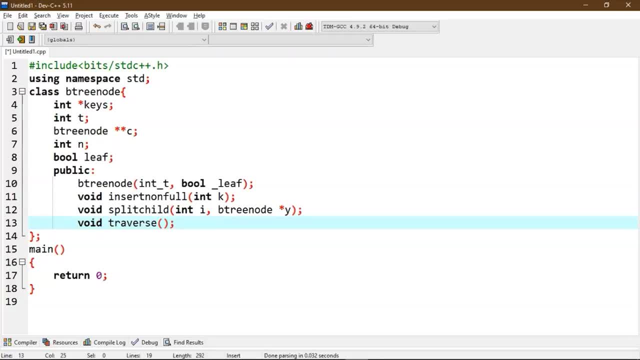 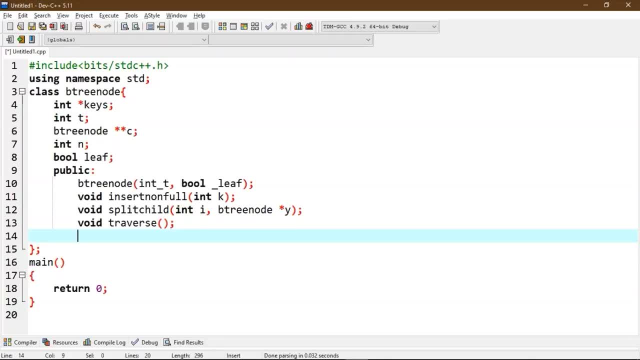 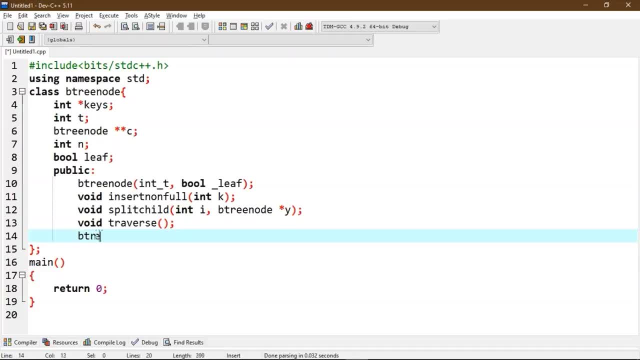 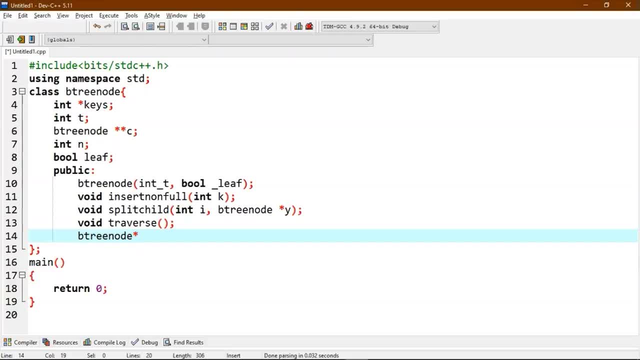 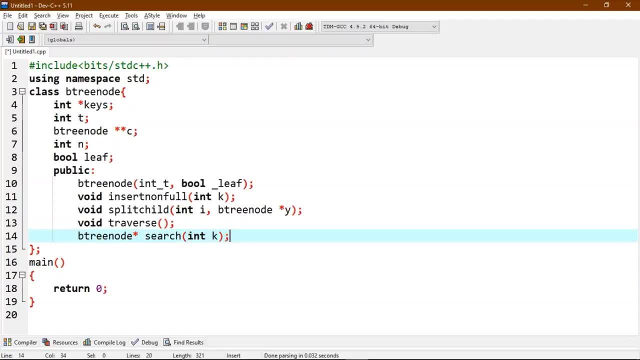 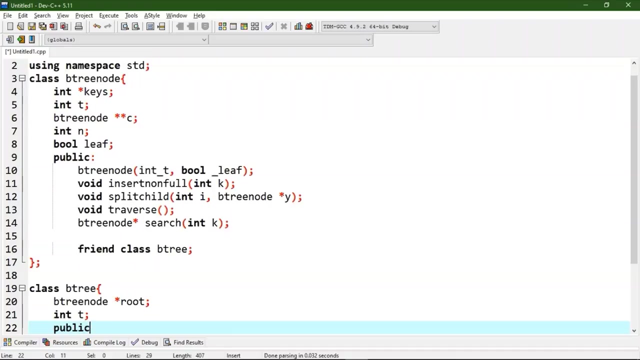 Now we will create another class btree. make it a friend of this so that we can access private members of this class in btree function. Now we will create a pointer root, minimum degree, then public, and then we will create a constructor btree. 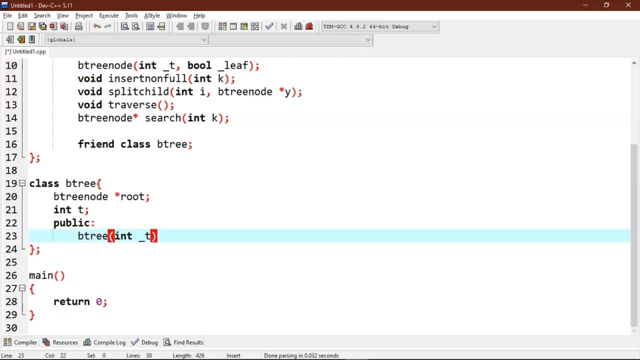 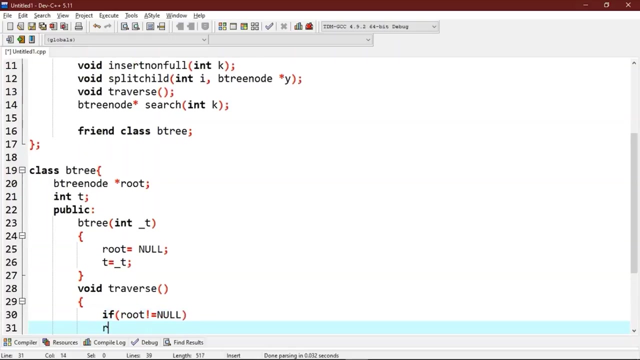 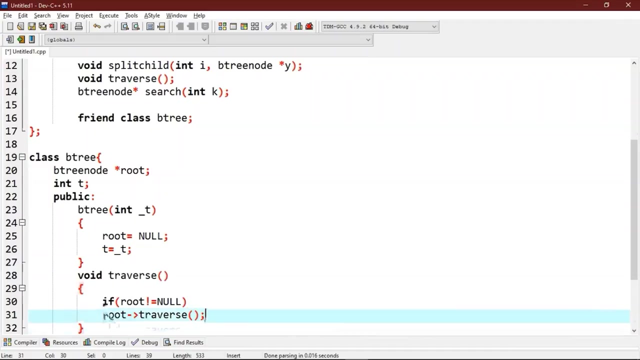 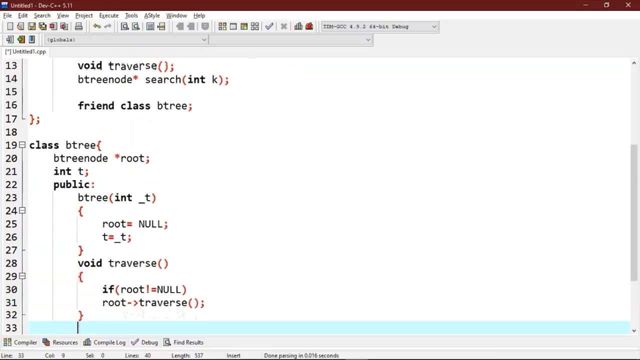 root equals to null and t is equals to- let's call it t. Now we will write a function to track the function. Traverse this tree Traverse. if not null, Then root traverse. Now we will write a function. 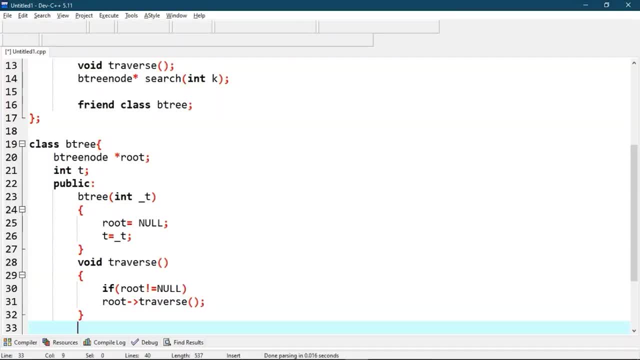 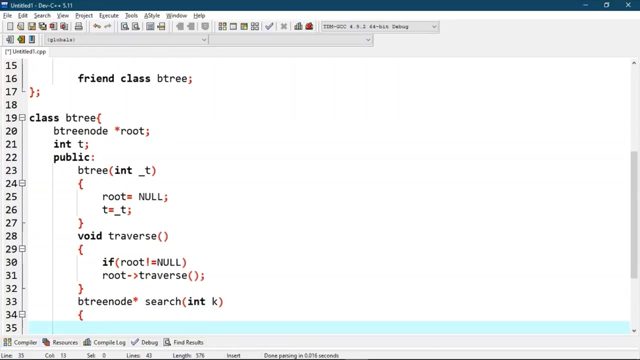 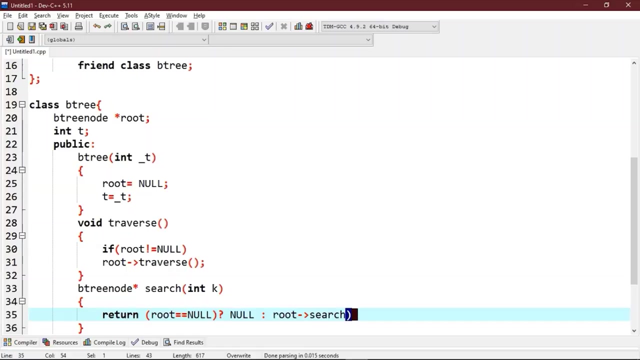 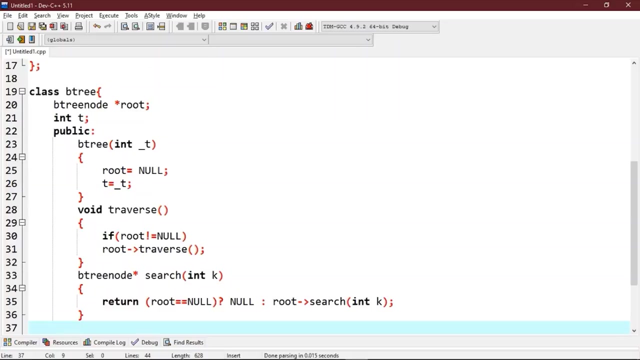 To search a key in this tree. To search a key. To search a key in this tree if root is equals to null and null else. root search. root search now the main function that inserts the new key in this btree. void: insert print k. 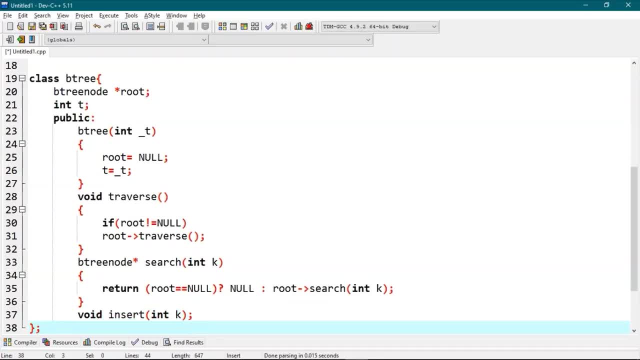 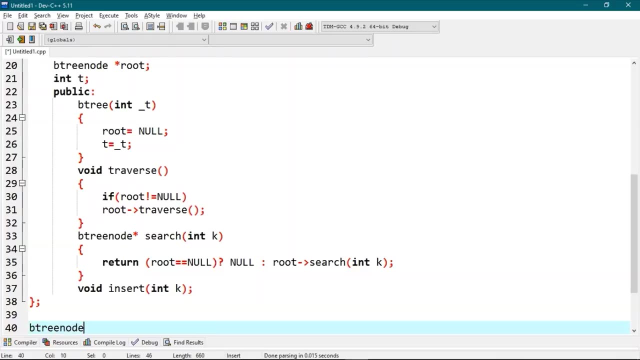 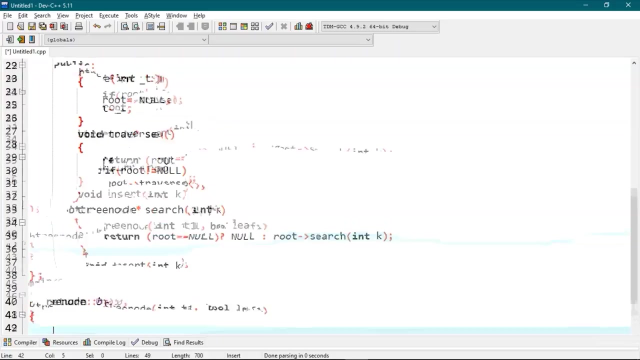 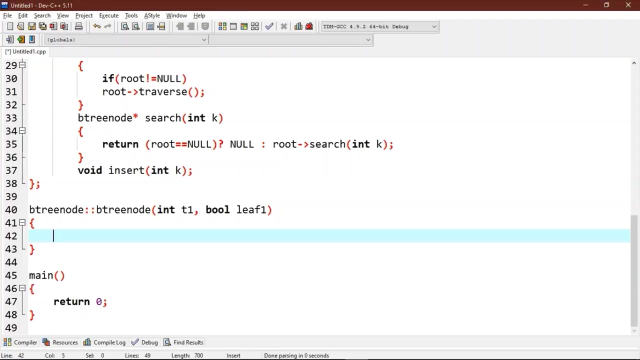 now we will write the constructor for btree node class. now we will write the constructor for btree node class. now the main function that inserts the new key in this btree node class. now we will copy the given minimum degree and leaf property. now we will copy the given minimum degree and leaf property. 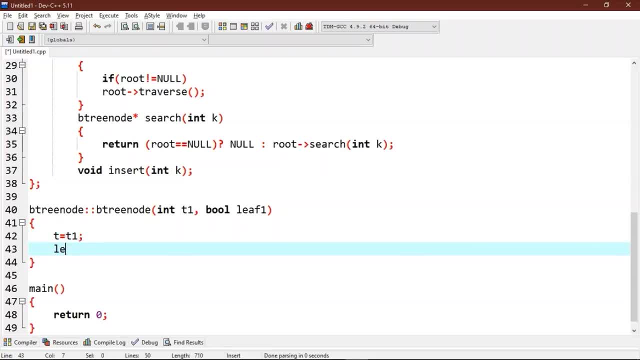 now we will copy the given minimum degree and leaf property …. … now we will allocate the memory of each maximum spann point …. … number of possible keys. and the child pointer and c equals to new btree code star bracket two, star t. now we will initialize the number of keys as zero. 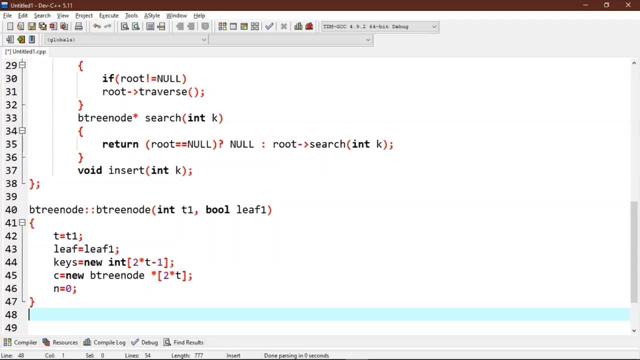 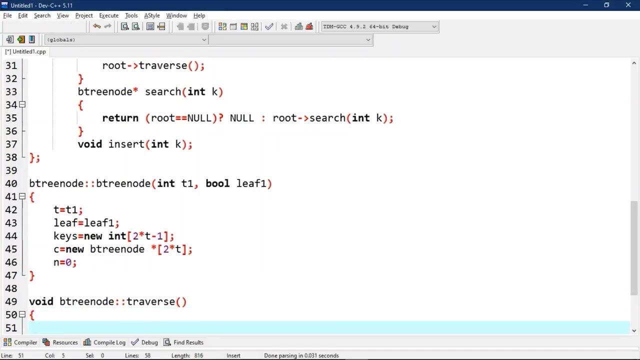 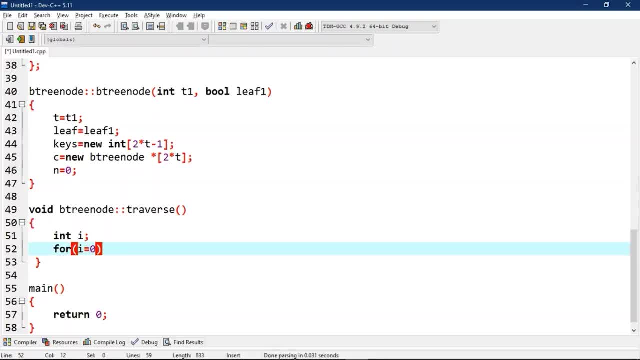 now let's write the function to traverse all node in the sub tree rooted with this node. i is equal to zero, i less than n, i plus plus. if this is not leaf node, then, before printing key, traverse the sub-tree rooted with child c, i. 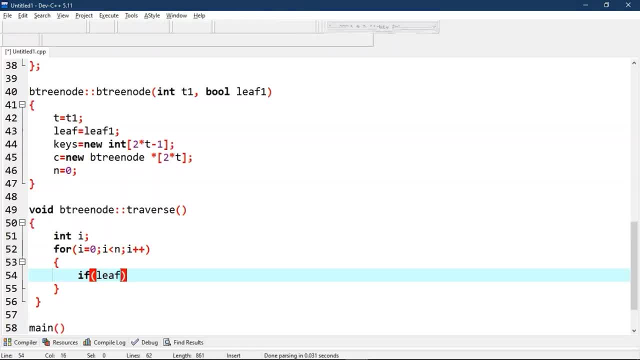 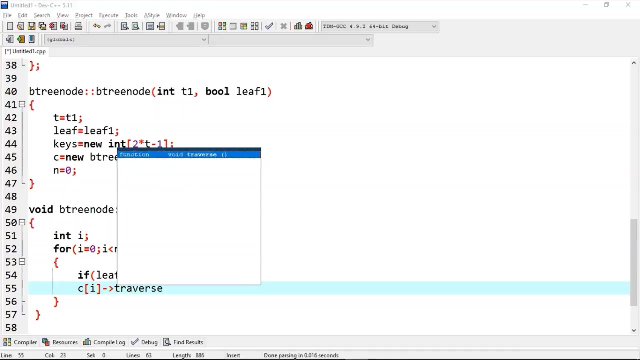 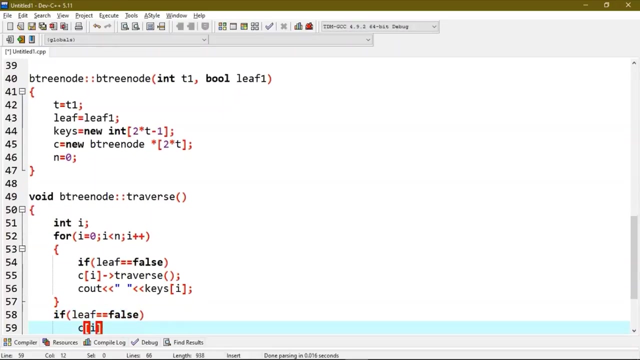 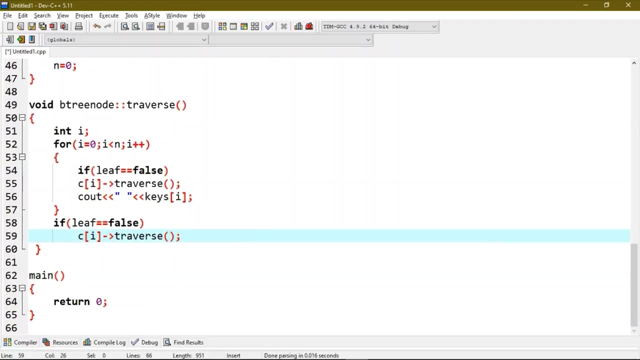 So if leaf is equal to false, then c bracket i is equal to traverse. Let's cout case: now we will print the sub-tree rooted with the last node. So if leaf is equal to false and c i traverse, Now we will write the function to search key k in sub-tree rooted with this node. 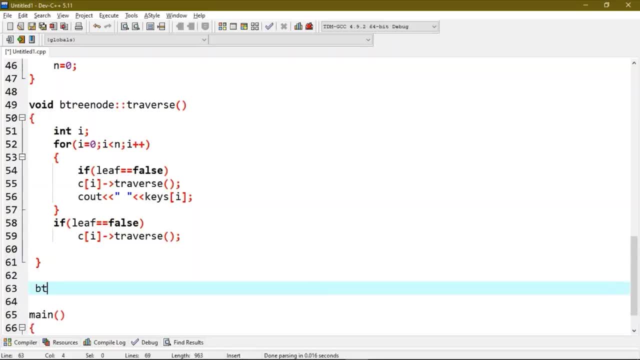 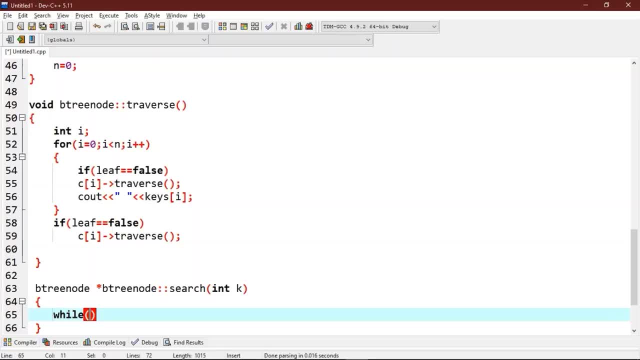 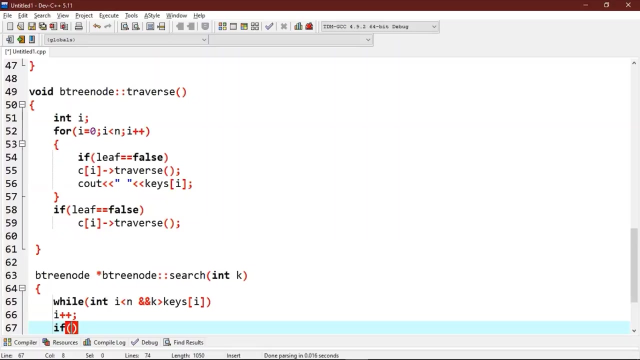 So while int i is less than n and k is greater than is bracket i, then i++. Now, if we found the key is equal to k, then we will return this node. If bracket i is equal to k, then we will return. 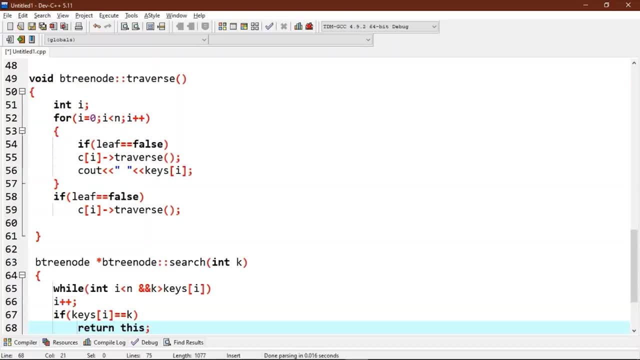 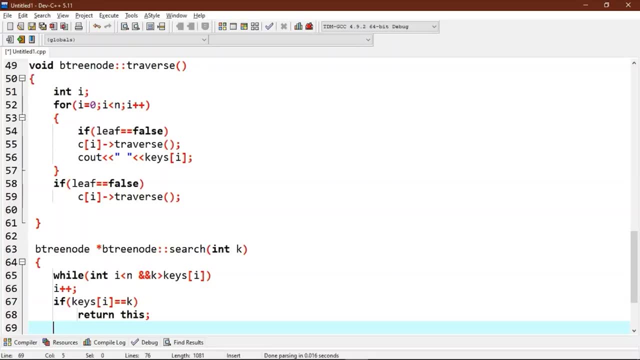 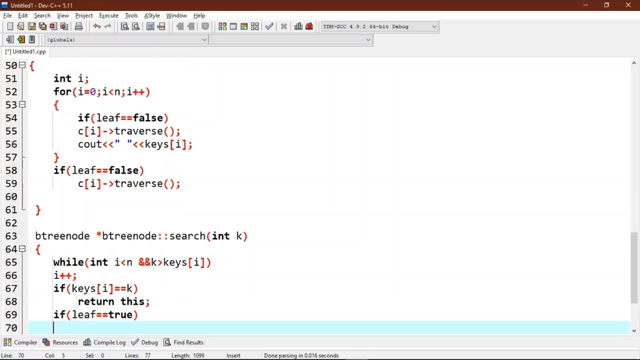 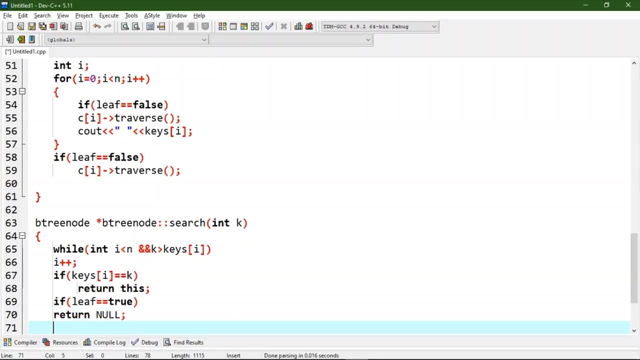 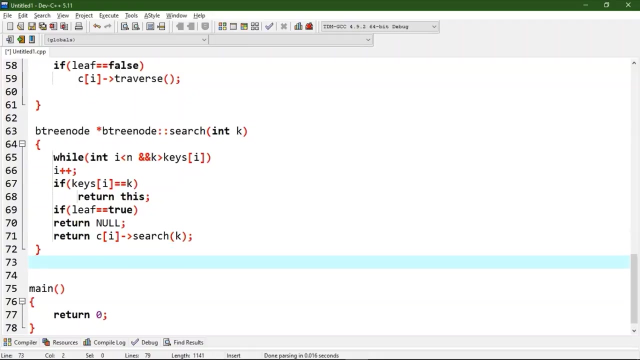 the If key is not found here and this is a leaf node, then if leaf is equals to true, then we will return L. Now we will try to go to the appropriate child, so we will use return C, bracket I arrow search. Now we will write the bean function that insert the new key in this Vtree. 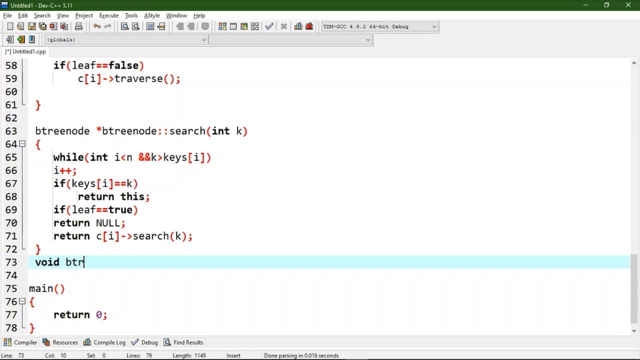 So void Btree, insert int k. Now we will write the bean function that insert the new key in this Vtree. So void Btree, insert int k. Now we will write the bean function that insert the new key in this Vtree. So if root is equals to null, then we will allocate the memory for root. 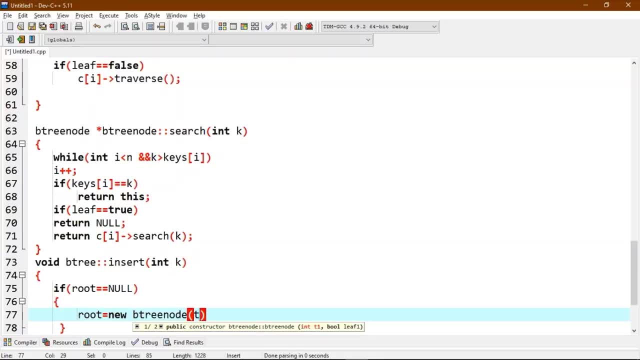 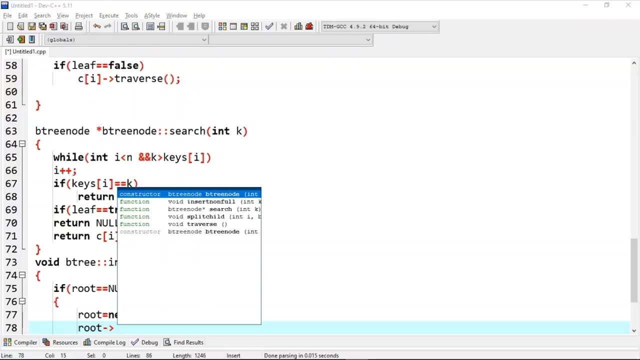 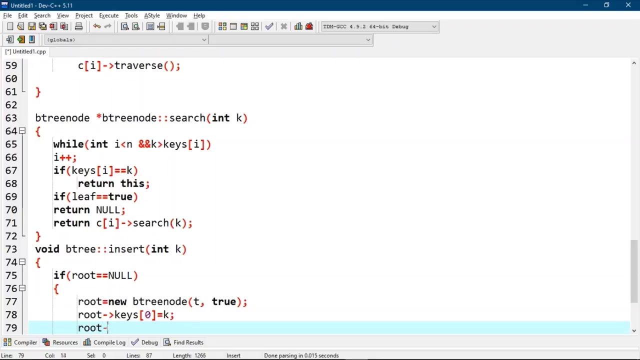 var. Stop Now. root keys. bracket zero is equals to k. Now we will change root Here. we are updating the number of keys in this root Now. if else else, if tree is not empty. 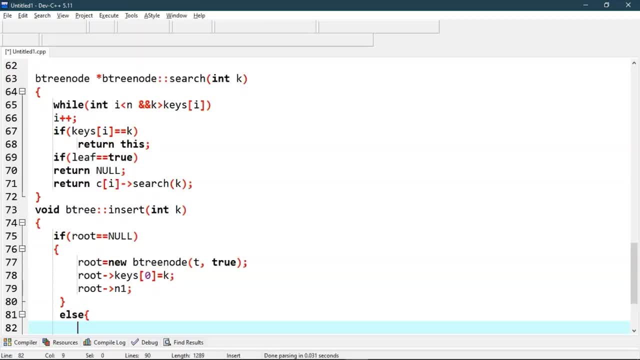 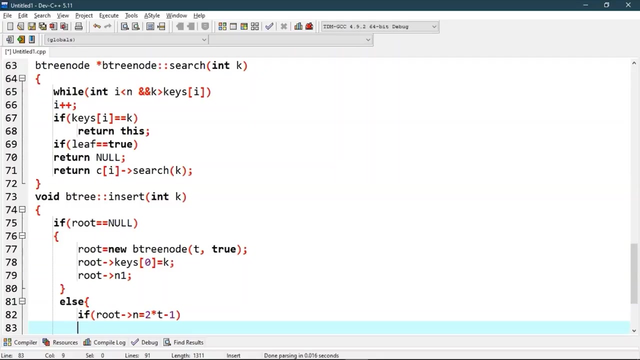 Ok, Then if root is full, then tree grows in height. So if root arrow n is equals to 2 star t minus 1. Then we will allocate The memory for the new root btree node star s equals to new btree node t, comma false. 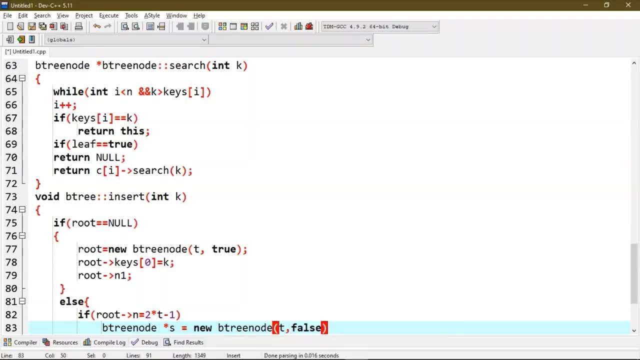 Ok, Now we will update the memory for the new root btree node star s equals to new btree node t comma false. Now, if else else, if tree is not empty, Then we will allocate The memory for the new root btree node star s equals to new btree node star s equals to: 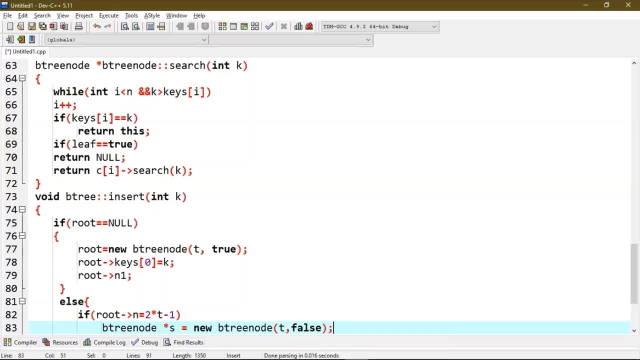 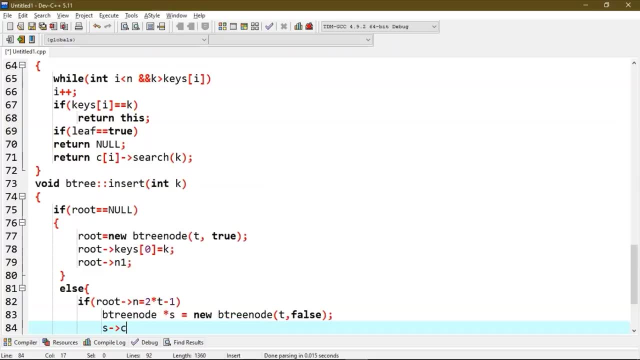 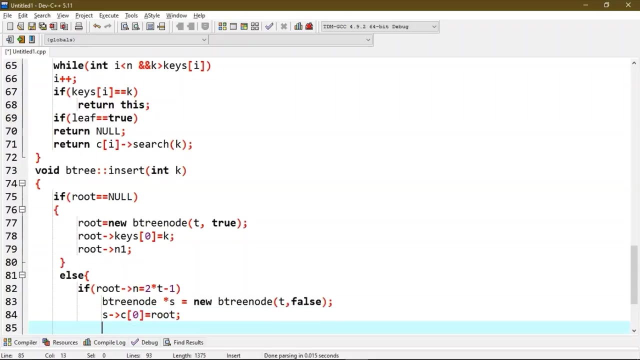 new btree node star s. Now we will make the old root as child of the new root, So s arrow c bracket zero is equals to root. Now we will split the old root and move one key to the new root. Ok, move one key to the new root So as split child. 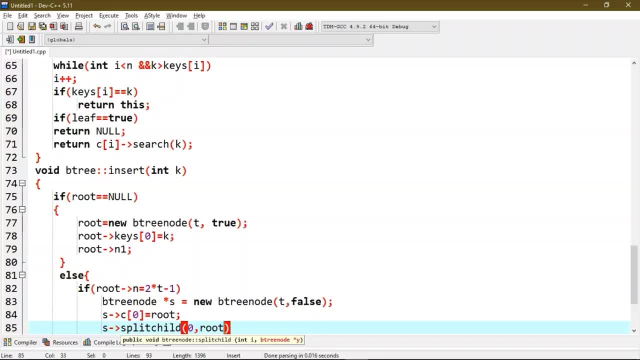 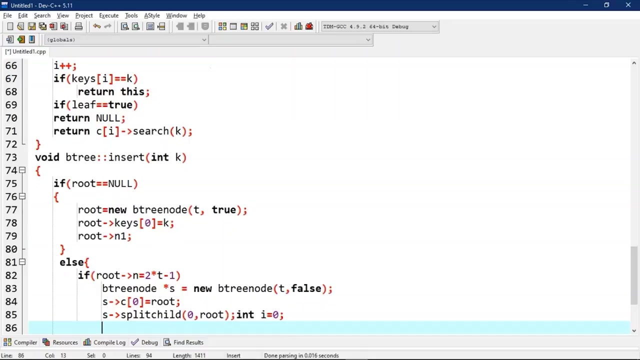 zero. comma root. Now new root, has two childrens. We have to decide which of the two children is going to have a new key. So int i is equals to zero. If So int i is equals to zero, So int i is equals to zero. 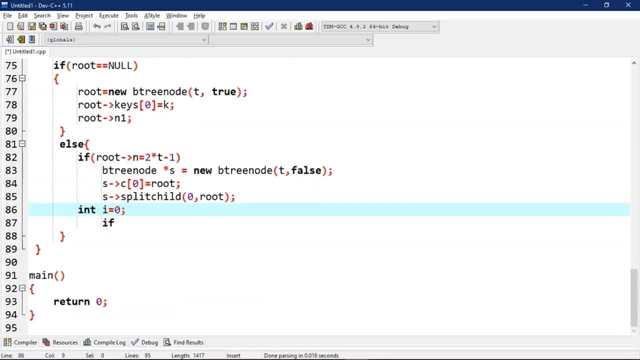 So int i is equals to zero. If, If, If as key is, as key is zero is less than is less than k is less than k, then i plus plus, then i plus plus, and as arrow c and as arrow c, bracket i, and as arrow c, bracket i: 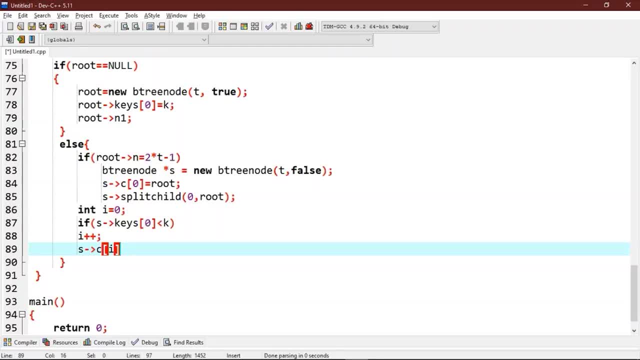 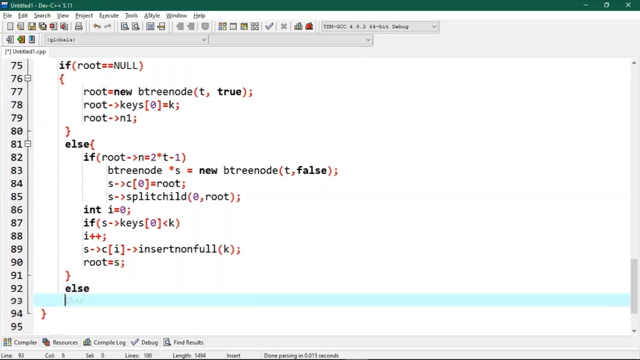 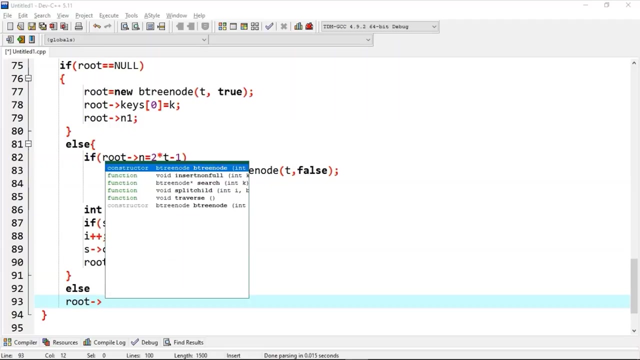 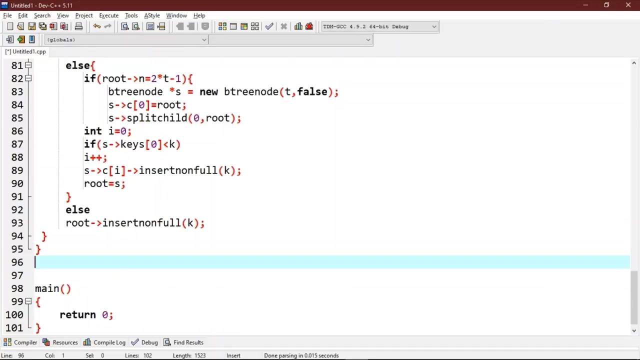 arrow. insert known full- k. now we will change the root equals to s. else. if root is not full, we will call the insert known full. now we will write a function insert for non-full. we will initialize int if is equals to n-1. if if is equals to true. 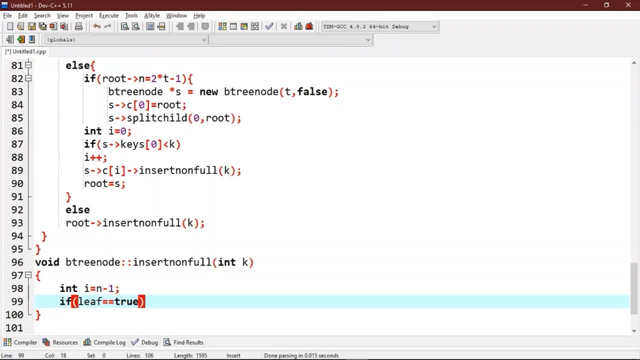 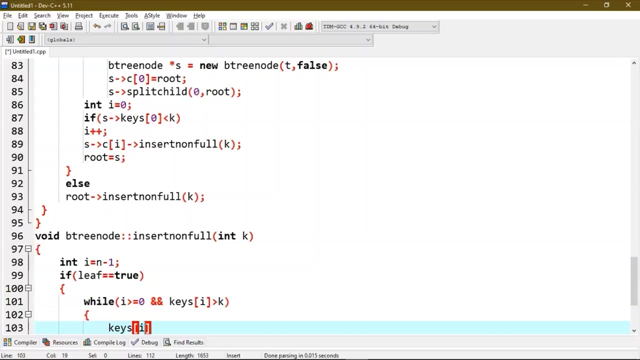 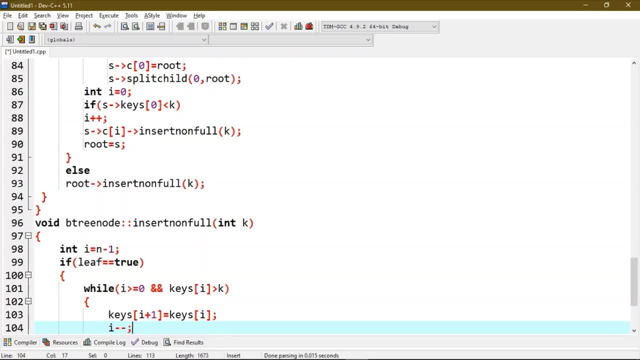 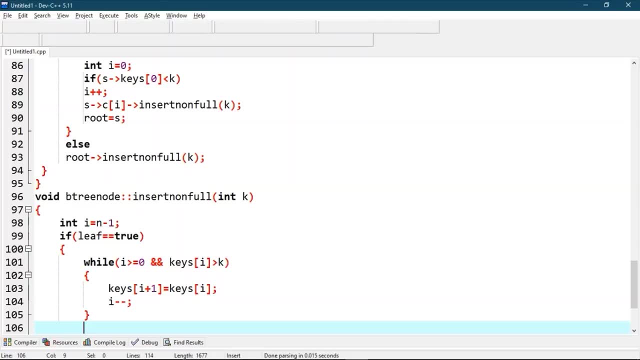 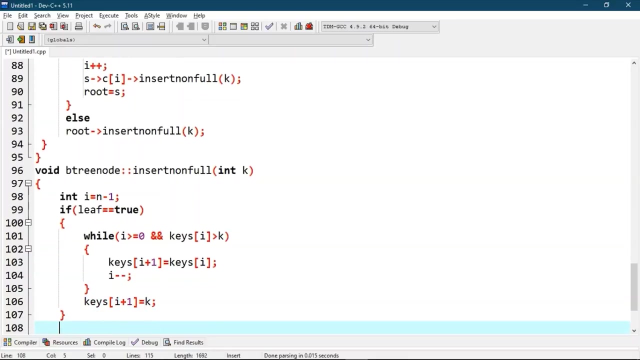 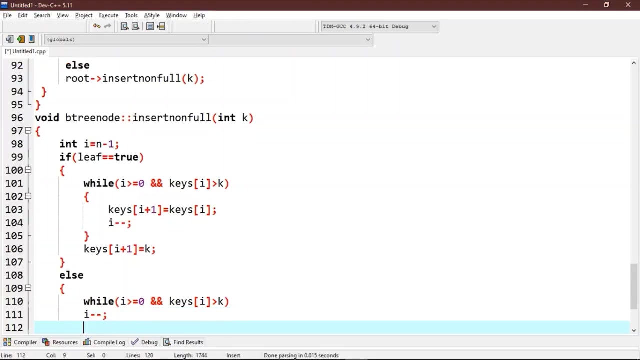 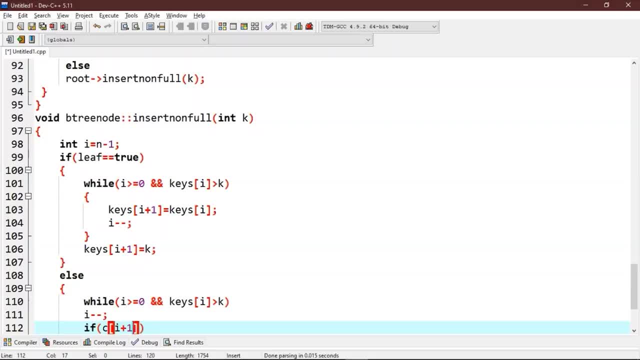 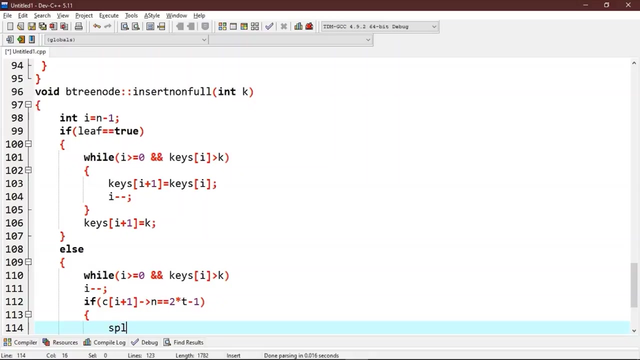 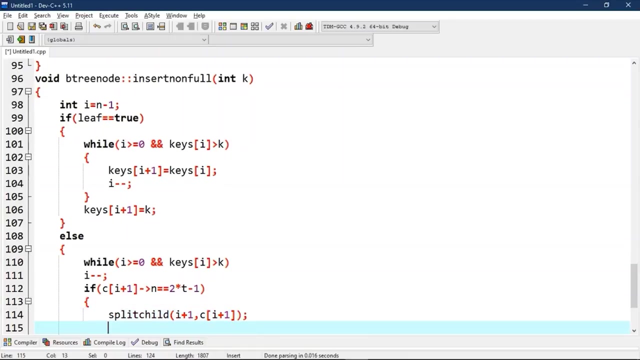 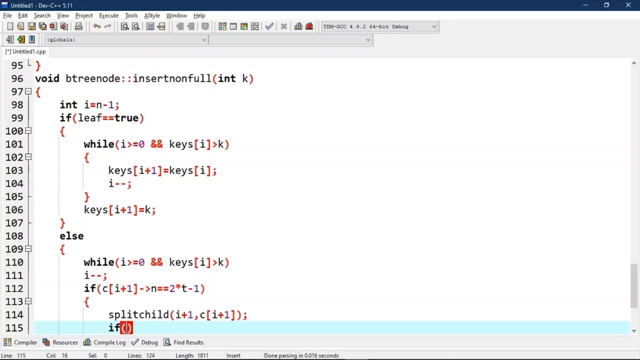 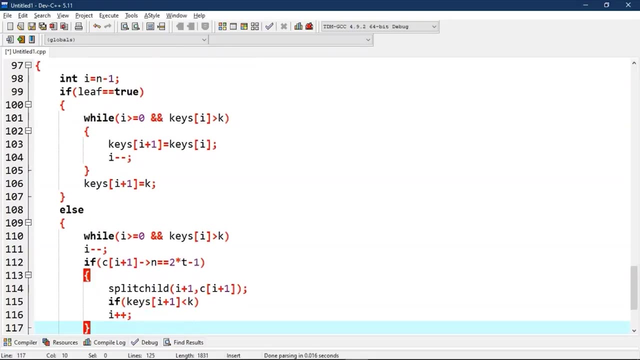 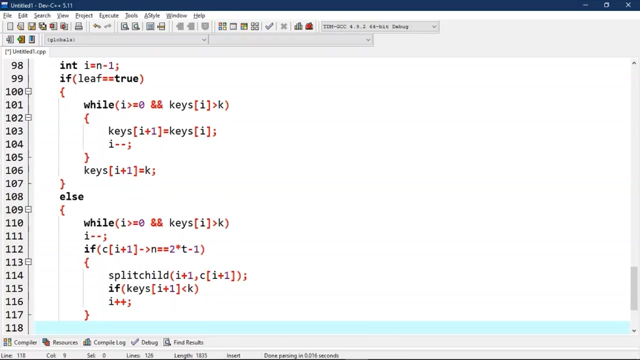 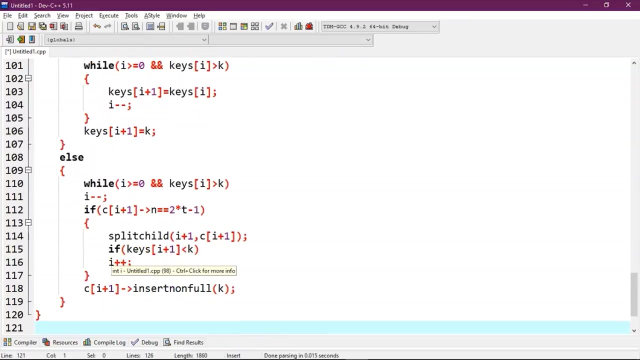 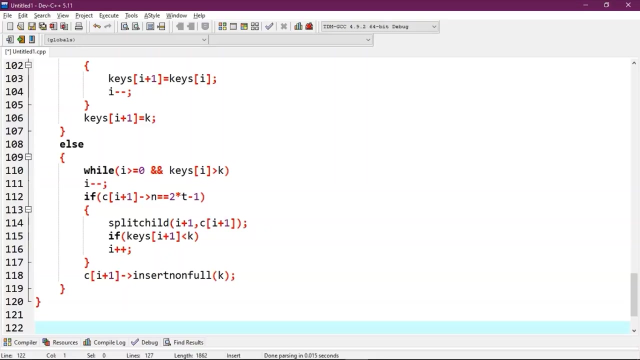 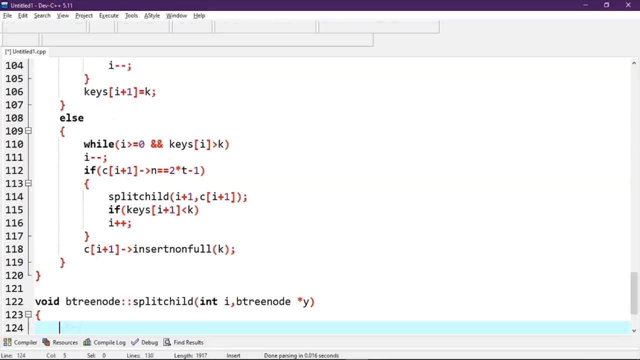 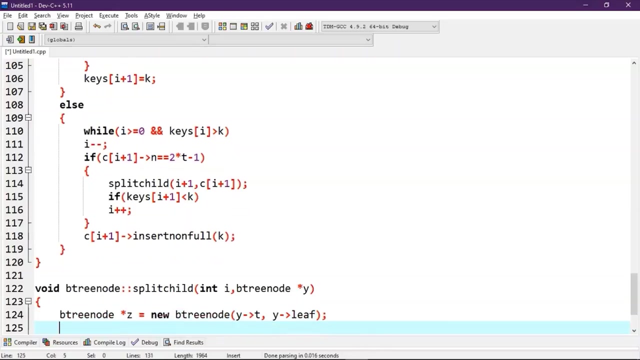 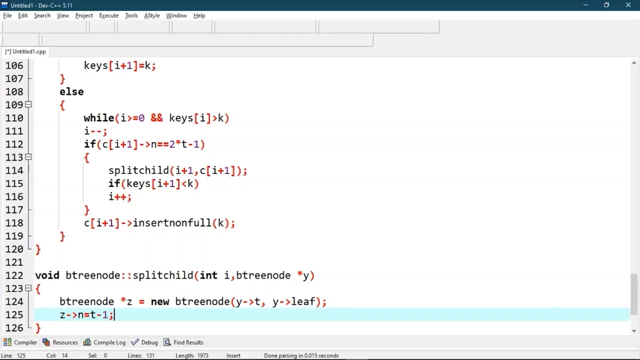 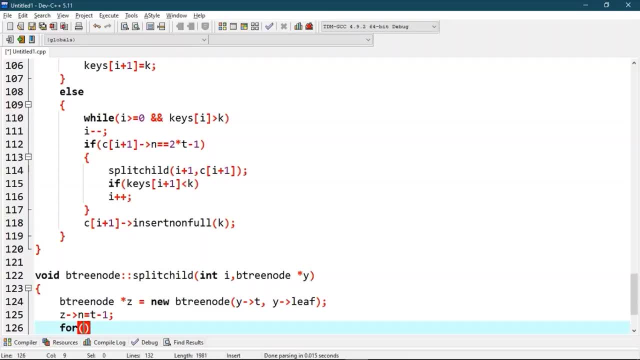 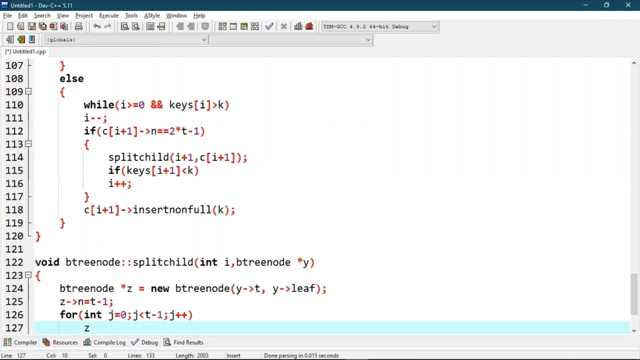 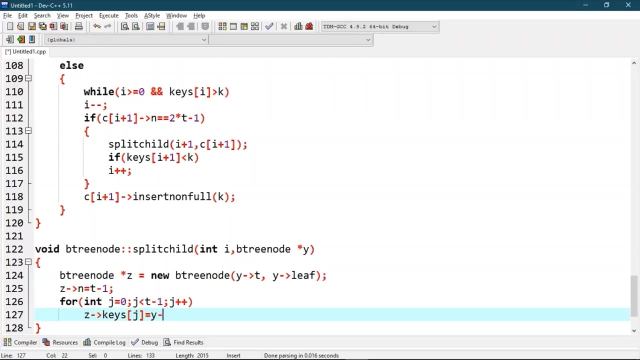 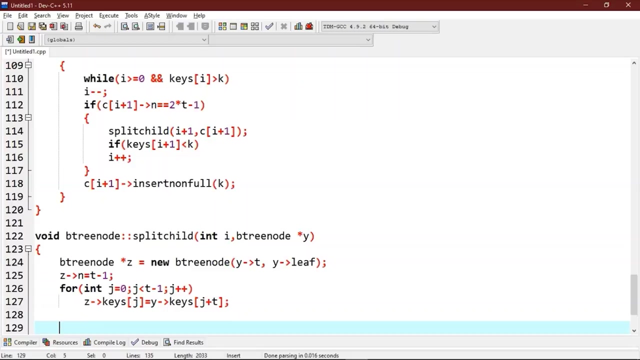 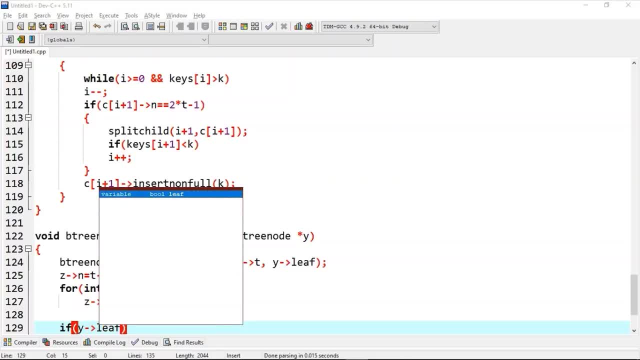 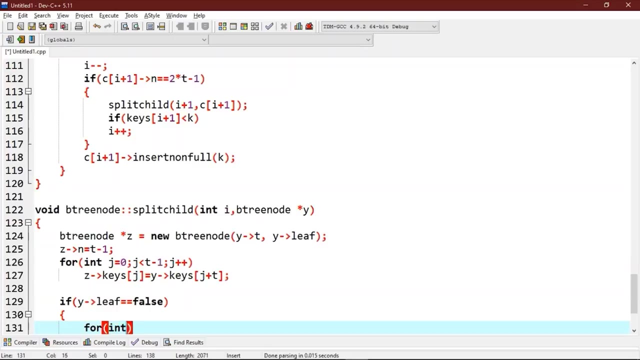 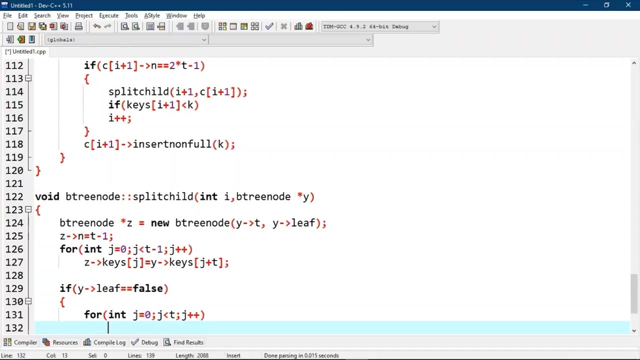 If yleaf is equals to false, then for int j is equals to zero, j less than t and j++. But if y i is equals to white, then for y we will hide. j is equal to n times x. Then put the t childrens in the cube: j equal to n times i. 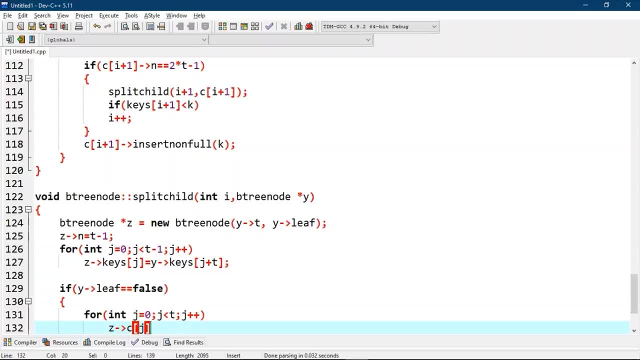 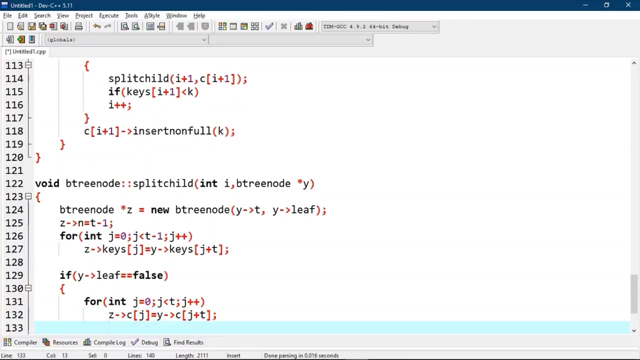 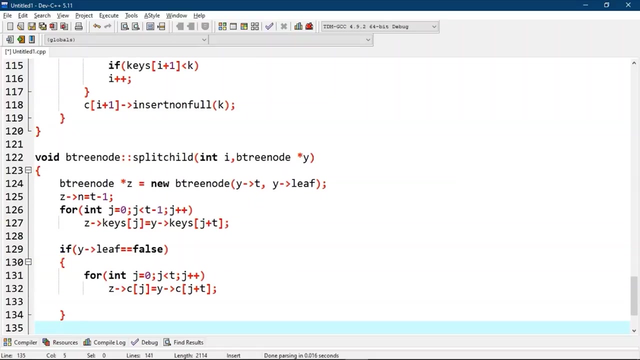 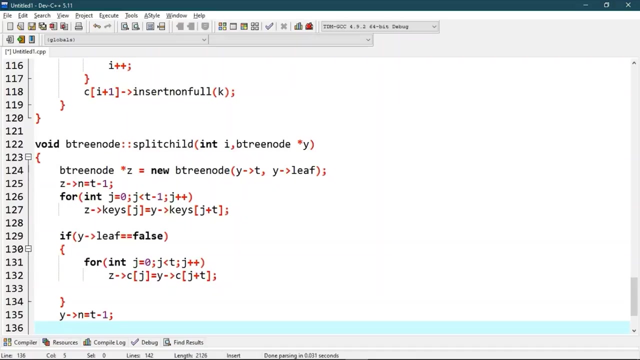 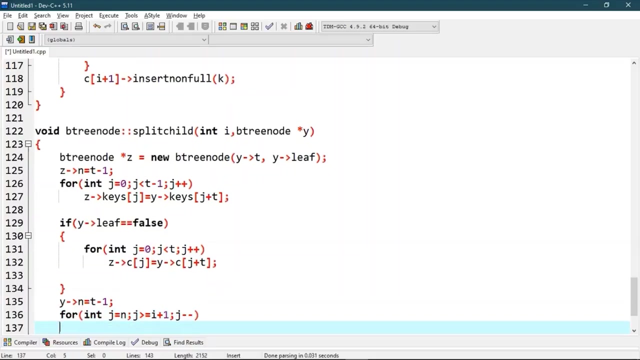 The Harsh Grandma will be reading the test- distances. 쌍 M. Now we will reduce the number of keys in Y. Since this node is going to have a new child, we will create a space for the new child. So for loop int j is equals to n, j greater than equals to i plus 1 j minus minus c bracket. 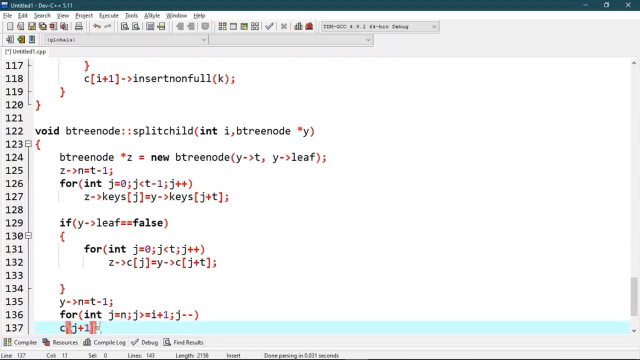 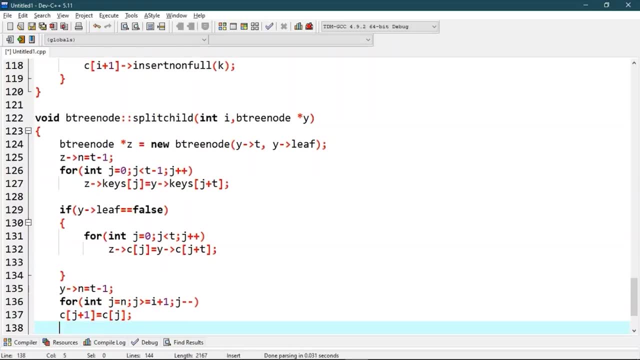 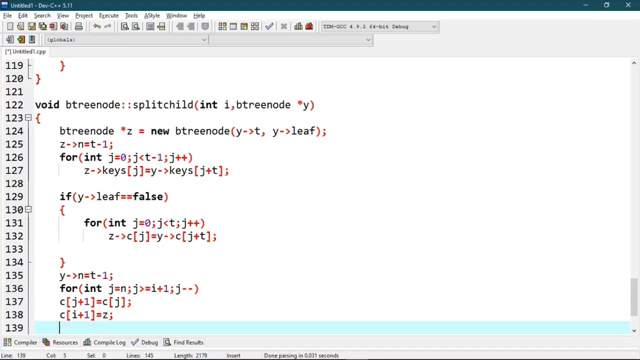 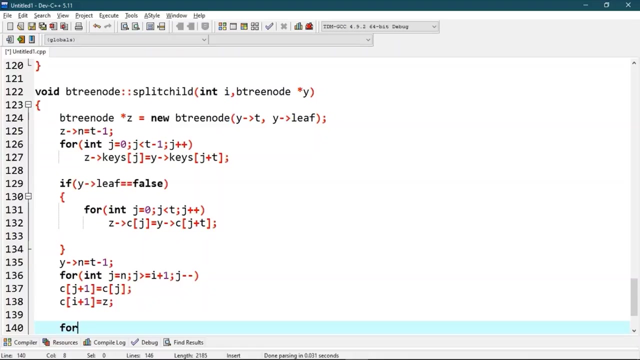 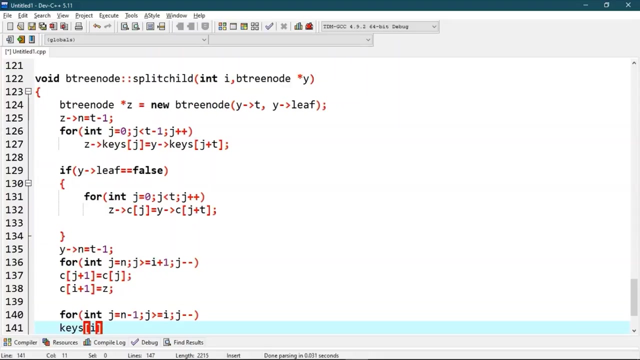 j plus 1 equals to c, bracket j. Now we will link the new child to this node. Now The new child of Y will move to this node and find the location of new key and move all greater keys one space ahead. If y of x equals to: 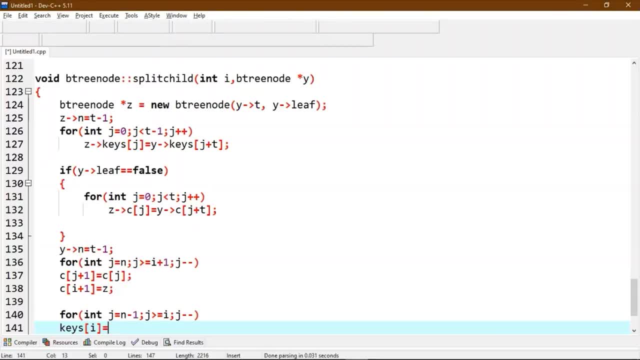 So protect the. Now you know the number of keys andough, you can use this and only give zero number of keys, And you can now be suitable for counting the multiple keys, Since how to connect all the keys in Y am 1 minus 2 various keys. 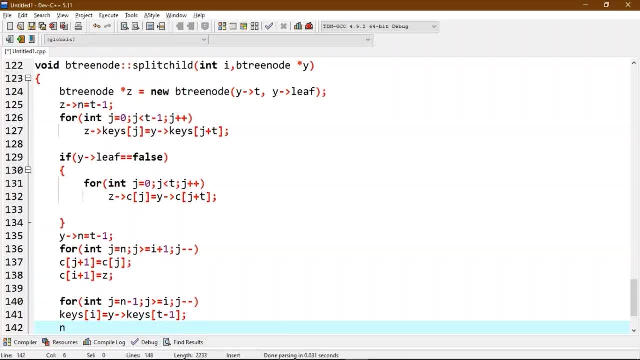 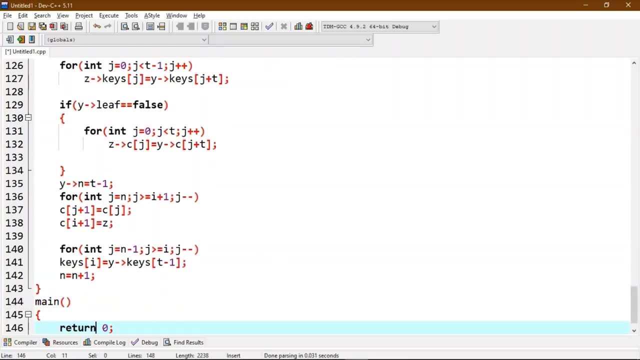 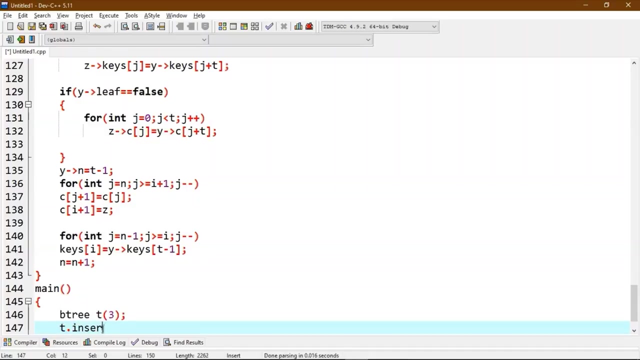 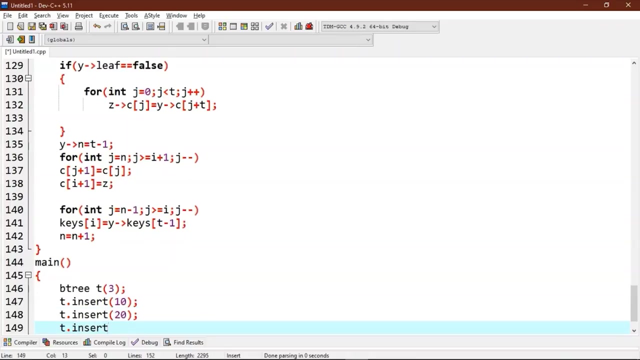 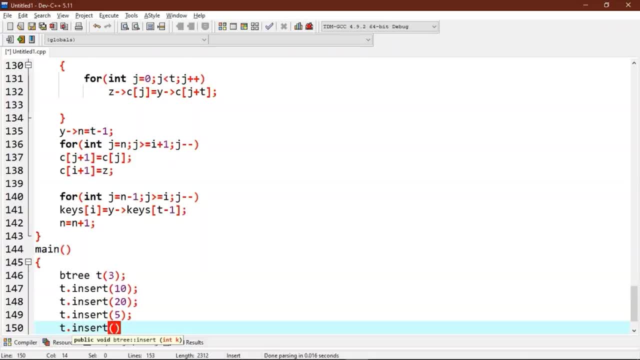 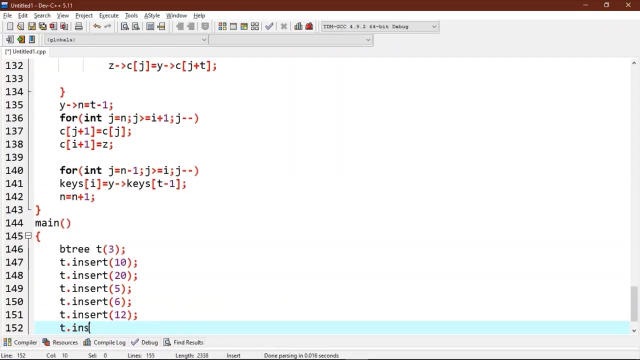 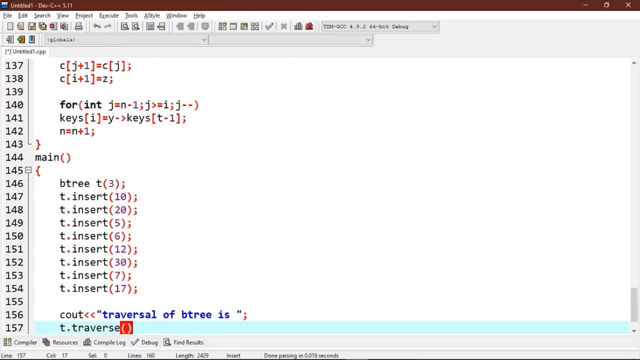 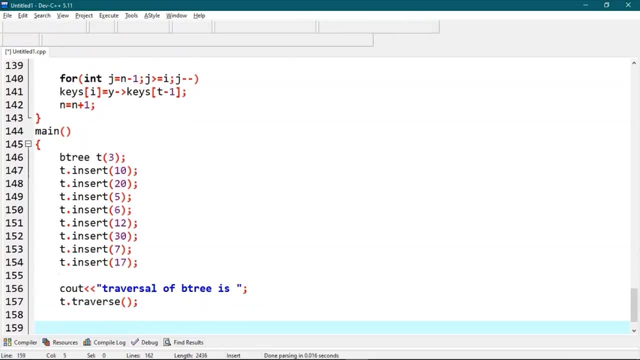 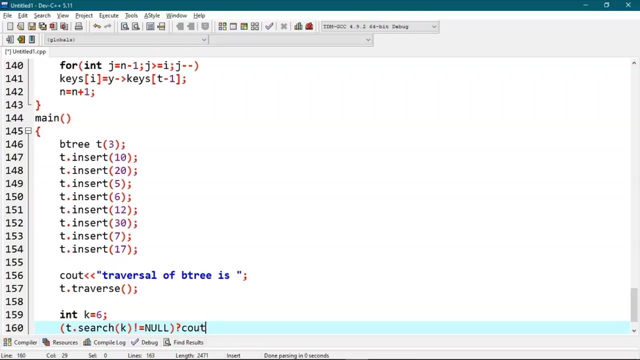 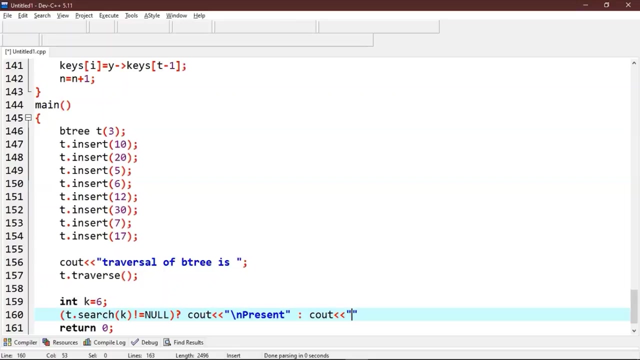 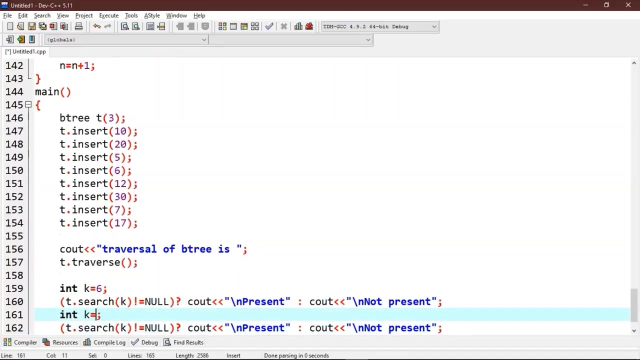 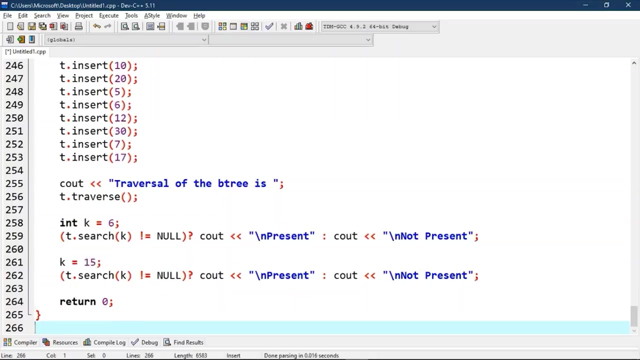 tinsert, tinsert, tinsert, tinsert, tinsert. Now let's search some keys. So let's state: int k is equals to 6.. So if tsearch k is not null, then cout, else cout. let's try this function one more time with k is equals to 15, let's execute this: 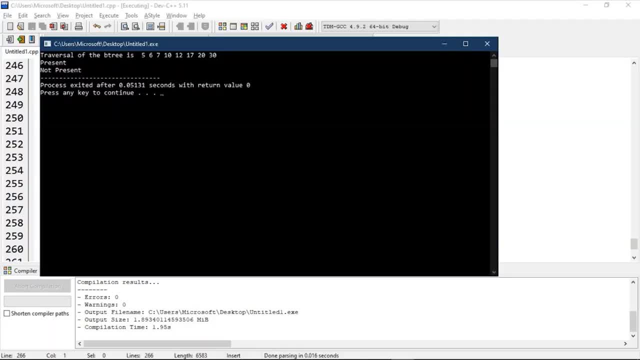 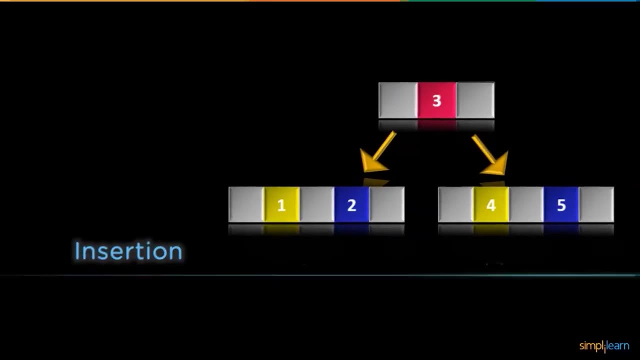 as you can see, we have successfully traversed this b-tree and we have checked two keys if they are present or not. the k is equals to 15 was not present and k is equals to 6 was present. let's get back to our slides. next up, insertion. we have to insert an element in such a way so that we won't disobey any. 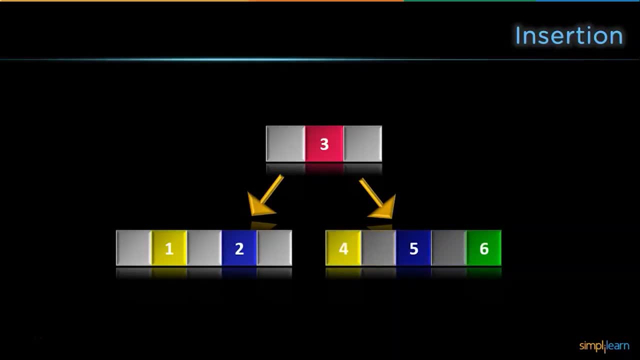 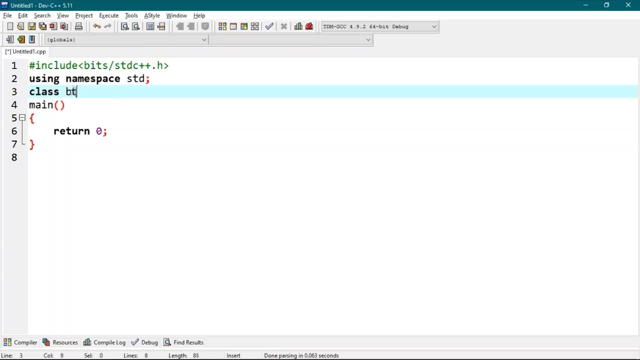 properties of b-trees. now let's try this operation in a code editor. we will start by creating a node. to do that, we will use class b-tree node. then we will create an array of keys, minimum degree, an array of child pointers. show subtle hash czasu. 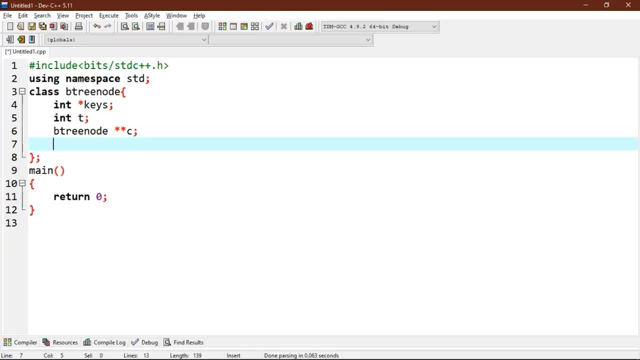 selected tag dis weekly, weekly next. expect Current number of keys and a boolean variable- leaf. This variable will tell if the node is leaf or not. Then we will define some public functions. We will start with constructor. Now we will create a function to insert a new key into the non-full node. 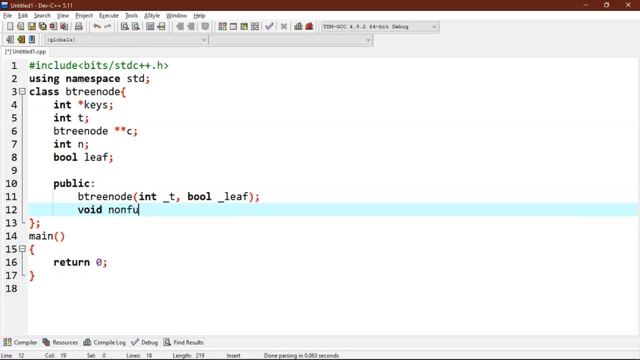 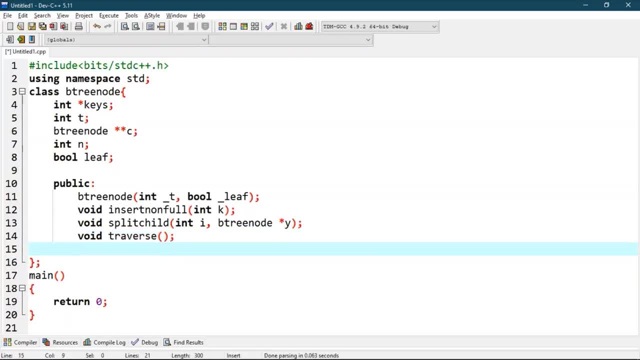 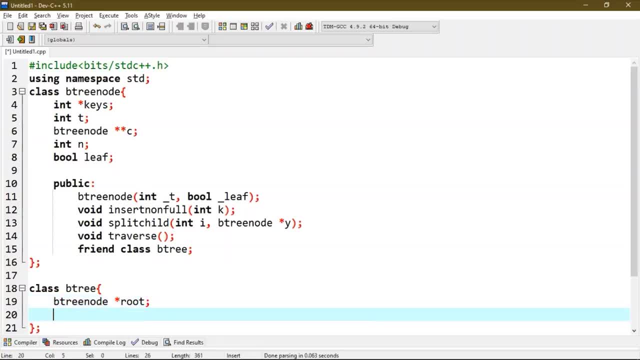 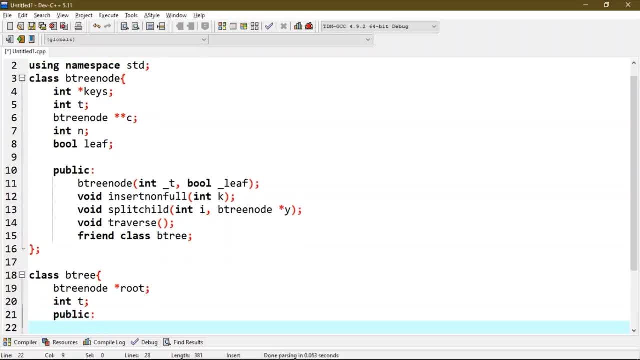 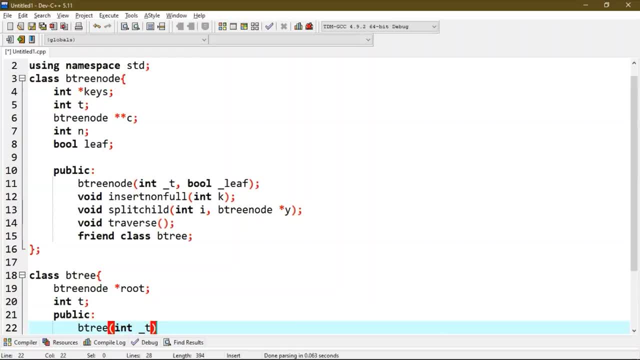 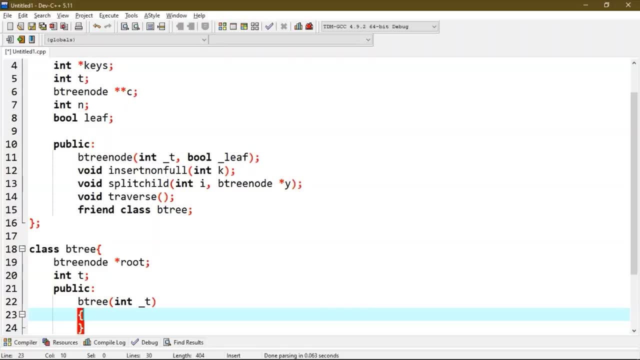 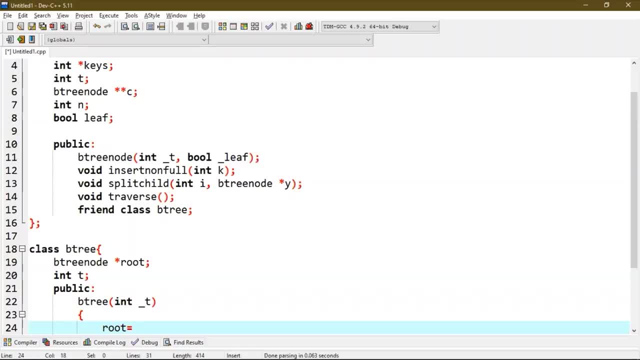 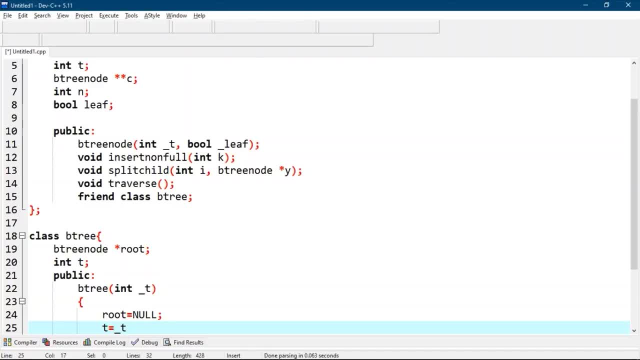 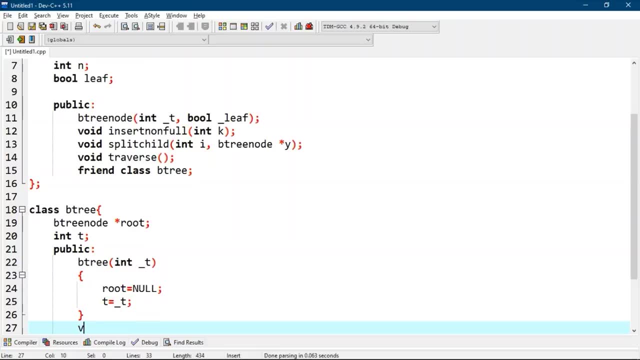 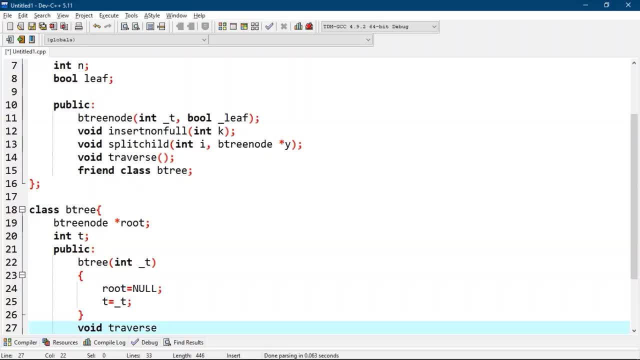 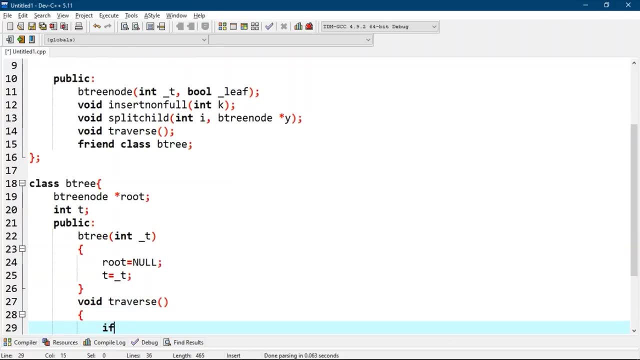 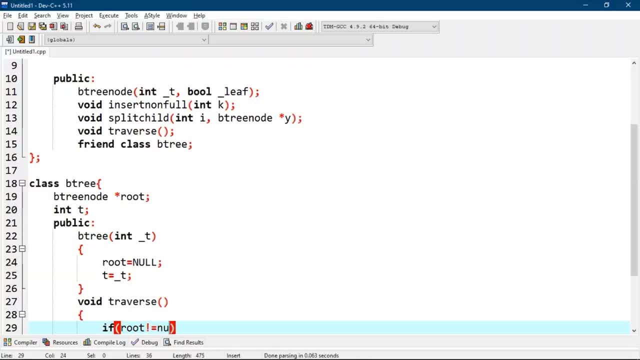 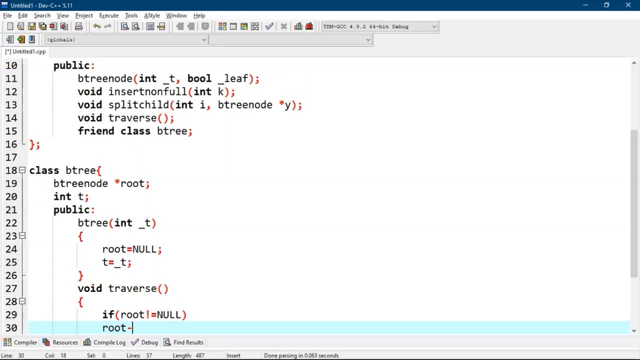 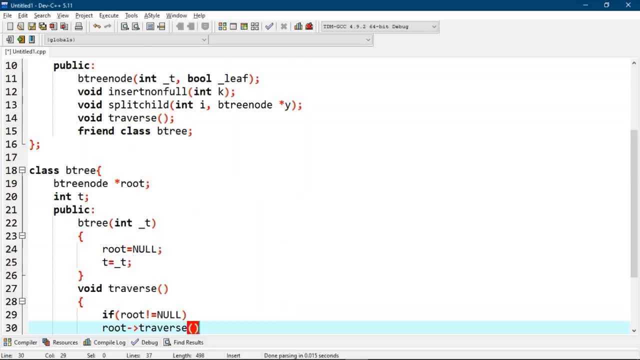 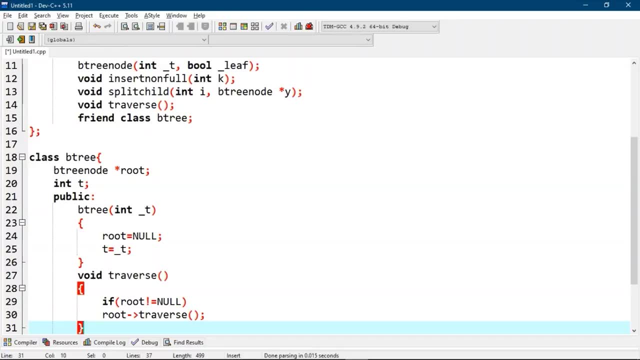 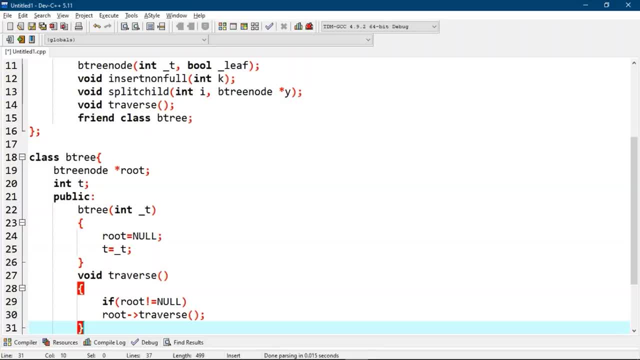 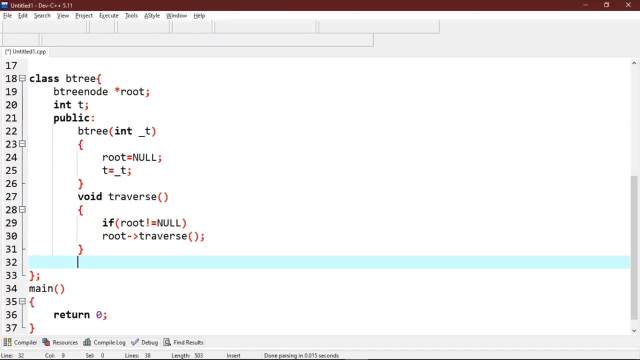 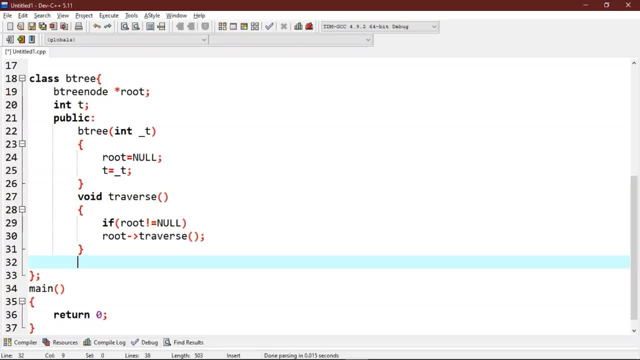 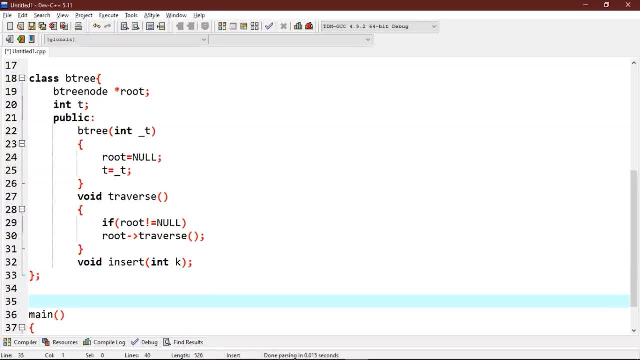 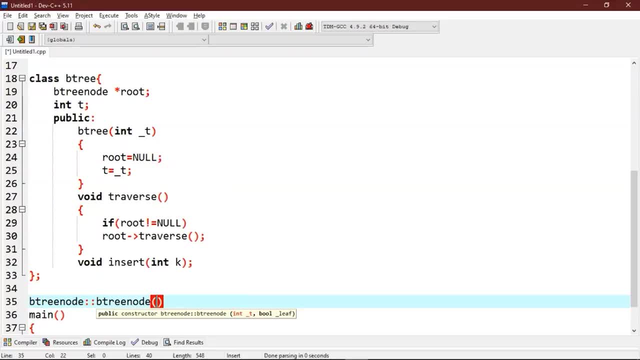 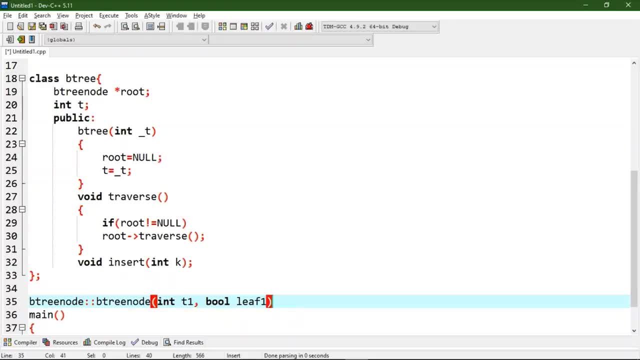 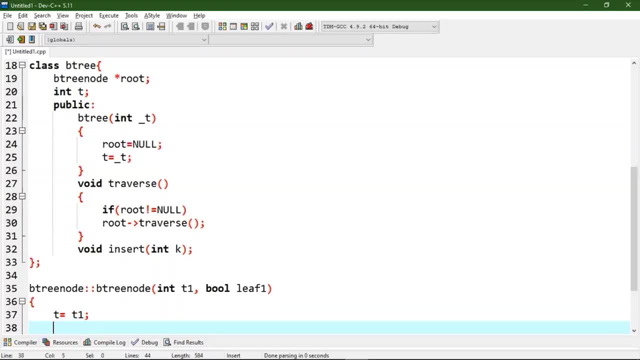 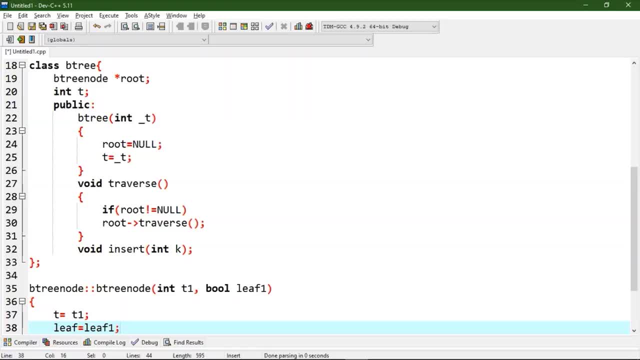 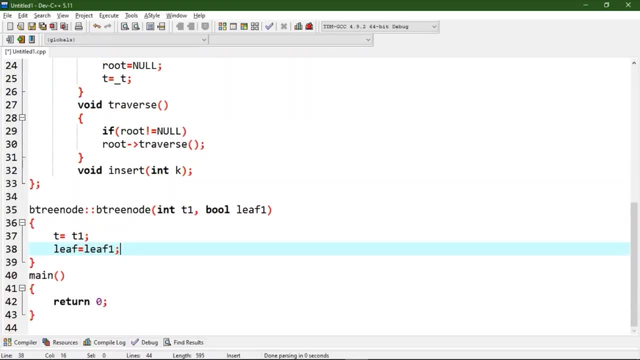 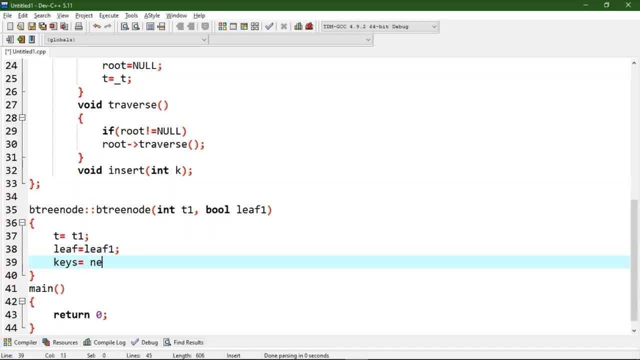 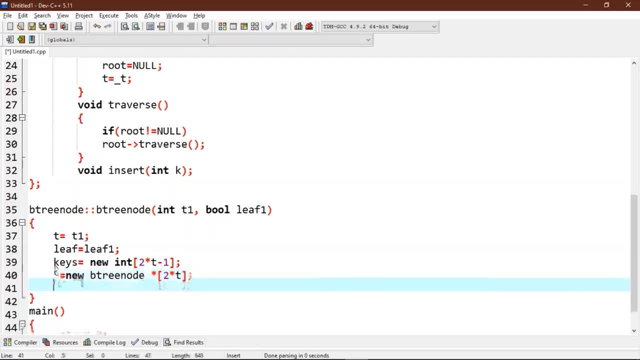 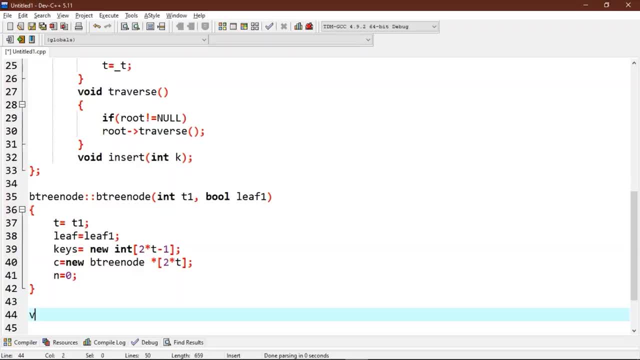 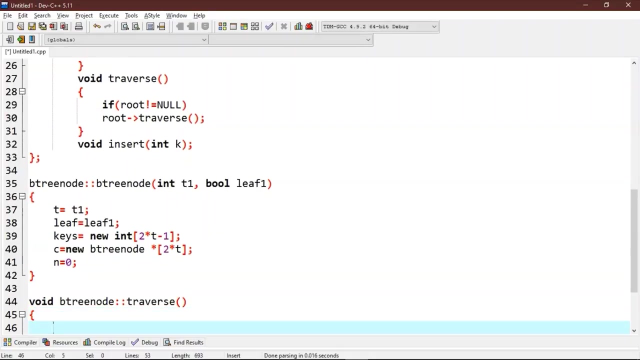 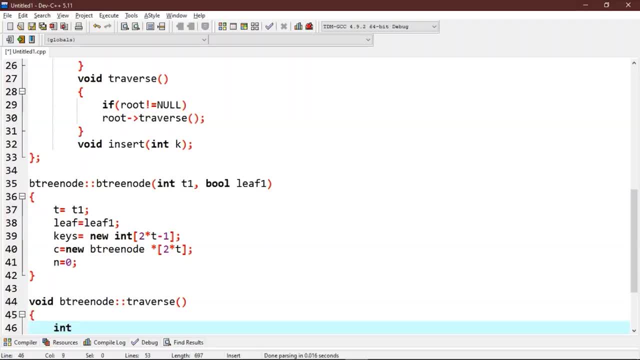 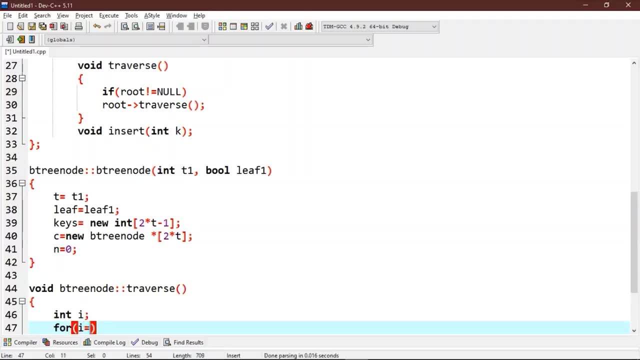 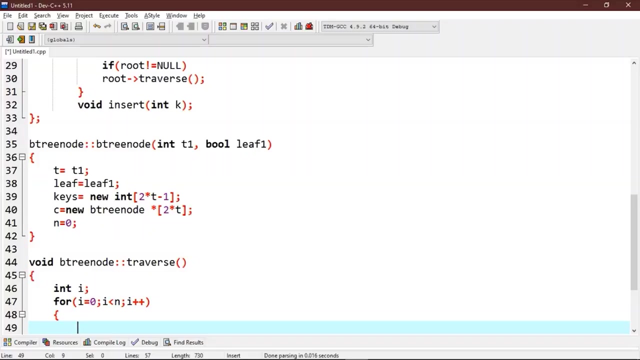 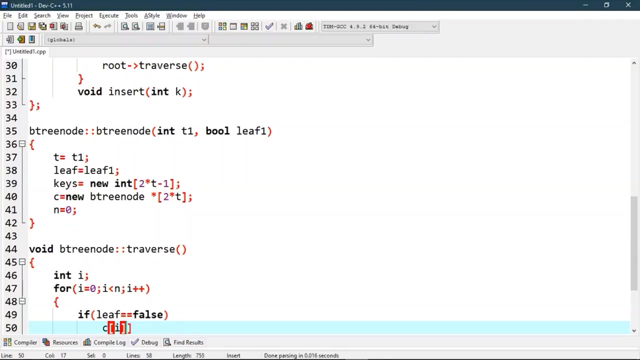 n children. So int i for loop, i is equal to 0, i less than n and i plus plus. Now suppose if this is not linked, Then before printing key we will traverse the subtree rooted with this child. So if if is equals to false, then ci arrow traverse. 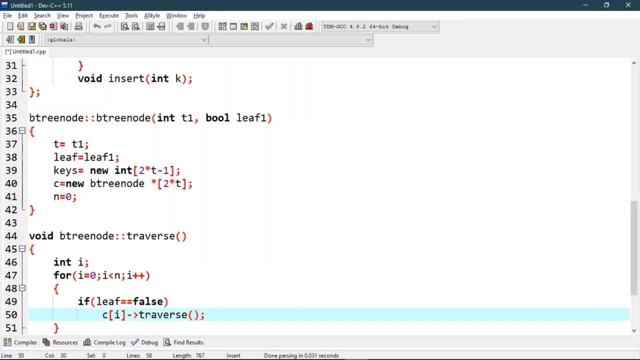 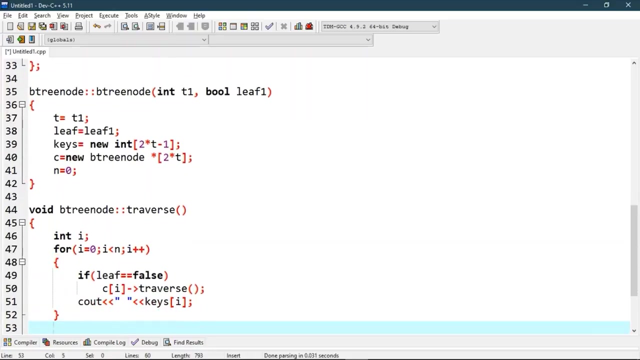 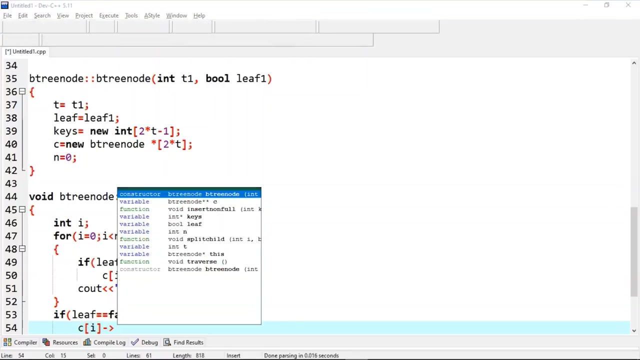 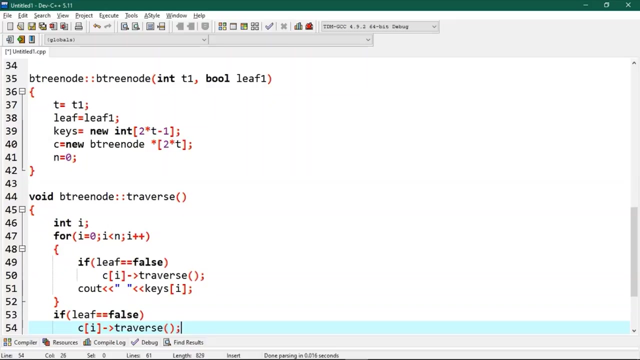 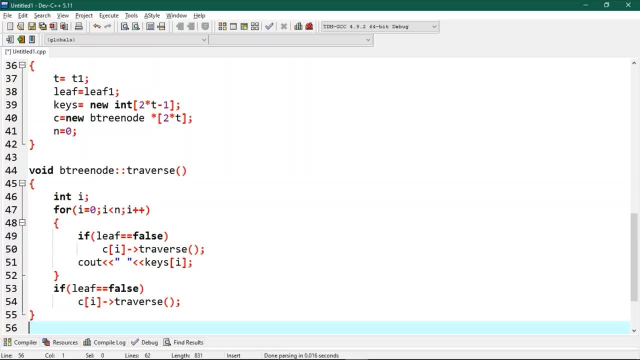 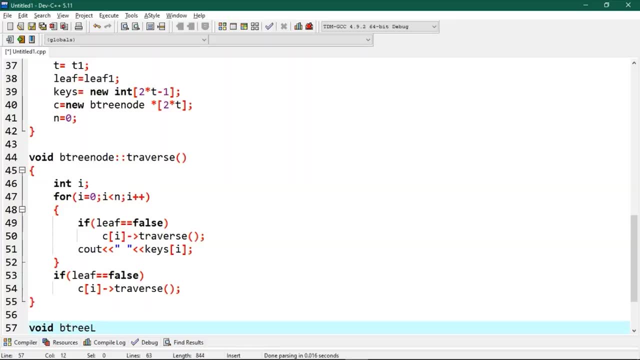 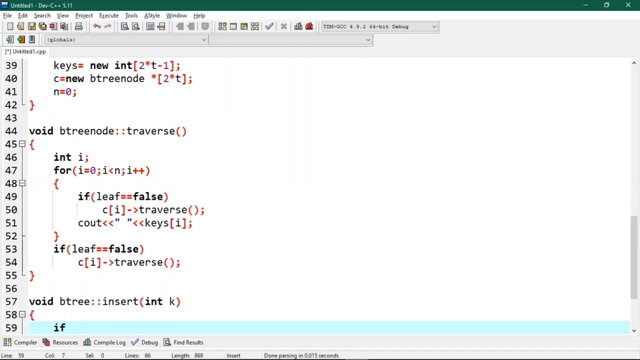 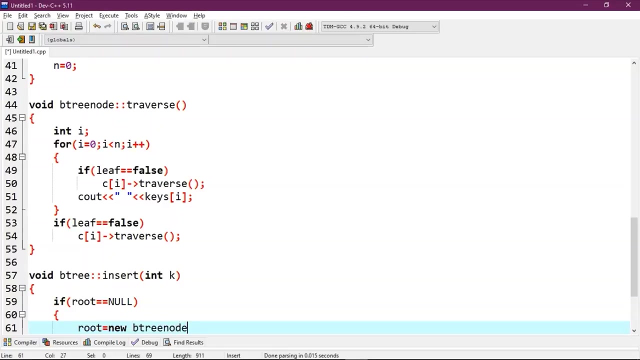 Now we will write the main function. Now we will enter domain that inserts a new key in this btree: void btree. insert int k Now. if tree is empty Now, Then we will allocate the memory to root. so root is equals to new btrayNode. 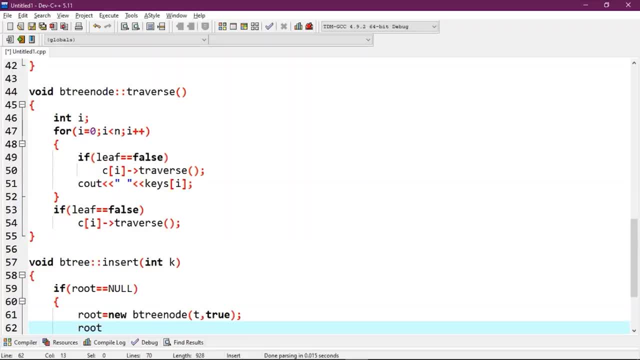 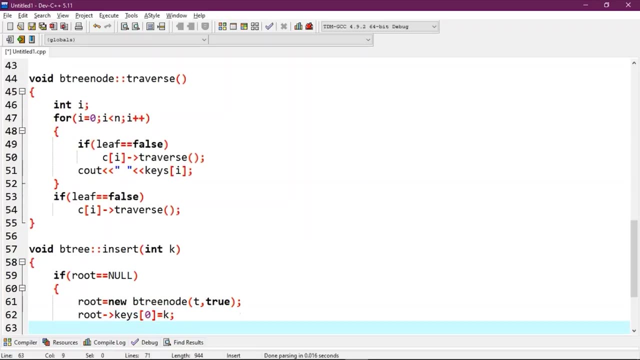 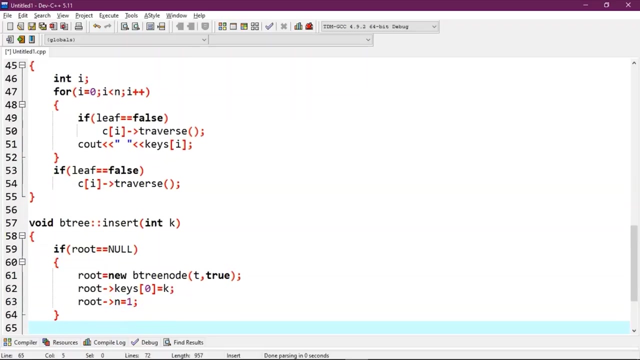 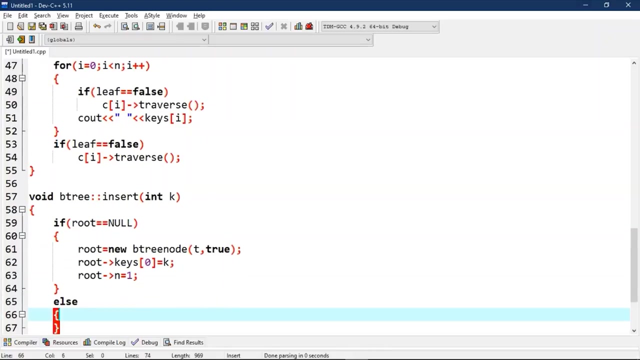 Now we will insert the key, so root arrow keys equals to k and we will update the number of keys in root, so root arrow n equals to 1.. Else, if tree is not empty and if root is full, then tree will grow in height. if root 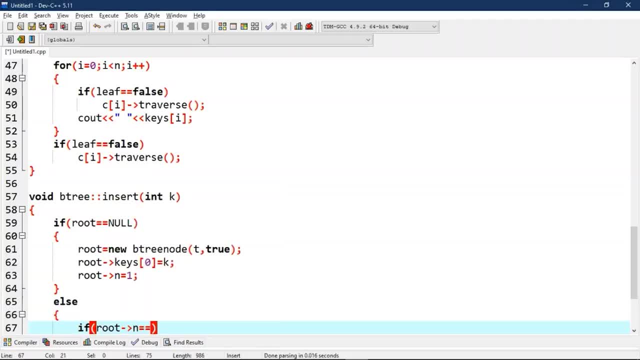 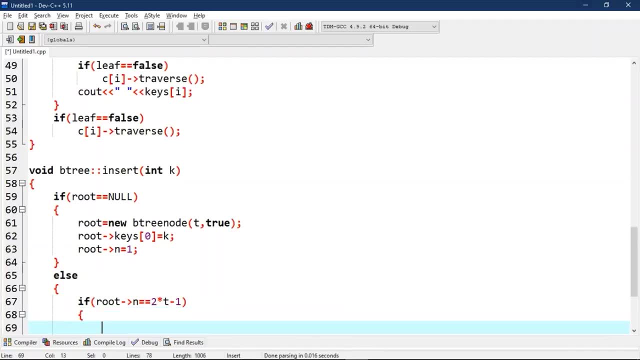 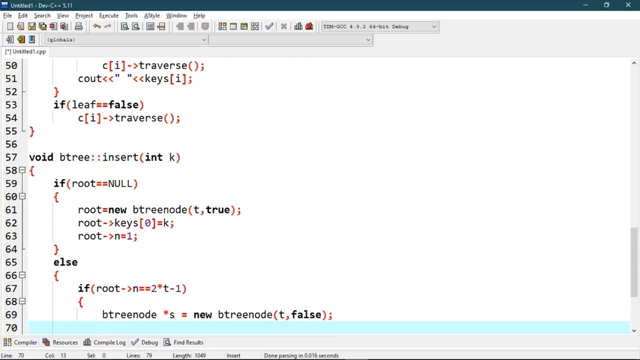 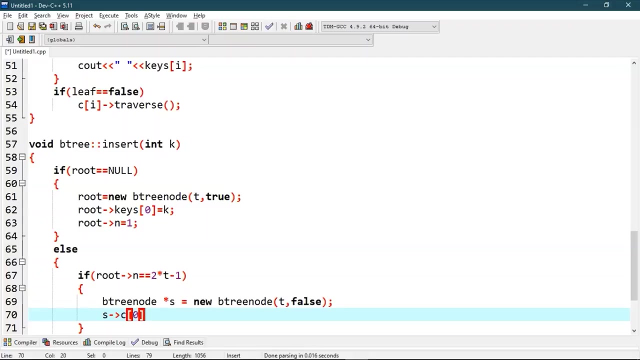 arrow n is equals to 2 star t minus 1.. Now we will allocate the memory of new root. Now we will make old root as child of new root. Now we will make old root as child of new root. Now we will split the old root and move one key to the new root. 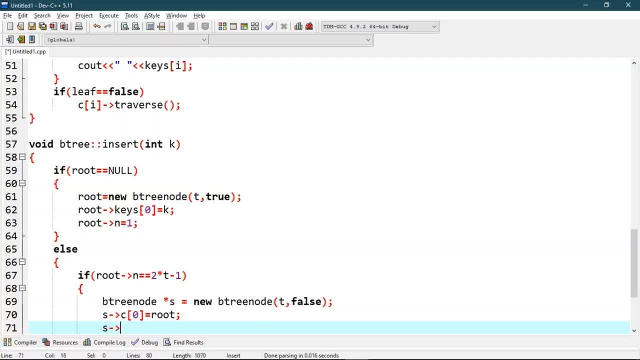 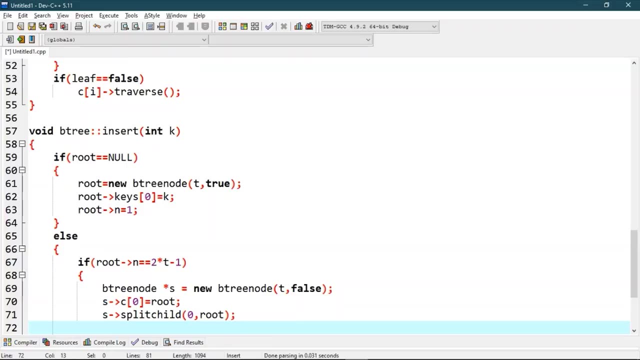 So we can see karIf button is empty, The old root isn't also empty. So to do that, we will use splitChild function. Now new root has 2 childrens. now We have to decide which of the 2 childrens is going to have new key. so to do that, we 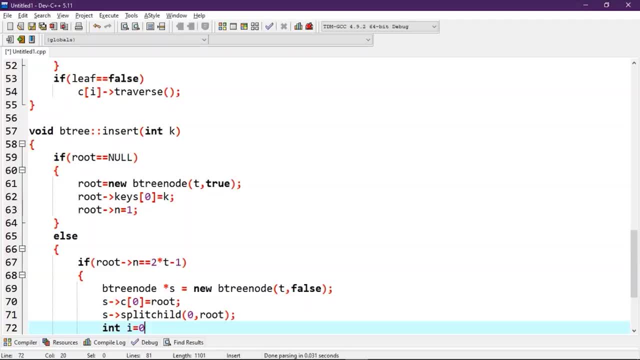 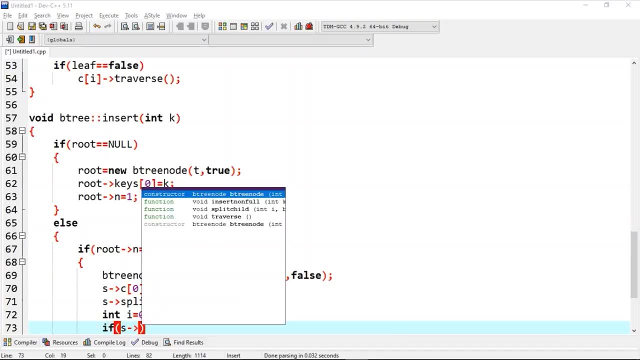 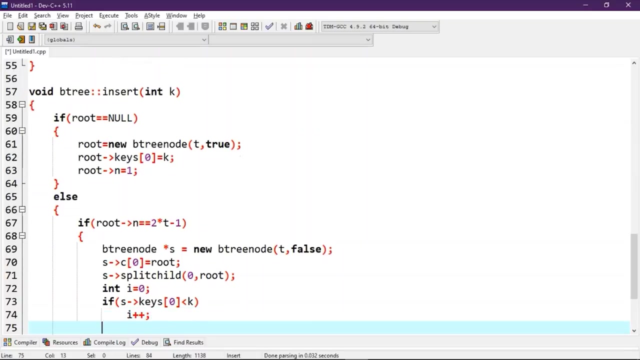 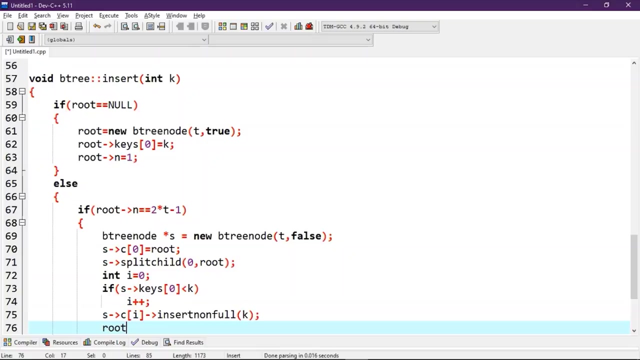 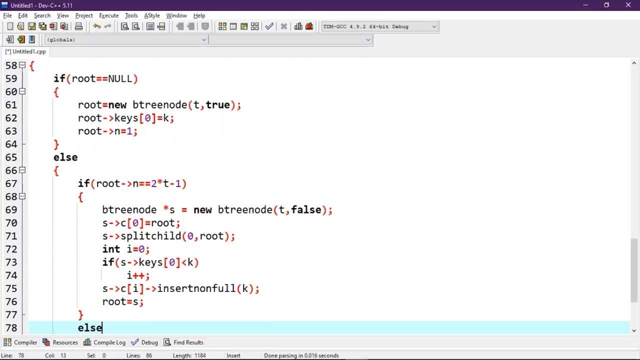 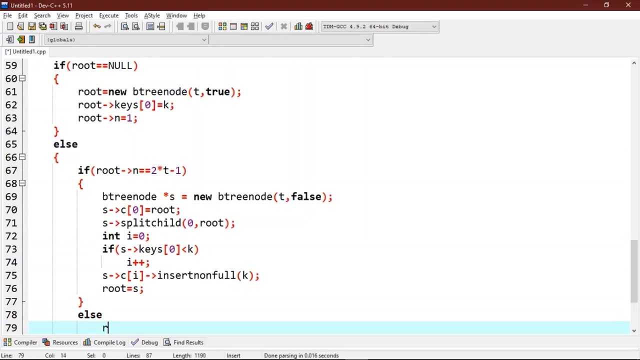 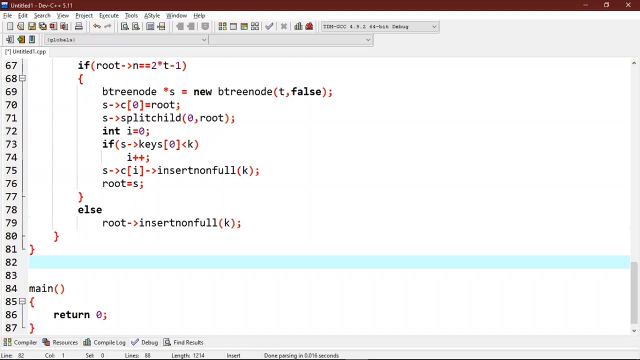 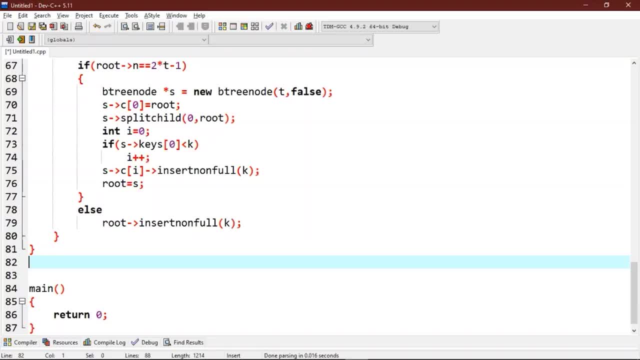 We will assume the node must be non-full when this function is called. So: void btreeNode. insert non-full int k. We will initialize index as index of rightmost element, So int i is equals to n-1.. Now if this is a leaf node, then the following loop does two things: a- finds a location of. 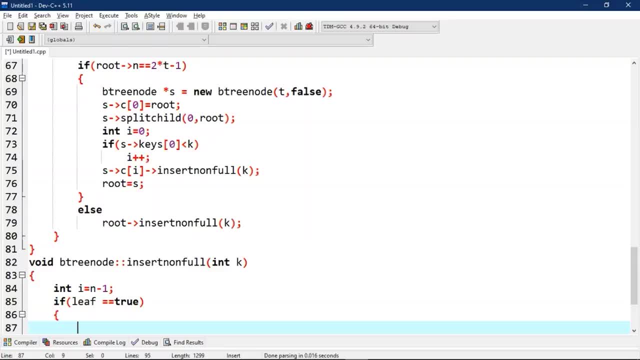 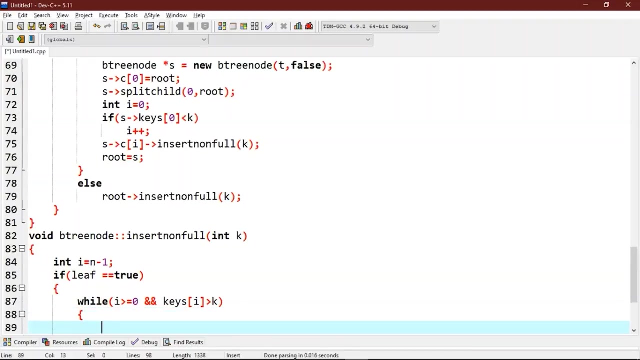 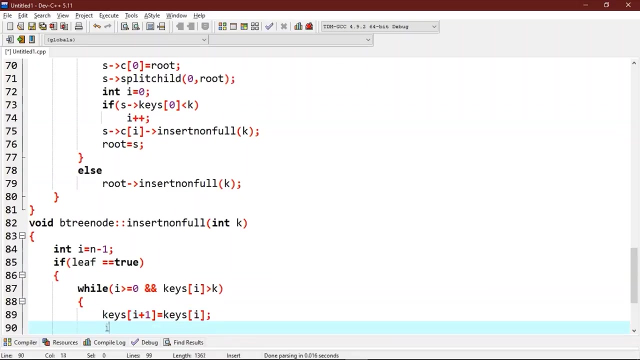 new key to be inserted or move all greater keys to one place ahead. So, while i is greater than equals to 0. And keys i is greater than k, Now keys i plus 1 will be equals to keys at i And i minus minus. 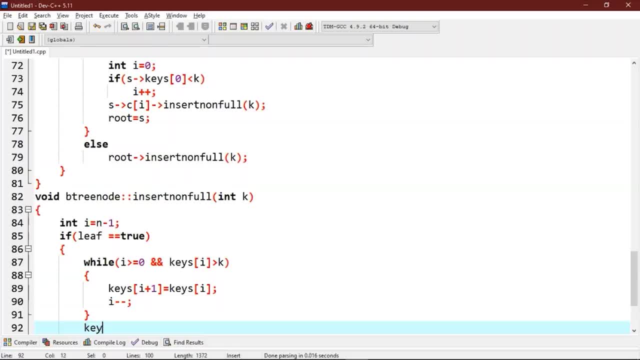 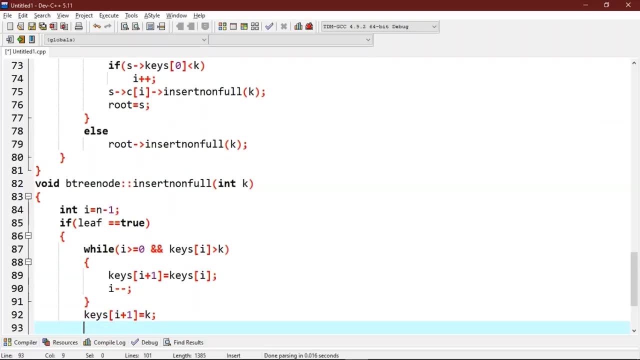 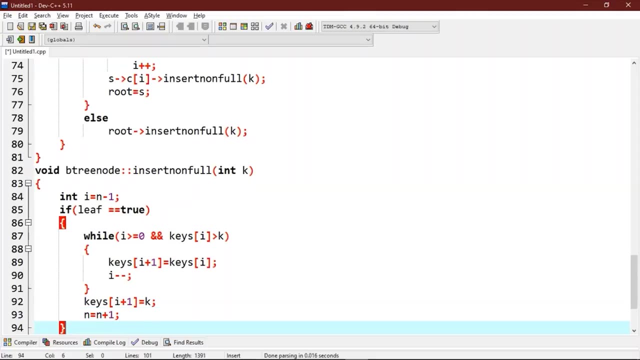 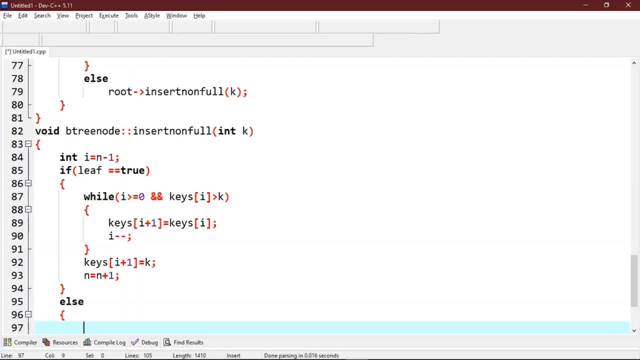 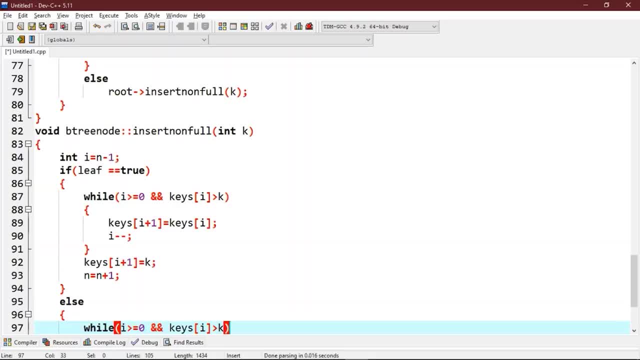 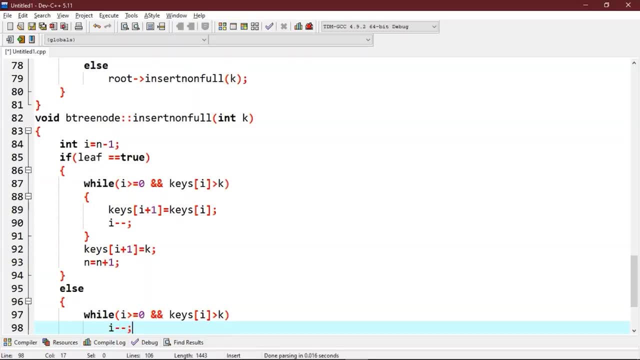 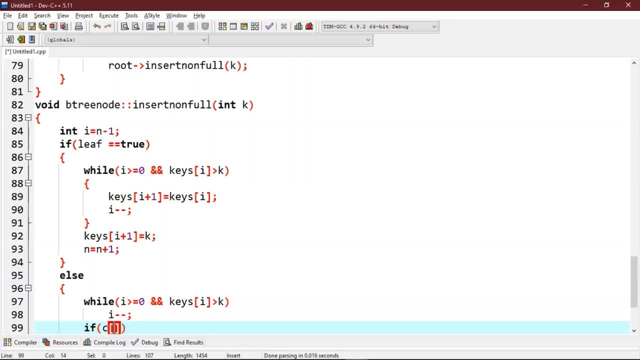 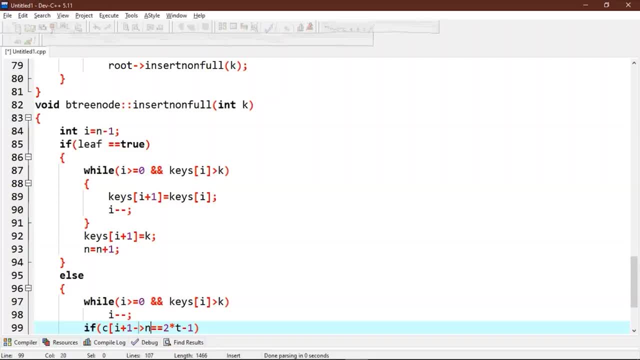 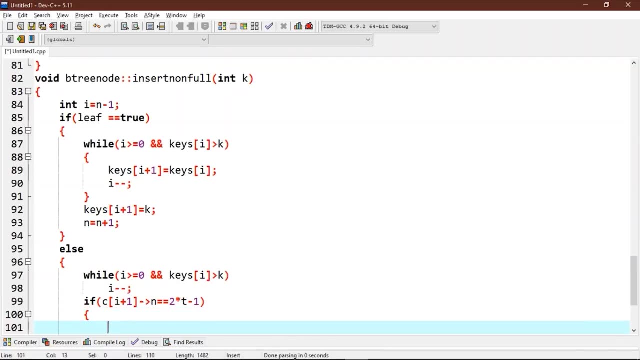 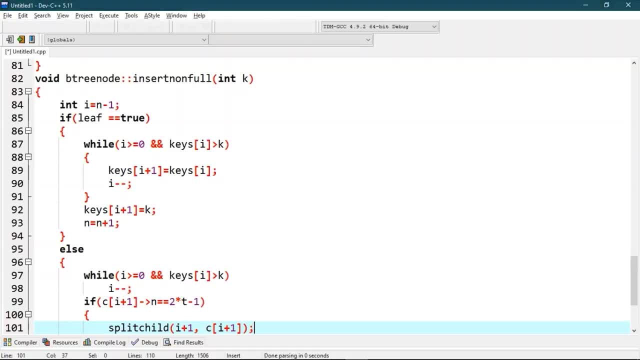 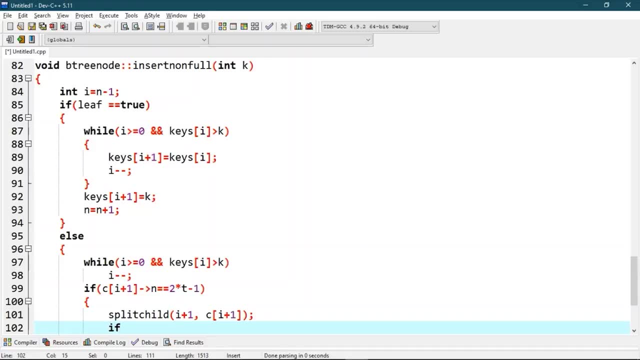 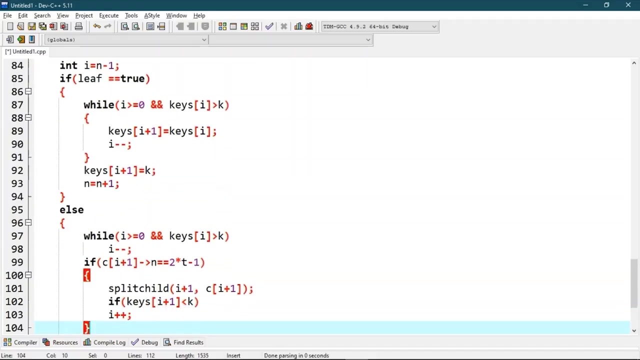 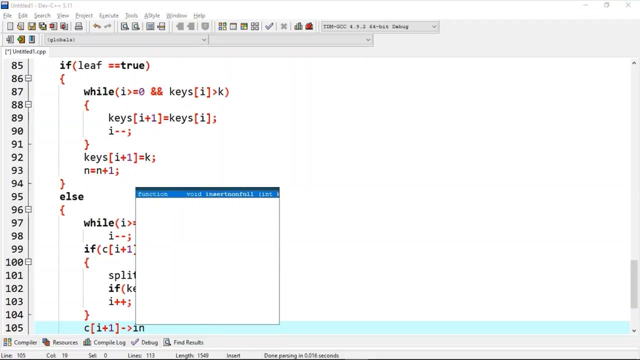 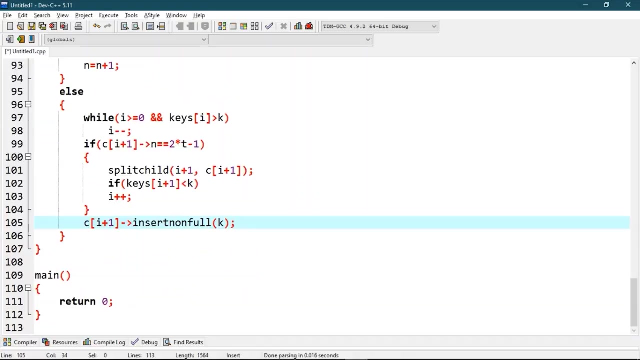 Now we will see which of the following will have the new key: f keys: i plus 1 is less than k. then i plus plus c, i plus 1. insert non-full k. i plus 1, i plus 1, another child and I comma: a tree. 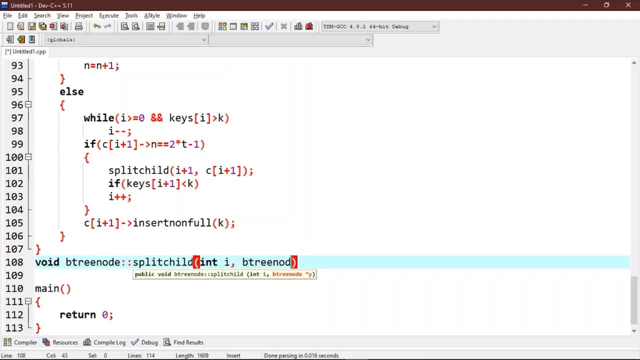 non-full, i plus 1 node. now we will create a new node which is going to store t-keys of y. So btree node star z equals to new btree node y arrow, t comma, t-key. So we will create a new node which is going to store t-keys of y. 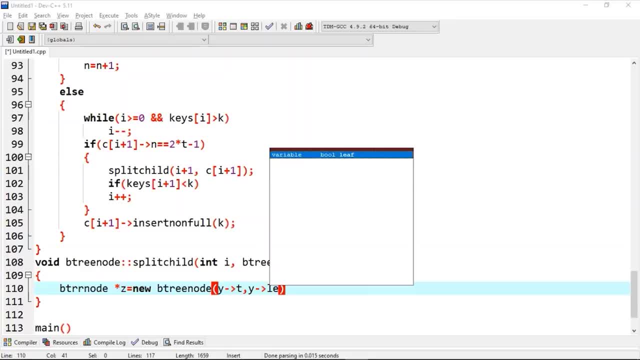 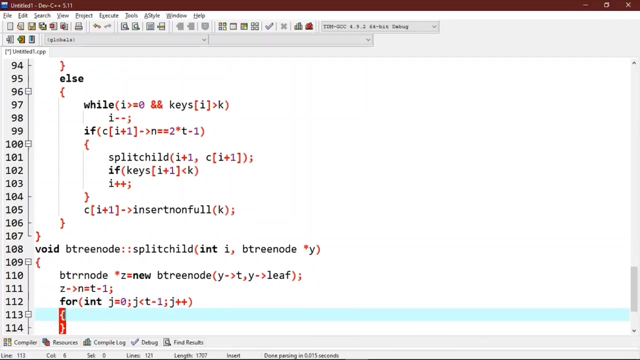 y arrow leaf, Now z arrow n is equals to t-1.. Now we will copy the last t-1 keys of y to z. So for loop int j is equals to 0,, j less than t-1,, j++. So z arrow keys j. 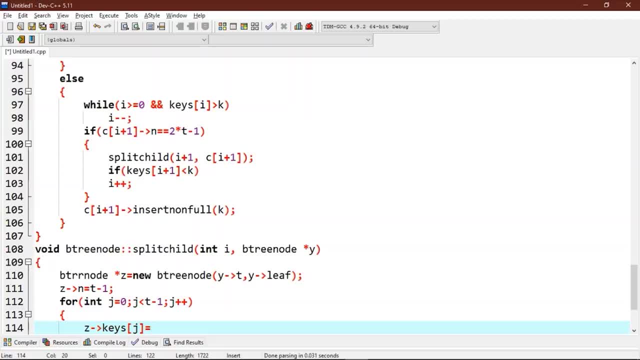 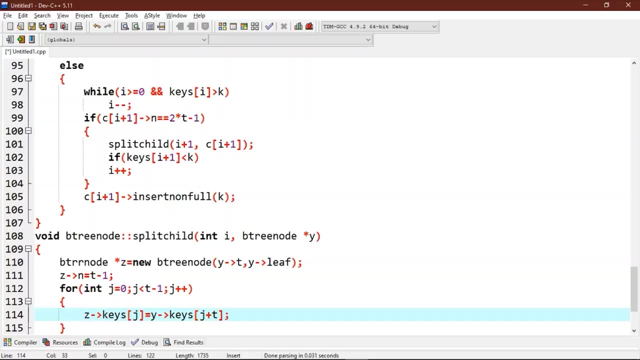 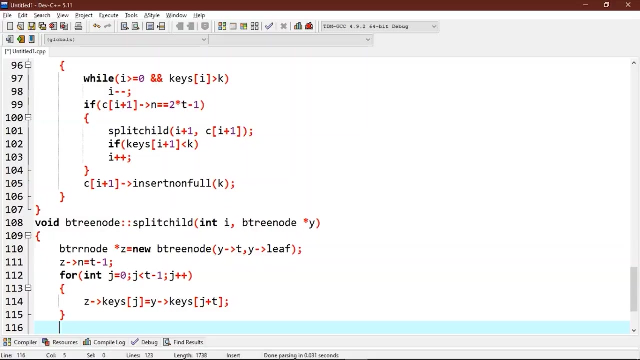 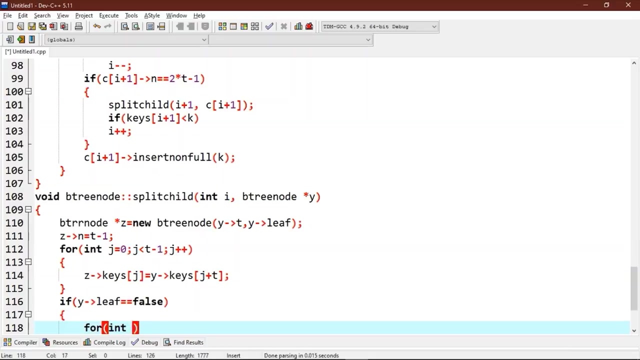 equals to y arrow keys j plus t. Now we will copy the last t childrens of y to z, So f y leaf is false. So for int j is equals to 0, j less than t and j++, So f. 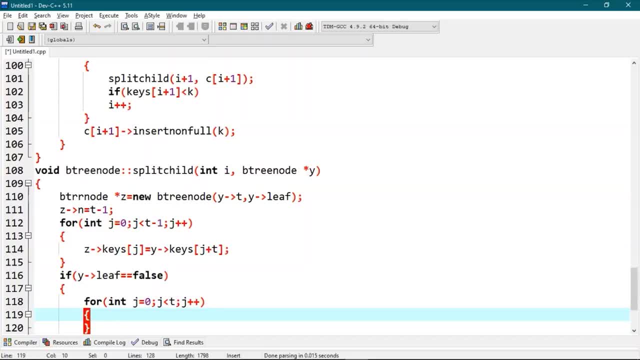 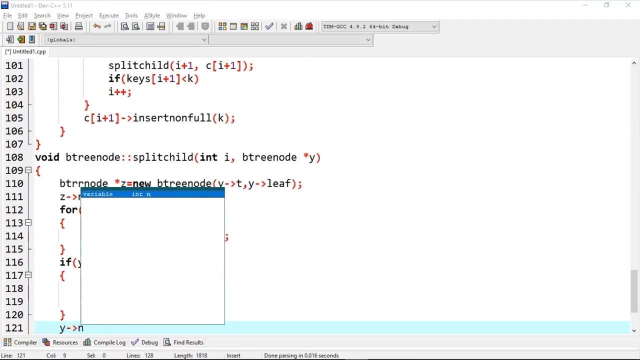 y. So z c j is equals to y, c, j plus t. Now we will reduce the number of keys in y y arrow. n is equals to t-1.. Now, since the node is going to have a new child, we 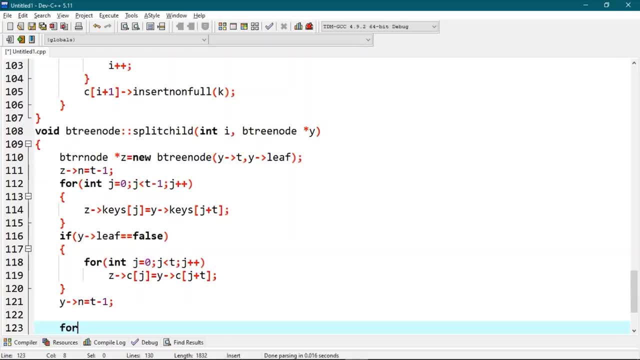 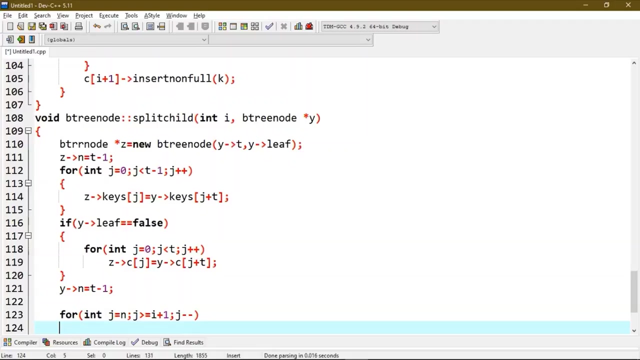 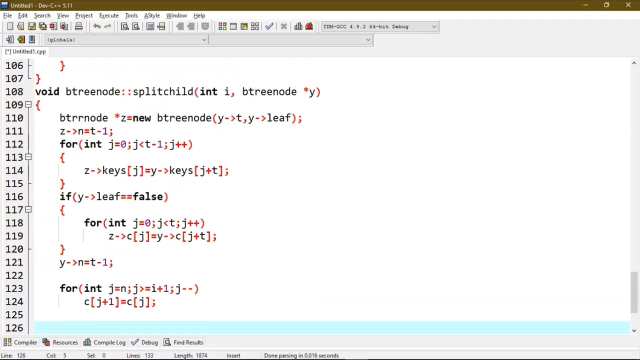 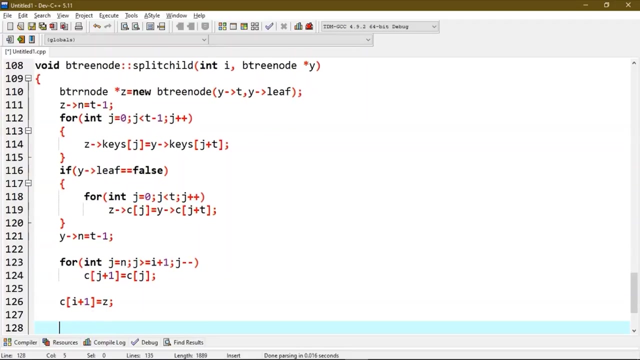 will create the space for the new child. so for int j is equals to n and j is greater than equals to, and c j plus 1 will be equals to. Now we will link the new child to this node, so C? y plus 1 equals to z. Now a key of y will move to this node, So we will find the location. 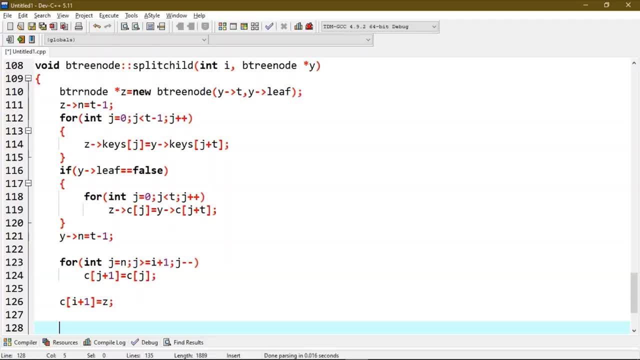 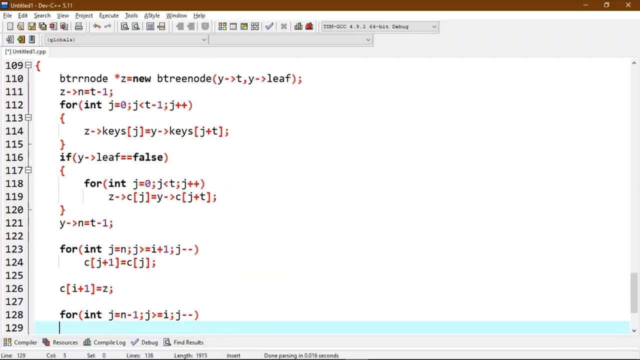 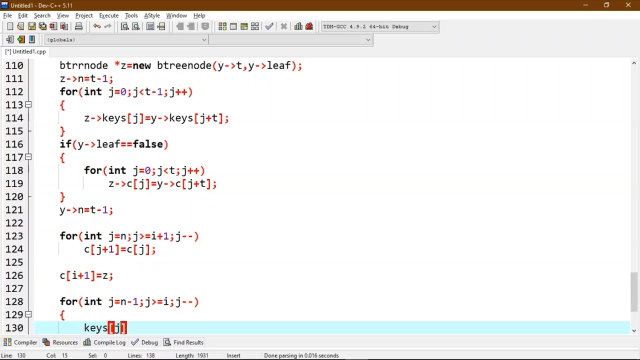 of new key and move all greater keys one space ahead. So for int, j is equals to n-1, j greater than equals to i. j minus minus is j plus 1 equals to n-1.. So we will find the location of new key and move all greater keys one space ahead Now. 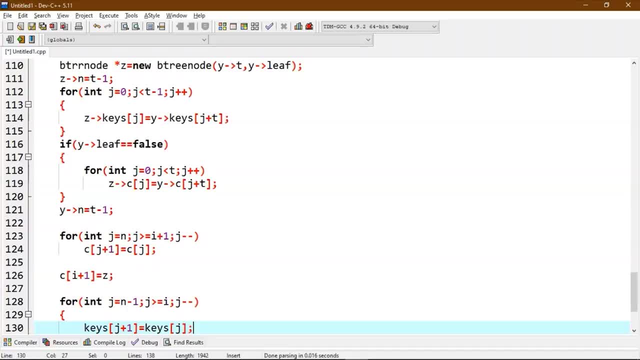 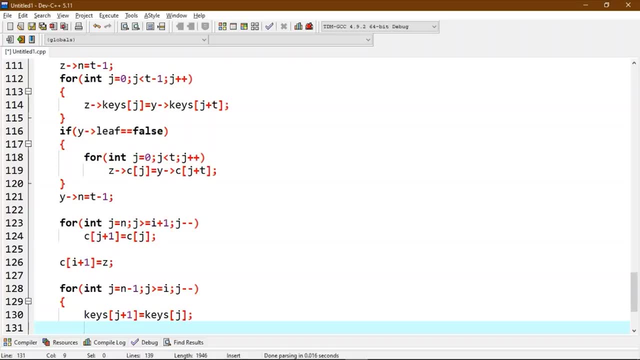 we will find the location of new key and move all greater keys one space ahead. So we will find the location of new key and move all greater keys one space ahead. Key is j. Now we will copy the middle key of y to this node. 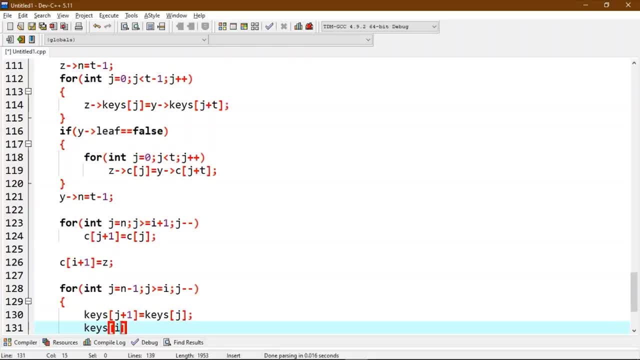 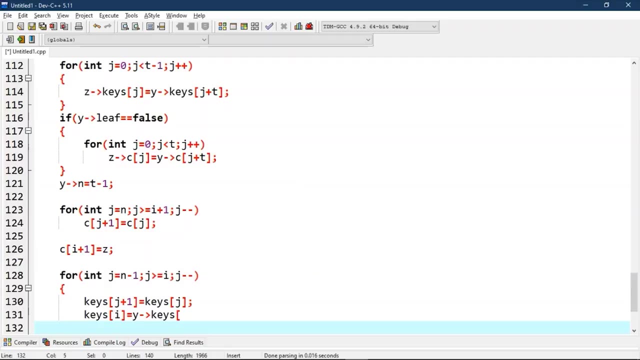 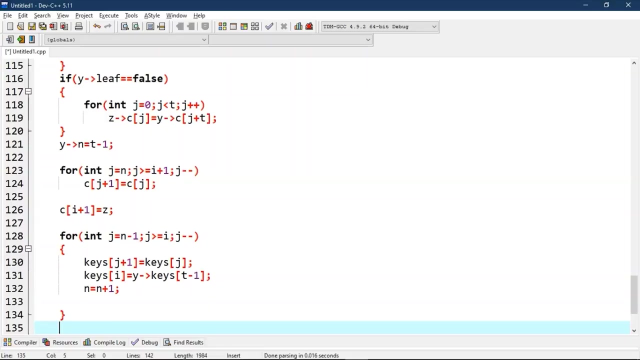 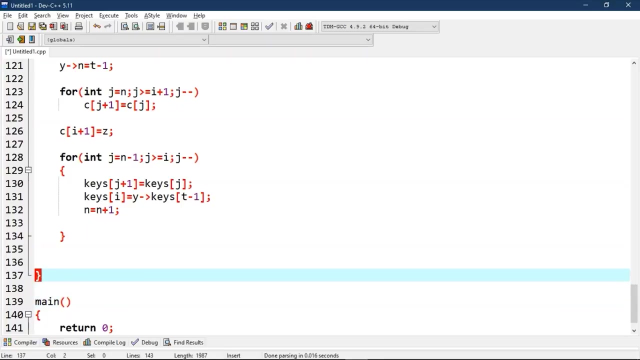 So key is bracket i is equals to y arrow. Key is at t-1.. Now we will increment the counts of key in this node, So n equals to n plus 1. Now we will write a driver program to test above functions. Now we will write the main block. 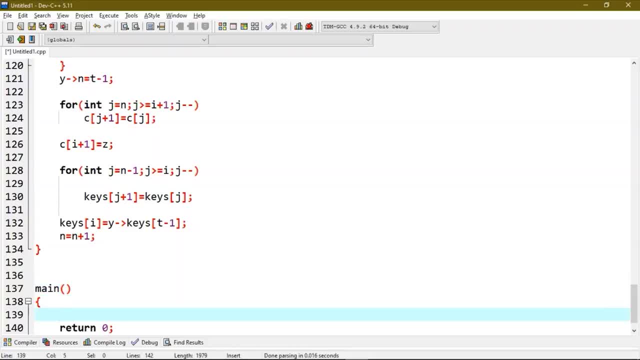 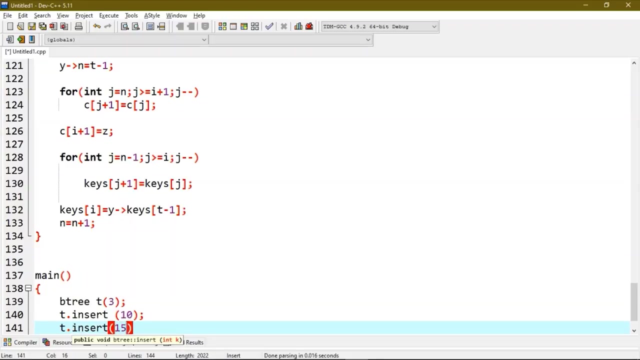 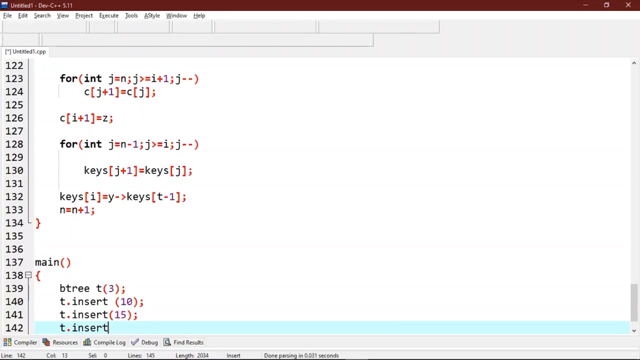 We will start with a B tree with menu of degree 3. Now we will write the main block. We will start with a B tree with menu of degree 3. Now we will insert keys in this tree: tinsert 10, tinsert 15, tinsert 5. 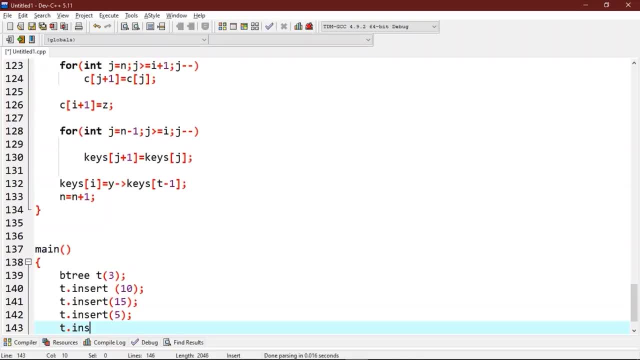 tinsert: 5 tinsert 6 tinsert, 7 tinsert, 8 tinsert, 9 tinsert, 10 tinsert, 11 tinsert, 12 tinsert, 13 tinsert, 14 tinsert, 15 tinsert, 16 tinsert 17. 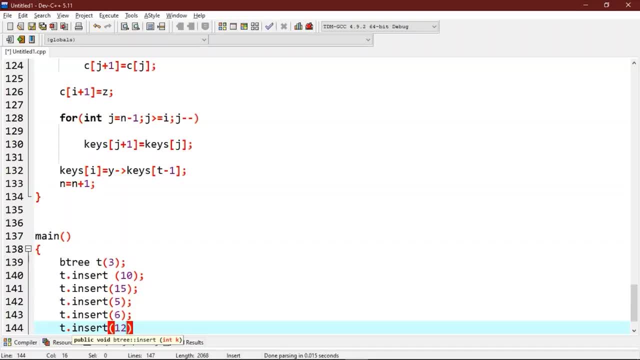 tinsert: 18 tinsert 19 tinsert, 20 tinsert, 21 tinsert, 22 tinsert, 23 tinsert, 24 tinsert 25 tinsert, 26 tinsert, 27 tinsert 28 tinsert 29 tinsert 30. 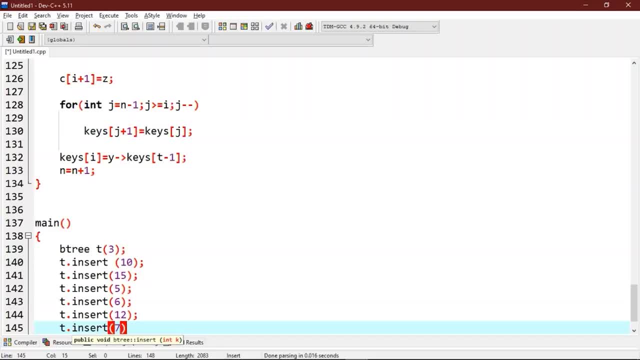 tinsert 31: tinsert 32 tinsert 32 tinsert 33 tinsert 34 tinsert 35 tinsert 38 tinsert 39 tinsert 40 tinsert 41: tinsert 42 tinsert 43: tinsert 44: 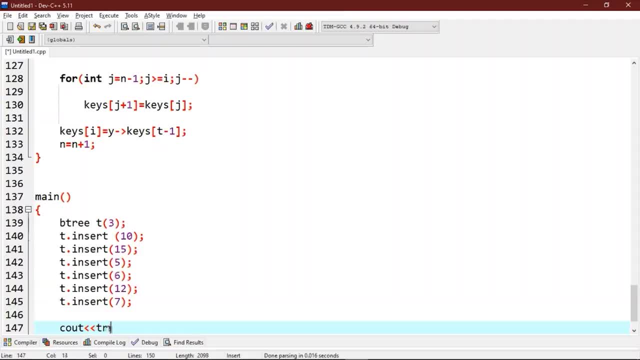 tinsert 45 tinsert 48 tinsert 49 tinsert 50 tinsert 51 tinsert 52 tinsert 53 tinsert 54 tinsert 55 tinsert 56 tinsert 57 tinsert 58 tinsert 59. 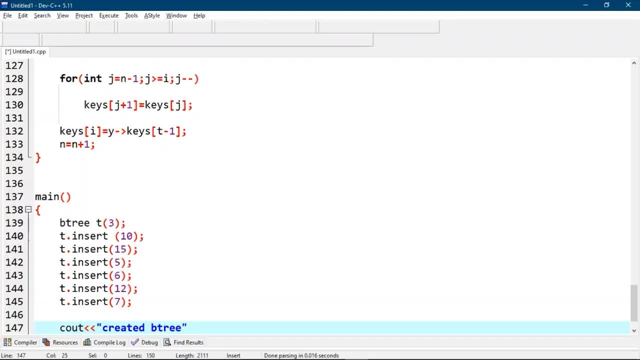 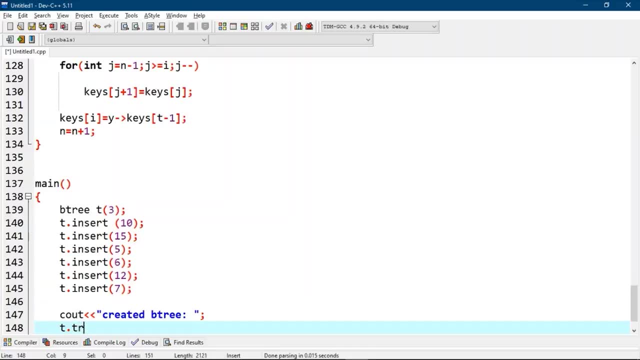 tinsert 60 tinsert 61 tinsert 62 tinsert 63 tinsert 63 tinsert 64 tinsert 65 tinsert 67 tinsert 68 tinsert 69 tinsert 70 tinsert 71 tinsert 82. 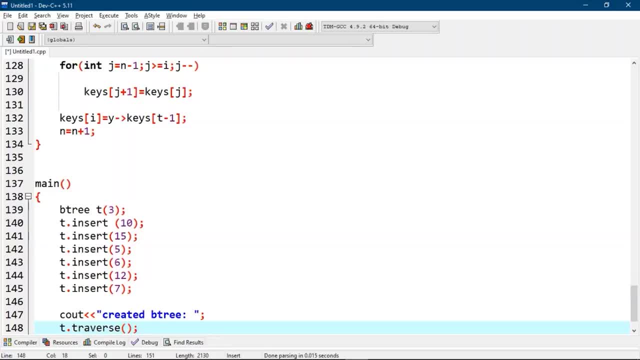 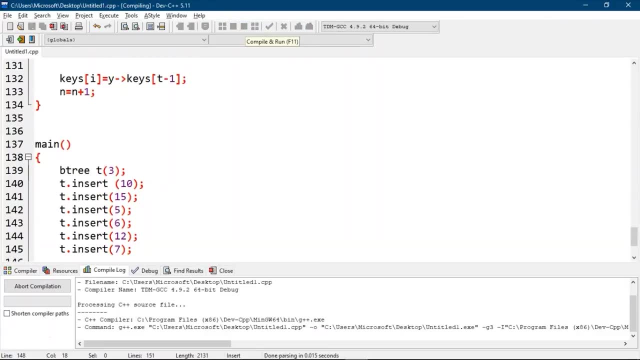 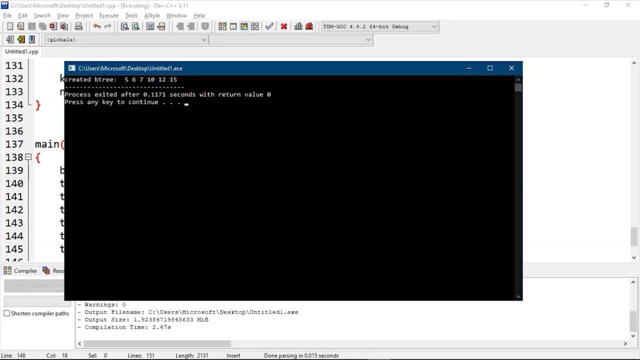 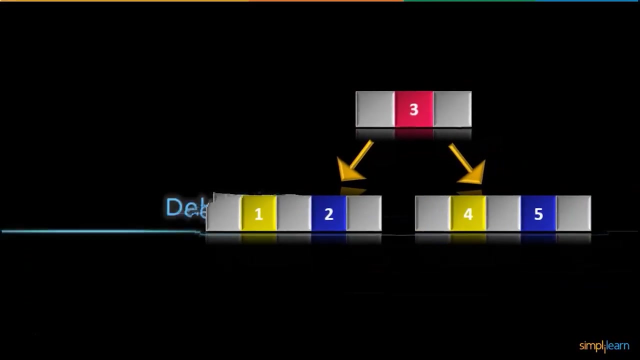 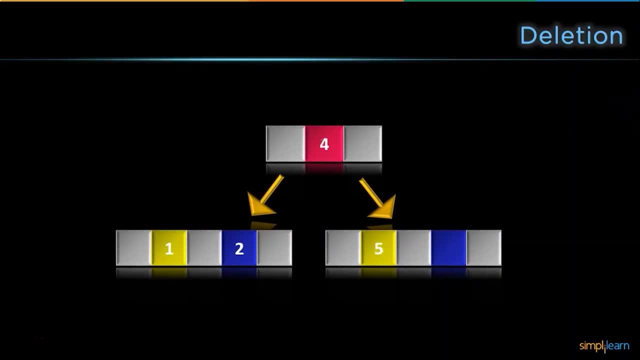 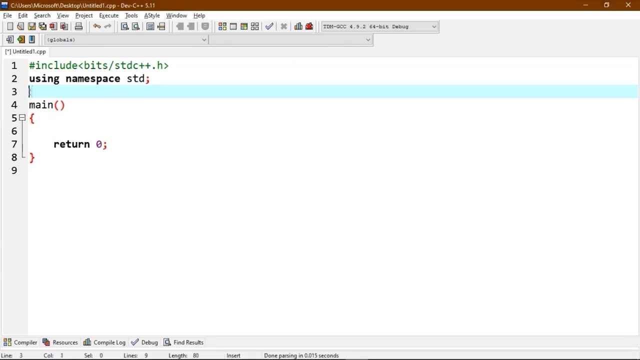 any elements from B tree. we have to be careful not to break any properties of the B tree. like all, the leaves must be present at the same level or elements must be in ascending order. now let's try this operation in a code editor. let's start by creating a node. to create a node, we need a class: node, int start. 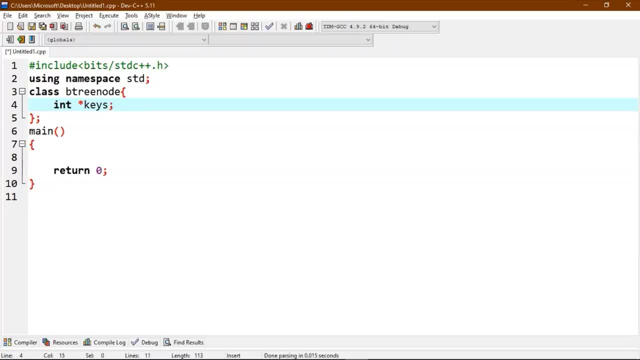 keys. this is an array of keys: int t, a minimum degree. now we will define an array of child pointers, so B, tree node, and a number of keys. int n, a boolean variable leaf, to tell us if the node is leaf or not now. now we will define some public functions. 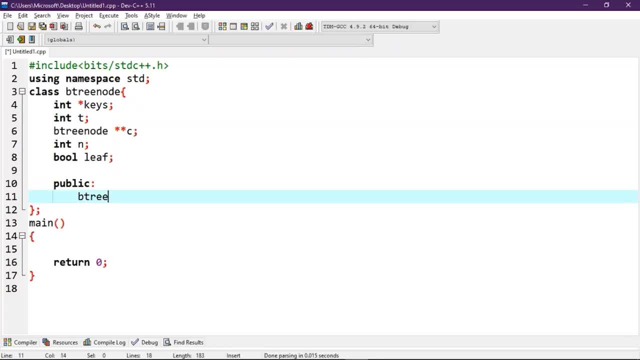 we will start with the constructor less class B tree node int underscore T boolean. no, not, no, sorry, no, no, o min, min underscore leaf. and a function to traverse the all nodes in the sub-routed tree, so void traverse. now a function to search a key in the sub-tree, so btree node, star search. 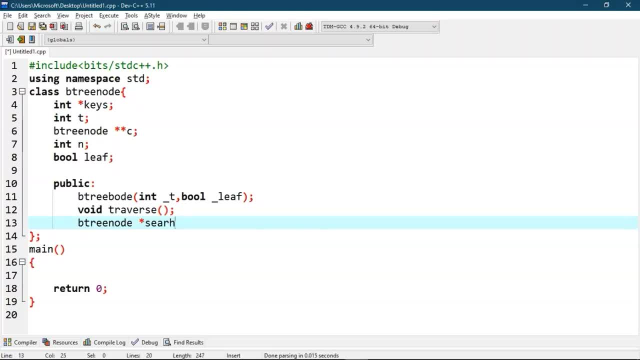 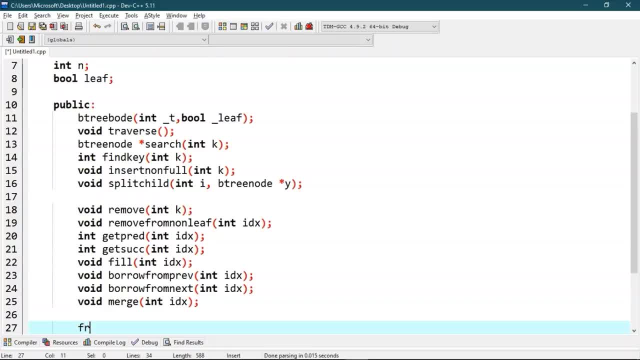 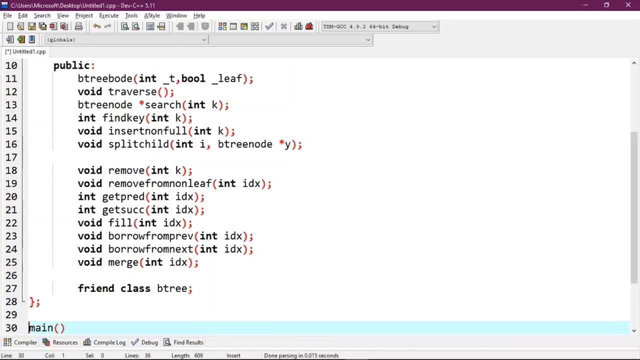 now we will write an utility function to enter a key in the sub-tree node star search. now we will write an utility function to enter a key in the sub-tree node star search. now we will write an utility function to enter a key in the sub-tree node star search. 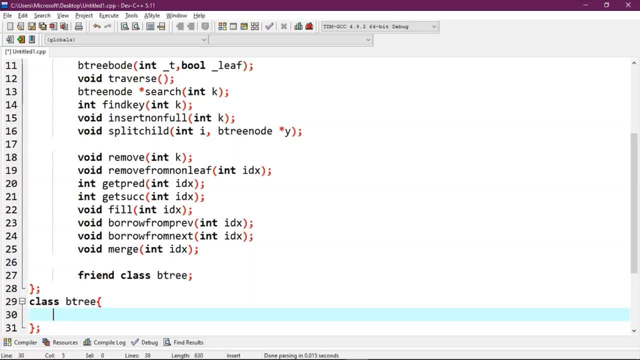 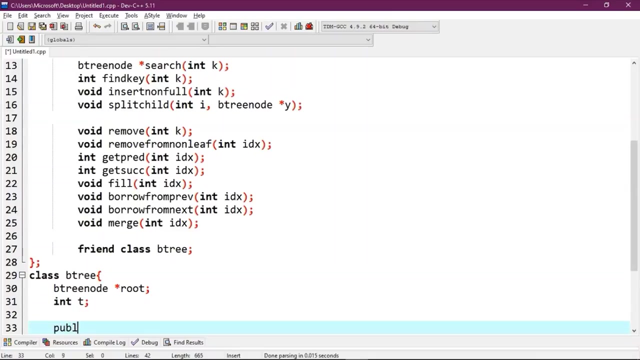 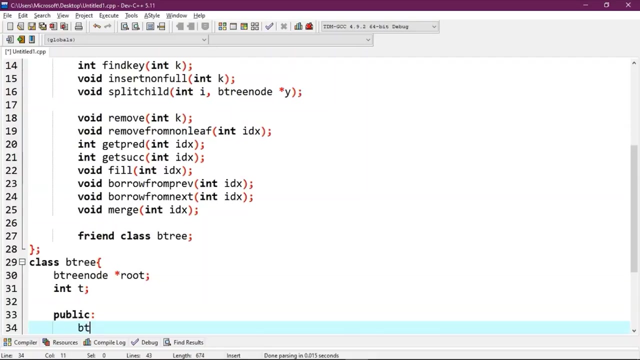 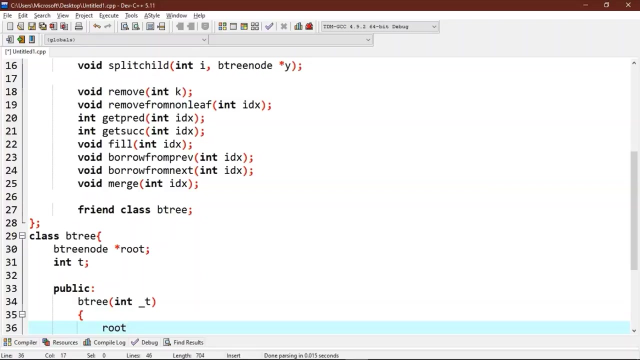 We will start with the pointer to the root node. so btree node, star, root and t. Now we will write some public functions. we will start with the constructor: So btree int underscore t. So root is equals to null And t is equals to null. 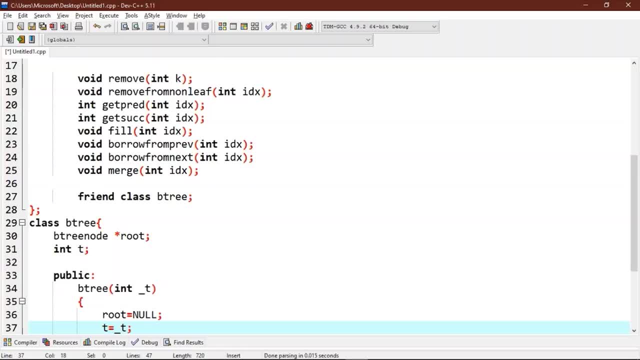 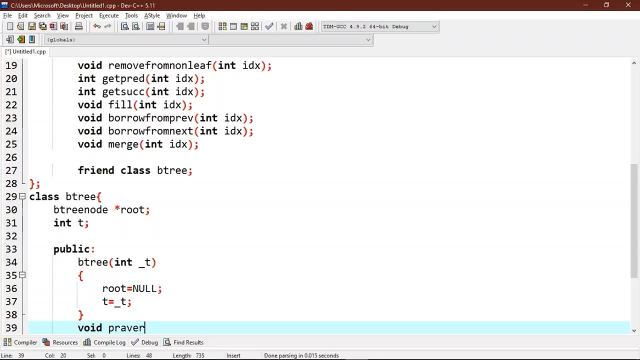 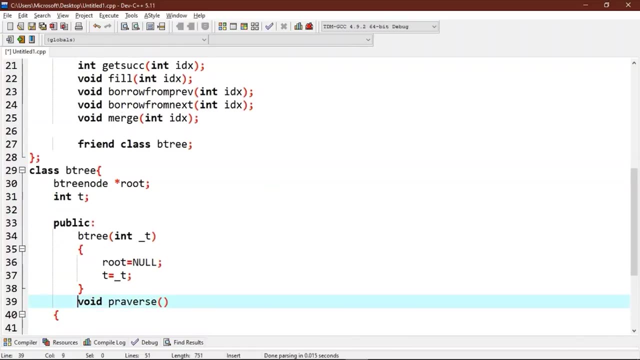 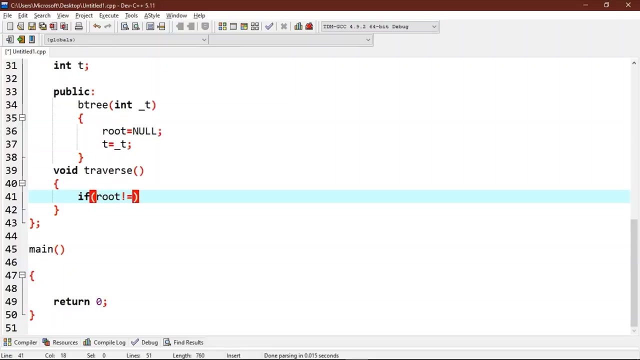 So btree. int. underscore t. Now a traverse function, void traverse. So we will check. if root is not null, Then root arrow traverse. Now we will write a function to search a key in this tree. So btree. Now we will write a function to search a key in this tree. 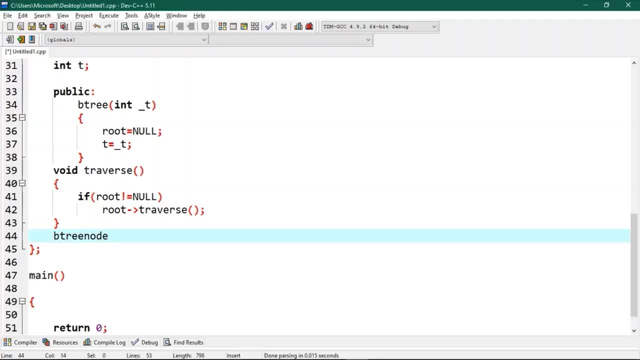 So btree Now, if we search a key in this node, search int k, we will return f. root is equals to null, So function will remove. Then we will return NULL, else root. arrow search at key. Now we will write the main function that inserts a new key in this b-tree. 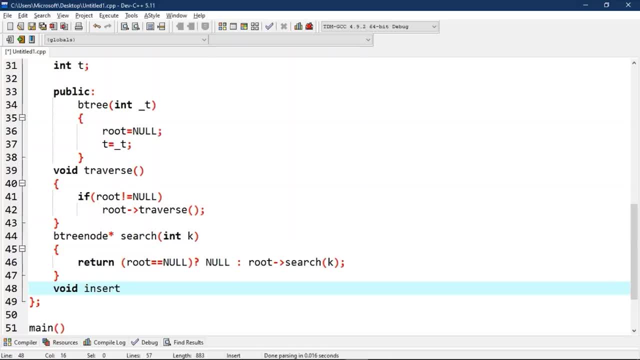 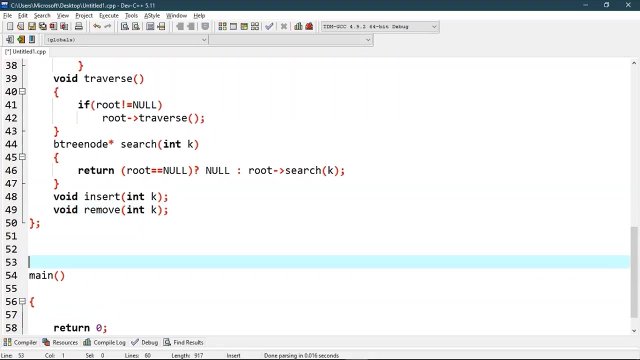 So void, insert int k. Now another main function that removes the new key in this b-tree. So void: remove int k. Now we will write the constructor for this b-tree node as int k. Now we will write the constructor for this b-tree node as int k. 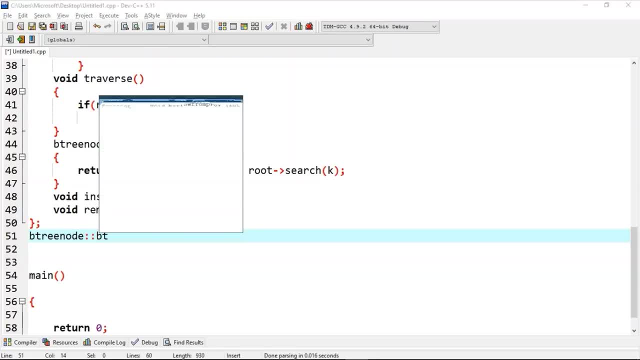 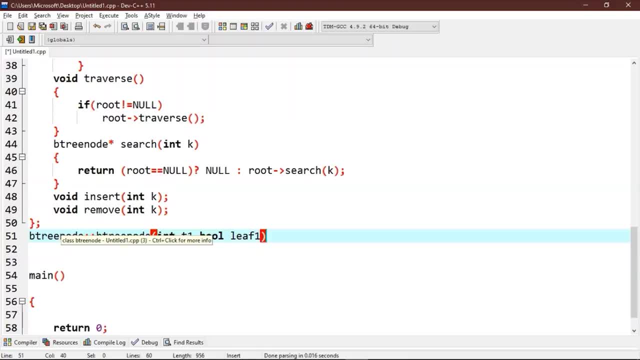 So t will be equals to t1 and leaf will be equals to leaf1.. Now we will allocate memory for the maximum number of possible keys and child pointers. So keys is equals to new int bracket 2, star t minus 1 and child c is equals to new btree. 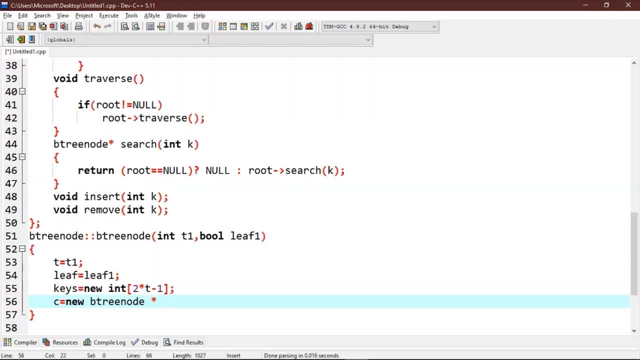 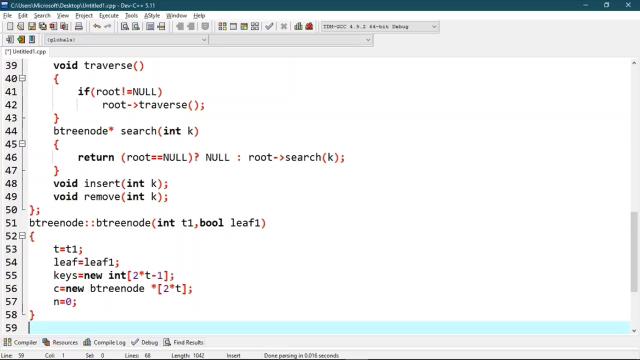 node: star bracket 2, star t. Now we will allocate memory for the maximum number of possible keys and child pointers. Now we will initialize the number of keys as 0. So n is equals to 0.. Now we will write a utility function that returns the index of the first key, that is: 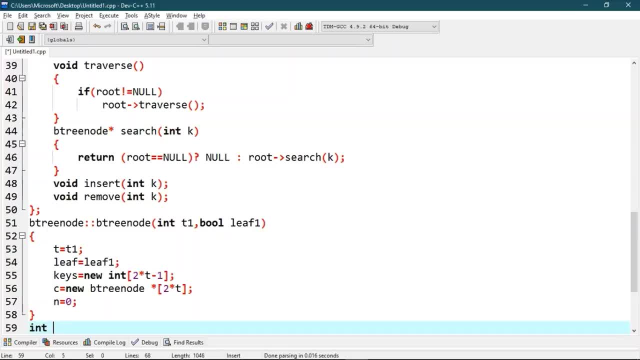 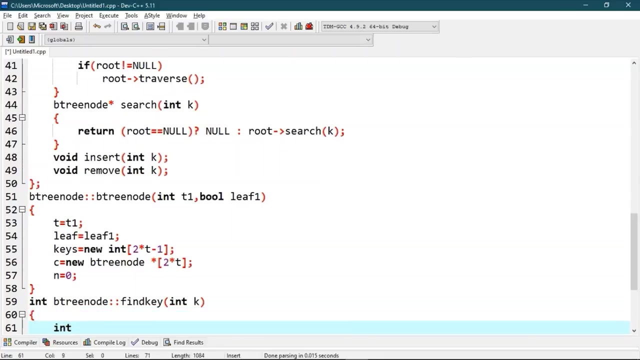 greater than or equal to k. So int btree node find key. Now we will write a utility function that returns the index of the first key that is greater than or equal to k. So int k Now int idx, is equals to 0.. 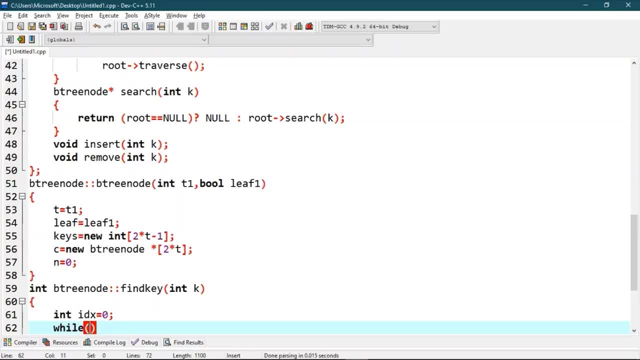 Then, while idx is less than n And keys is equal to 0. Now we will write a utility function that returns the index of the first key that is greater than or equal to k. Now int idx is equals to 0. So int k is equal to 9.. Then the number of keys that returns the index of the first key is also greater than or equal to 9.. Now int k is 2. if k is greater than or equal to 3 and 2 is equal to 3 and 3 is equal to. 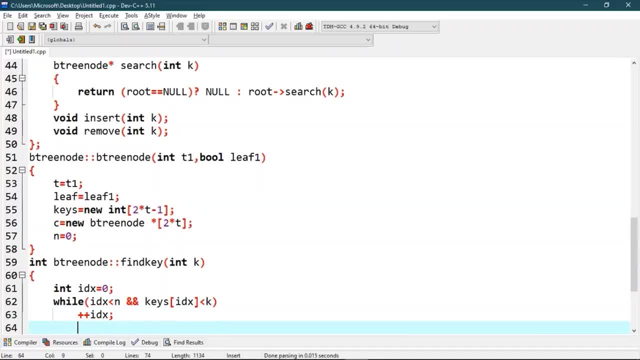 0.. Now int m is equal to k. Next we will write the result in the poking point world for whites and merges. Now we need to write a limit number which equals to a value of multiple digits. After this, int place isös plus dk. 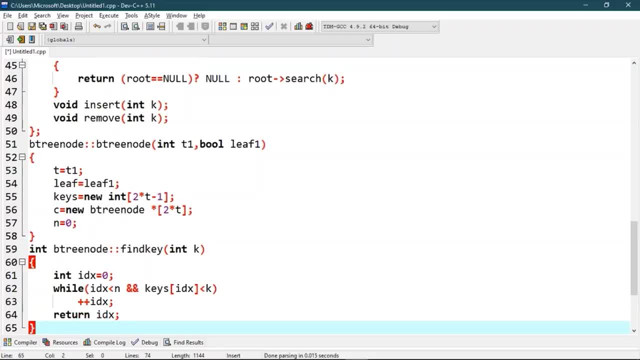 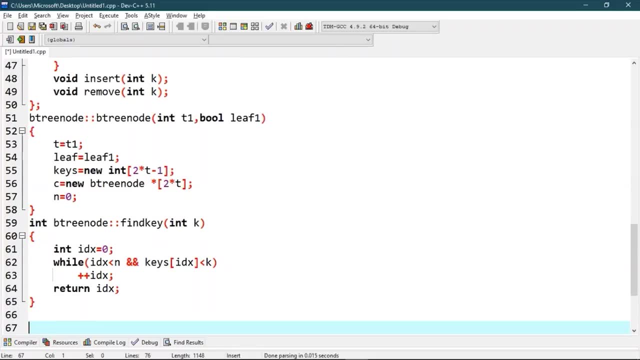 bP wool by in and out k. //P f nano platforms. call♡ mS ihm plusfeito Seong ‑‑. version w. Now we will write a function to remove the key k from the sub-tree rooted with this node. void btree node: remove int k. 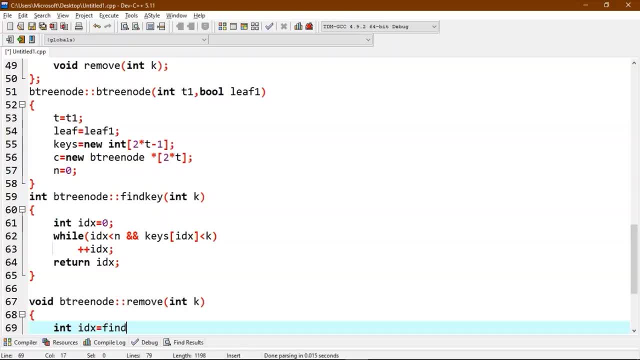 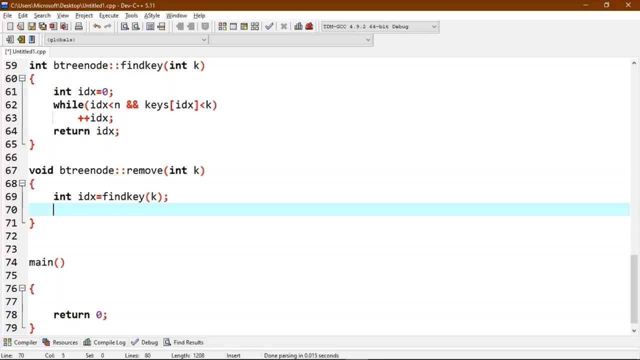 int idx equals to point key k. if the key to be removed is present in this node, then if idx is less than n and keys at idx is equal to k is equal to k. now if node is leaf node then we will remove from. leaf node is called. 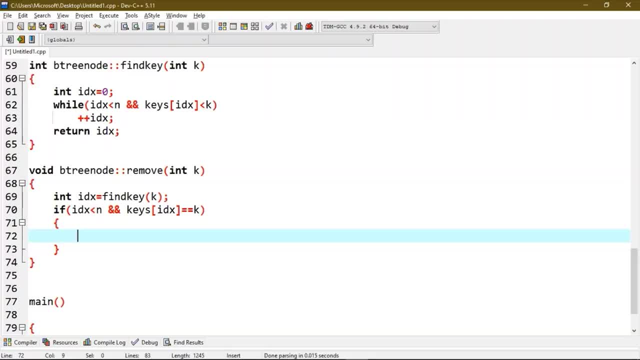 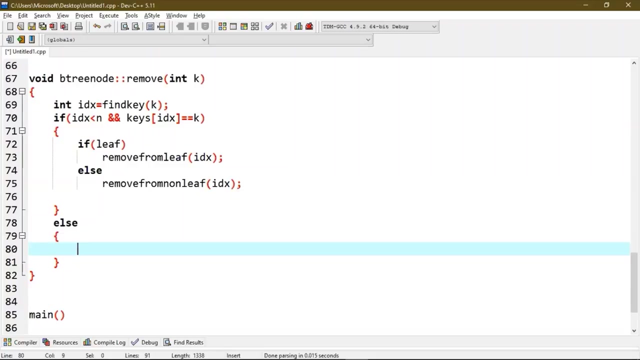 otherwise remove from non-leaf function is called. so if leaf, then remove from leaf idx, else remove from non-leaf idx now. else if this node is a leaf node, then the key is not present in the tree. so if leaf is a leaf node, then the key is not present in the tree. 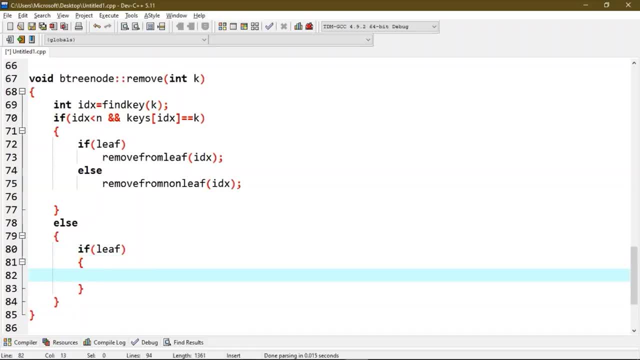 now else leaf node is also present in the tree and if the link distribution isharmonnet then we will use leaf node between side. so if critique node is cli z and if already c Lima, this is obviously zero, does not exist in this tree. The key to be removed is present in this subtree rooted with this node. 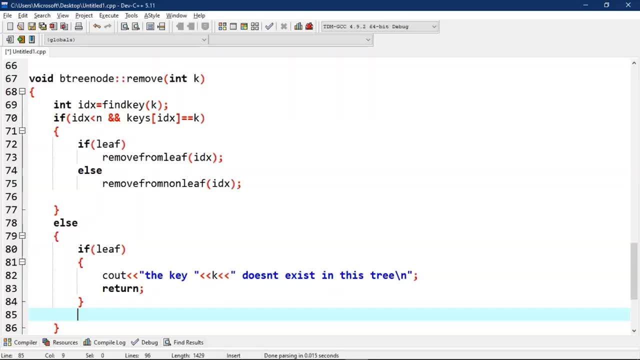 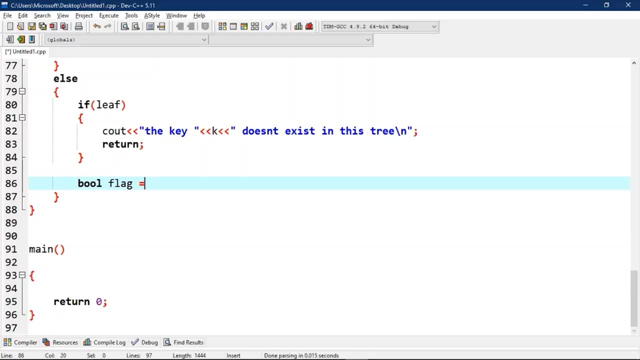 The flag indicates whether the key is present in this subtree rooted with the last child of this node. So bool flag is equal to idx, equals to n, if. if. if it is true, else false. If the child where the key is supposed to exist has less than t keys, then we fill that. 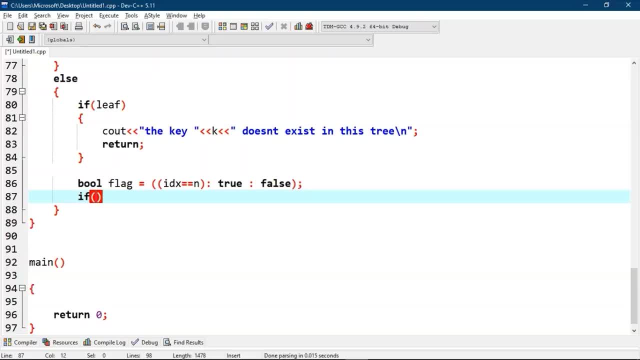 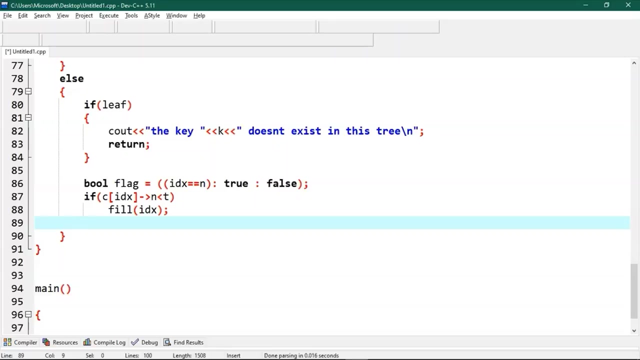 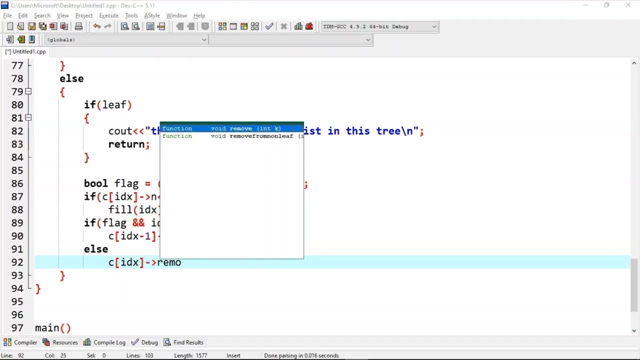 child. So if C at IDX N is less than T, then fill IDX. Now if flag and IDX is greater than N, then C IDX minus 1, remove A Else C IDX. remove A. Okay Return. 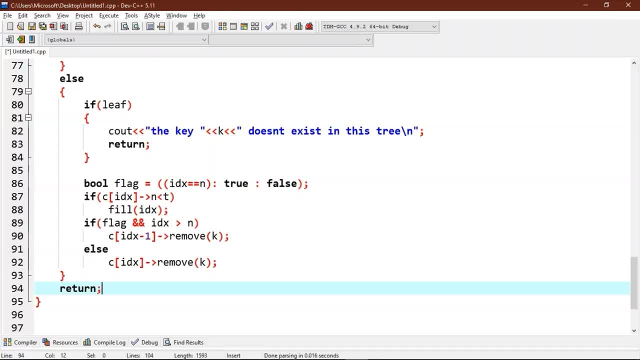 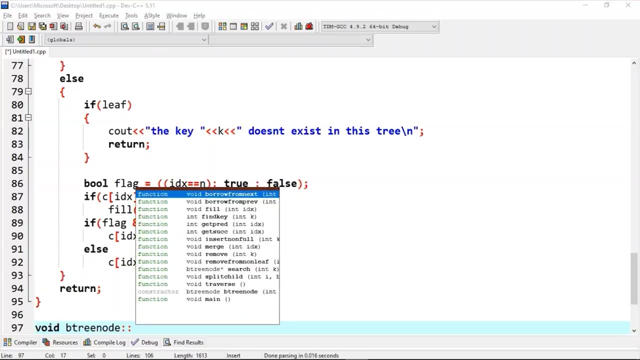 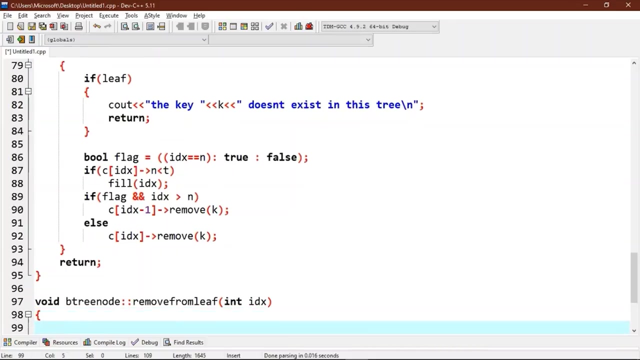 Avoid B tree node. Remove From leave From leave And IDX. Now we will move all the keys after the IDX position one place backward. So for loop int i is equals to IDX plus 1.. IDX plus 1.. 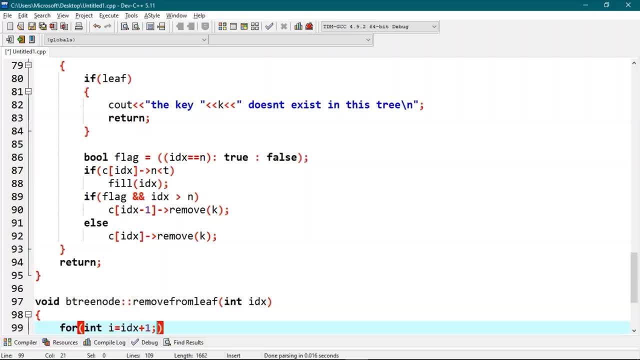 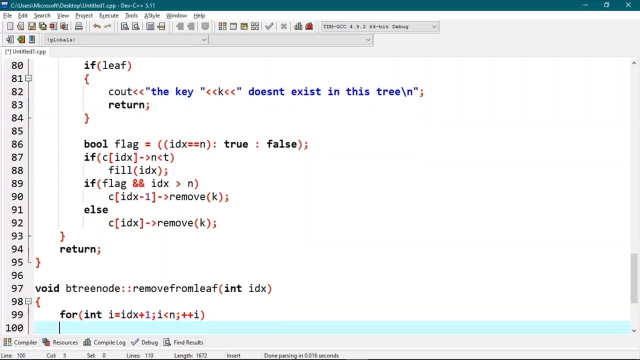 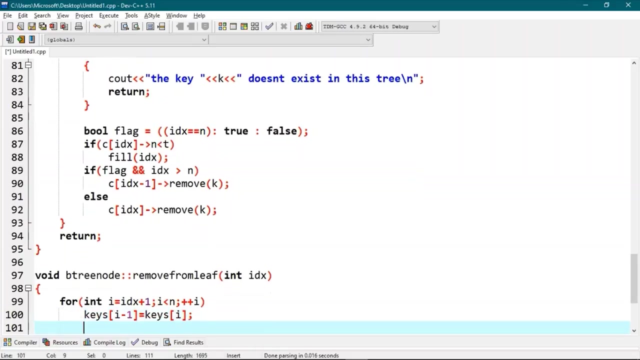 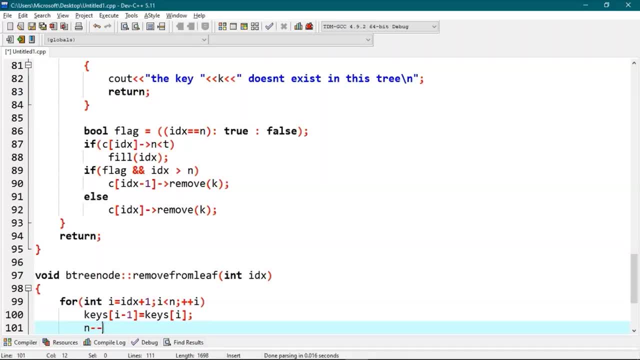 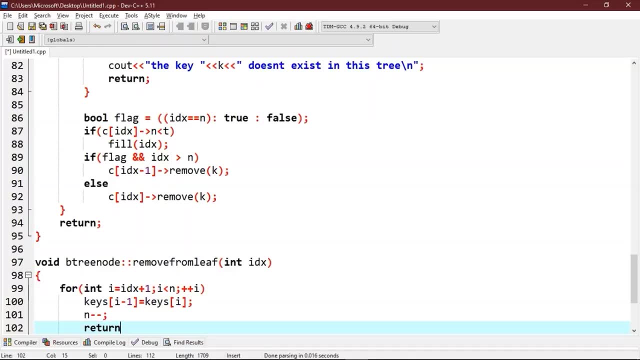 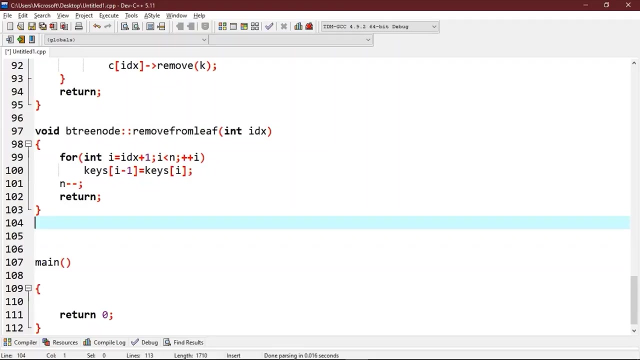 And we will reduce the count of keys. So N minus minus, Then return. Now we will write the function to remove the IDX key from the node which is non-leaf node. So void Leave tree node remove. 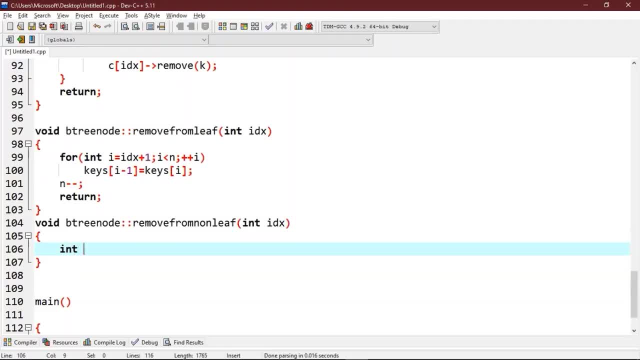 And then worked the day, So set to NOT IDX. So this calls for remote. Now you will resident 그리고 you will also see that. so we did not do theeme regularly. but I did not state the number tag. save the copy as Terra or not just the name. 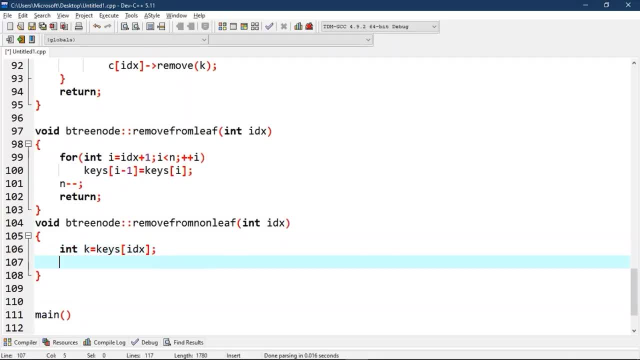 And then I am going to delete this part. Now, to delete this part, you will note, you can use two variables, And so that will give one by one, including the information that we put into the 내용. Nah, If the child that precedes K at CIDX has at least T keys, then we will find the predecessor. 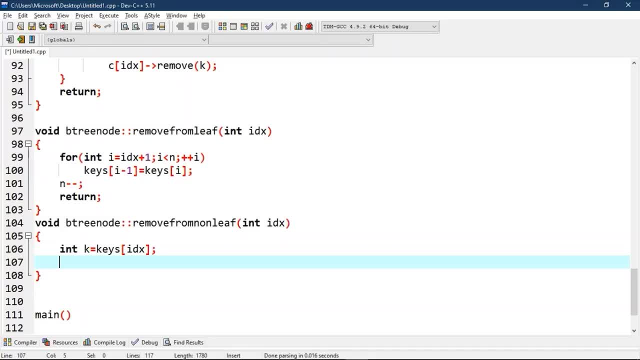 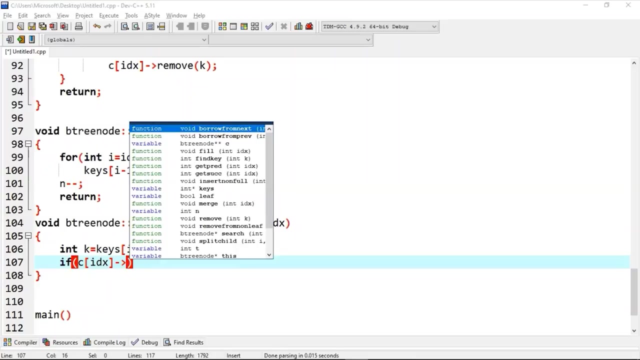 pred of K in the subtree rooted at CIDX. We will replace K by predecessor recursively and delete pred in CIDX. So if CIDX arrow N is greater than equals to T, N is greater than equals to T, N is greater than equals to T. 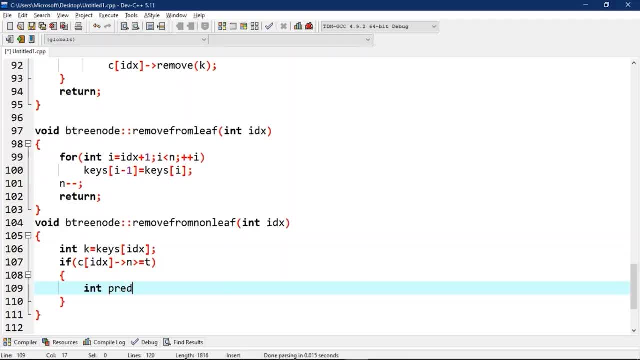 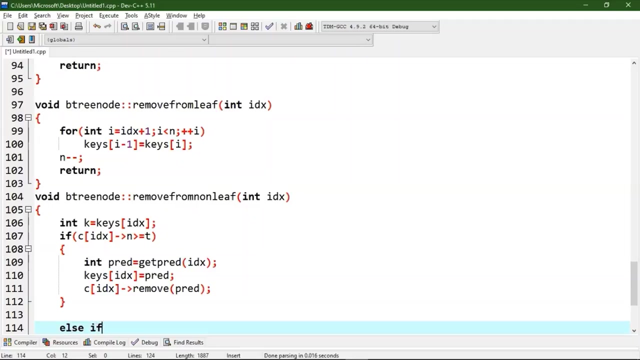 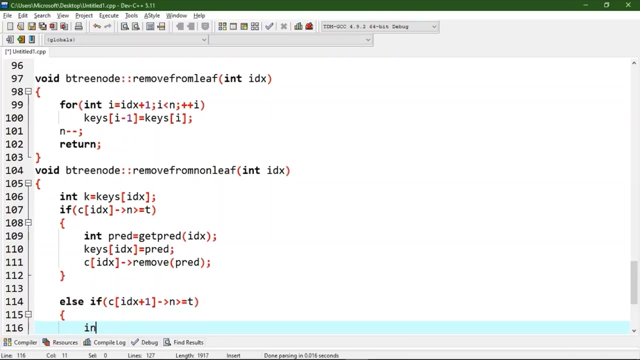 then int pred equals to get pred IDX keys. IDX equals to pred CIDX. remove pred else. if C at IDX plus 1 arrow N is greater than equals to T, then int pred equals to看到 if we want to remove pred IDX, if we want to remove pred IDX. 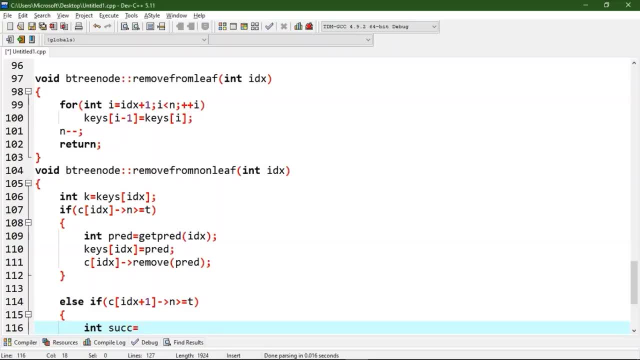 then int practically identity. so I will remove pred IDX, add Gamut I. if we want to remove pred IDX, add Gamut IDX. if we want to remove pred IDX, then the pred IDX entered as That. take maximum immigrants size: that as mustard, that as seed, that as Z and Z unpcomes. parent 564ition files at콜. 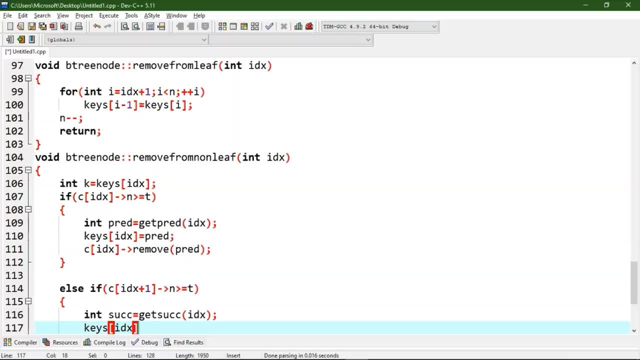 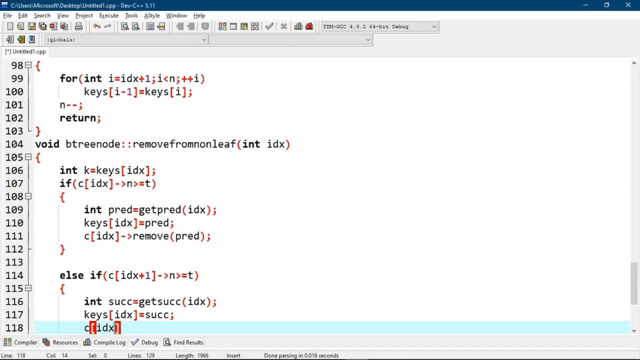 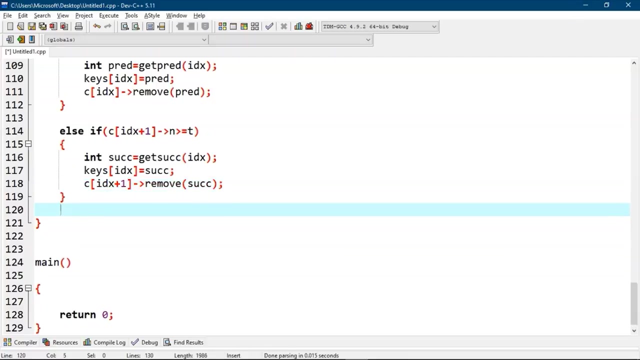 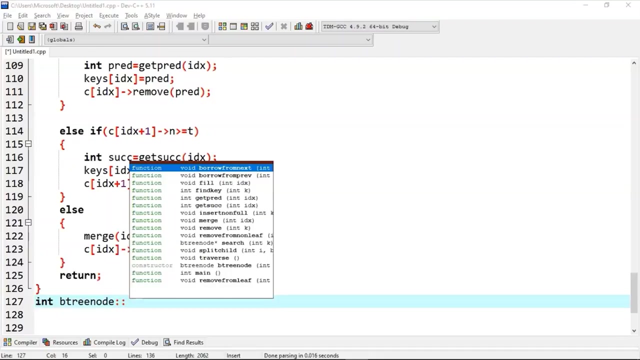 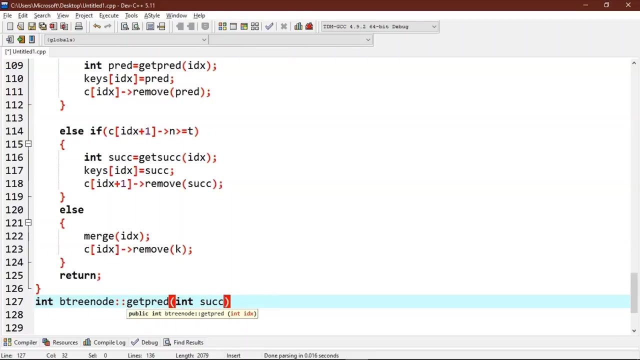 equals to at ID X is equals to suck. see at ID X plus 1 uses remove. sir, else will merge ID X and see at ID X will call remove. he at ID X will call remove, return. now we will write a function to get predecessor of keys ID X. so int B tree node, get bread and suck, repeat and. 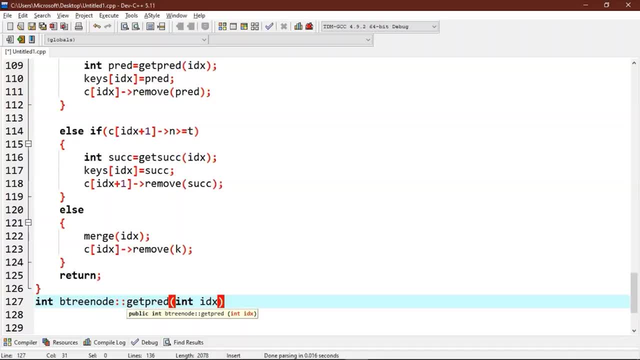 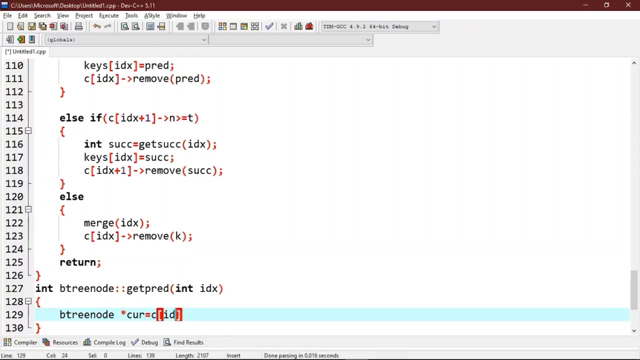 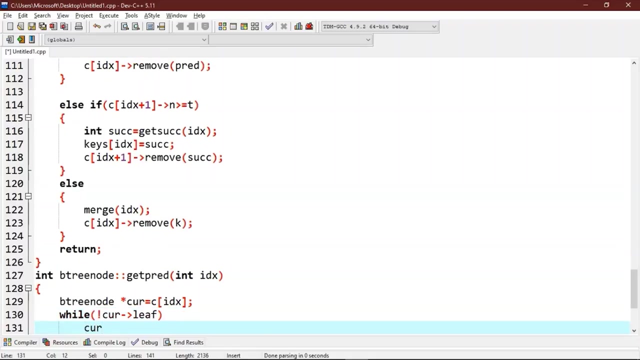 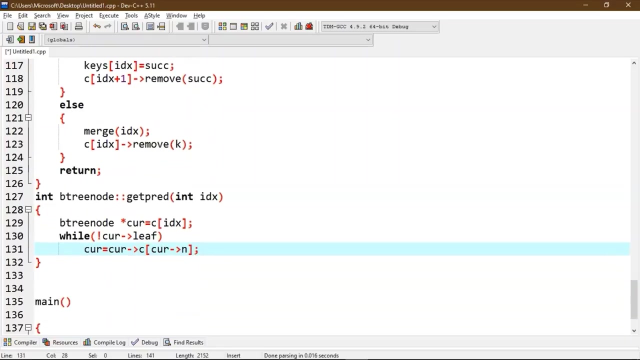 ID X. so B tree node, star curve is equals to C at ID X, while or is not, a leaf then will be equals to the arrow. see girl calls. and now we will return car key. now we will write and B tree node get suck. now we will write and B tree node get suck. 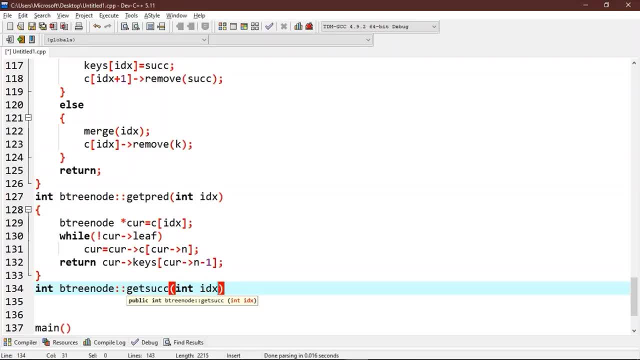 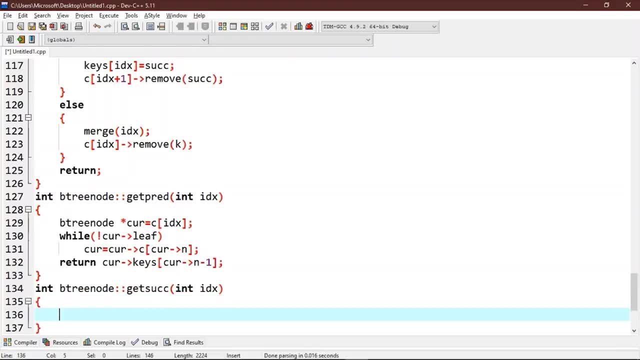 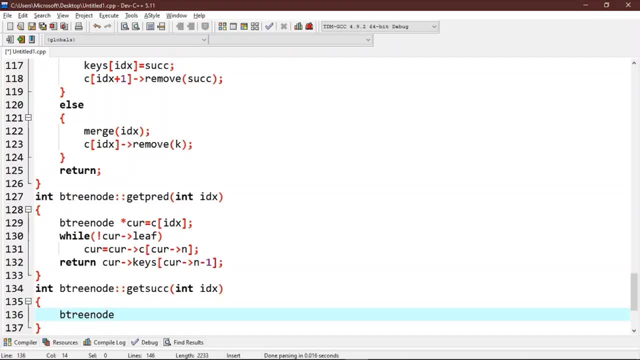 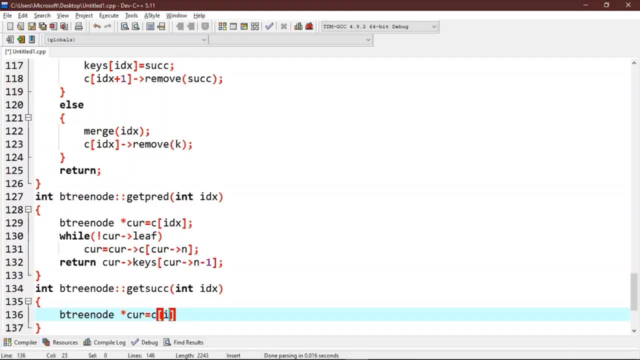 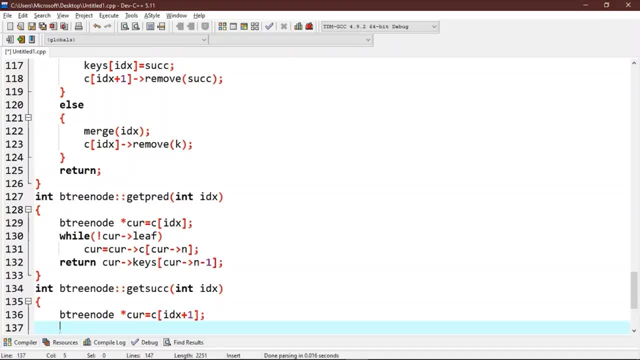 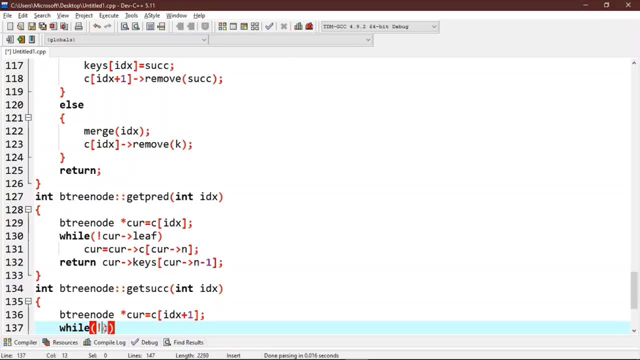 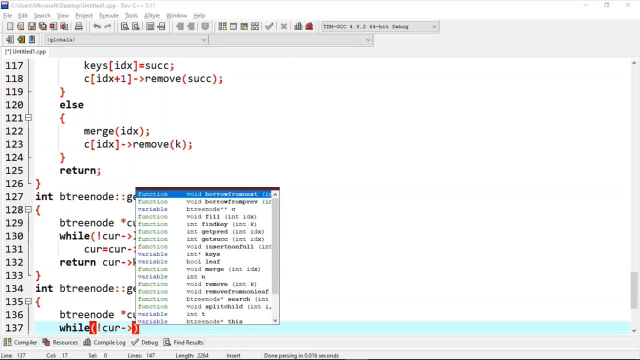 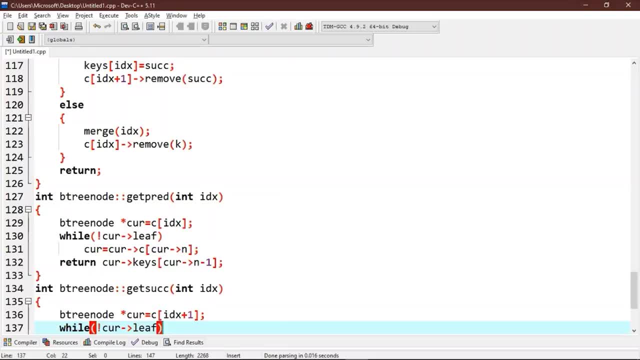 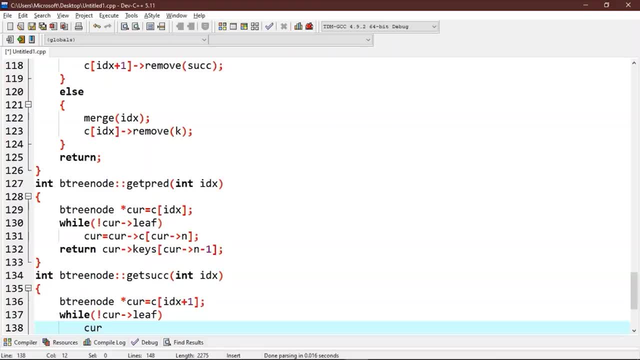 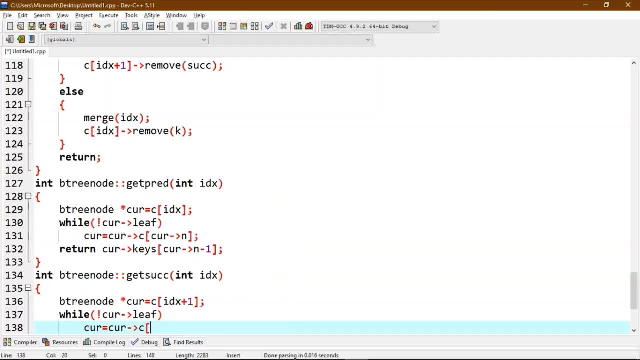 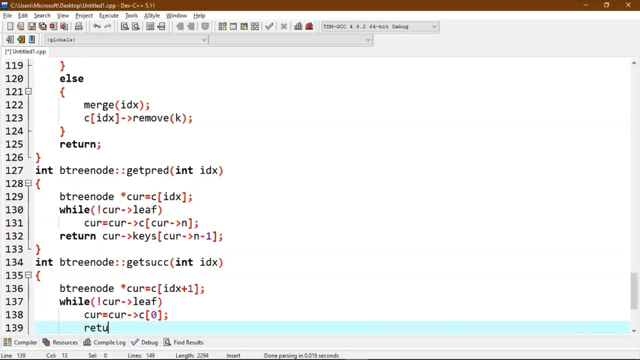 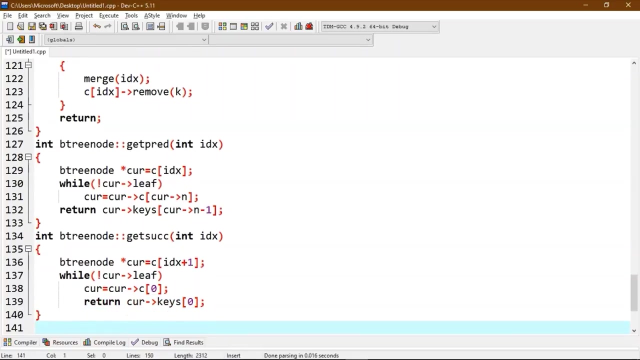 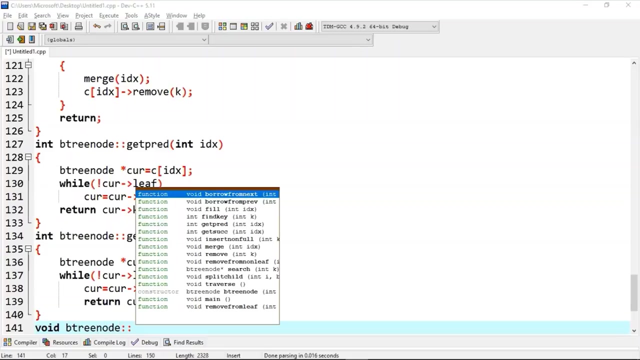 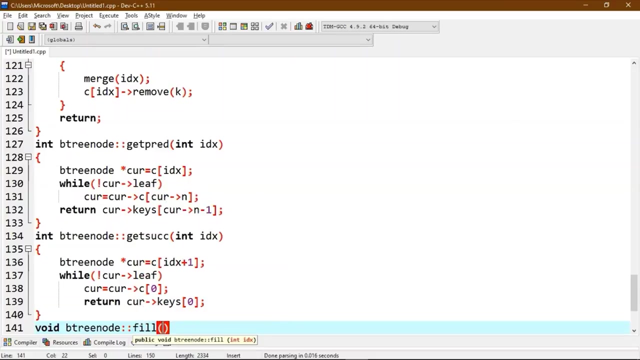 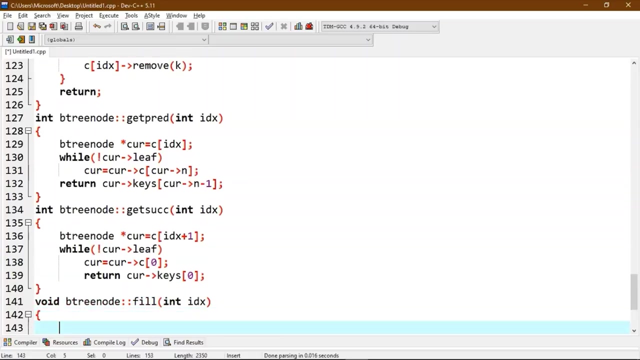 now we will write and B tree node get suck. Now we will write a function to fill child cidx which has less than t-1 keys. void btree node fill and irx repeat: if the previous child cidx-1 has more than t-1 keys, then we will borrow a key from. 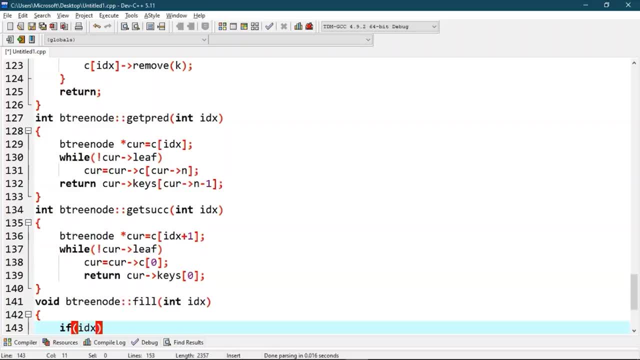 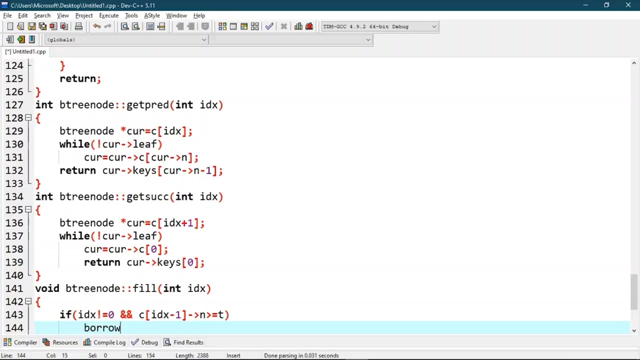 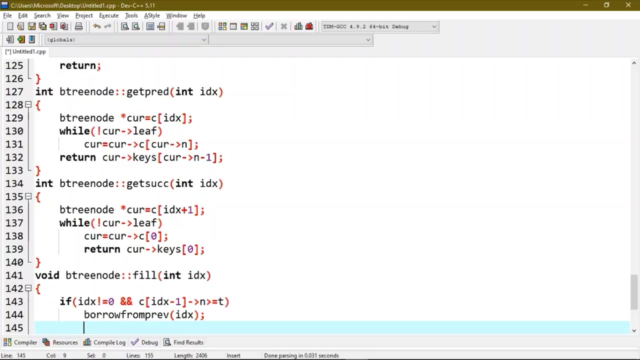 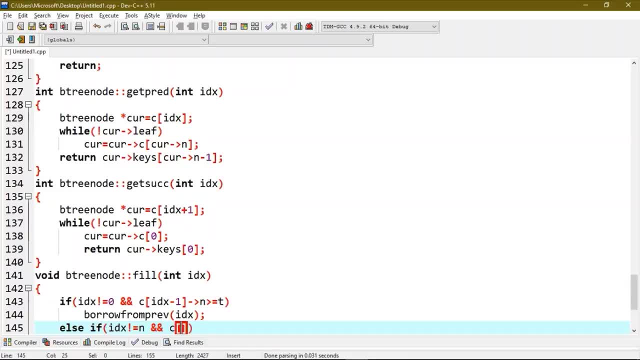 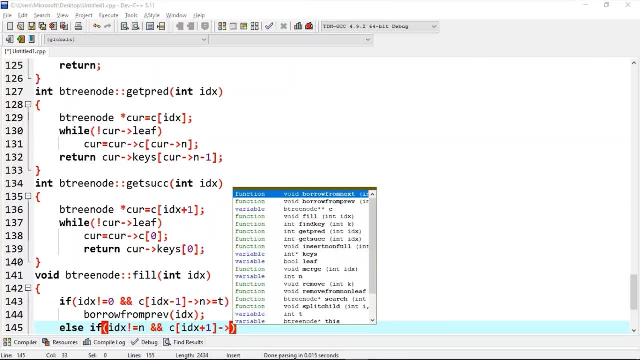 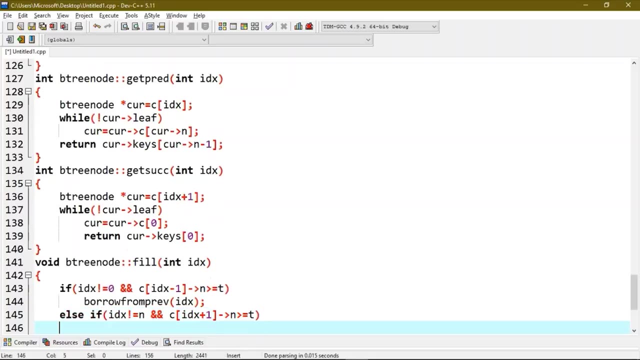 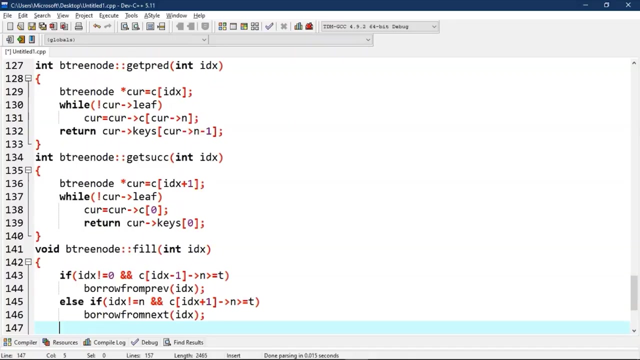 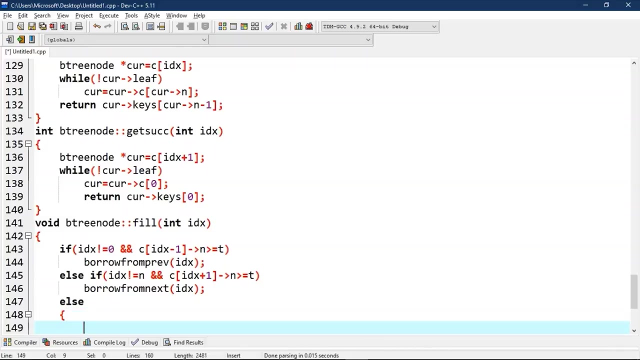 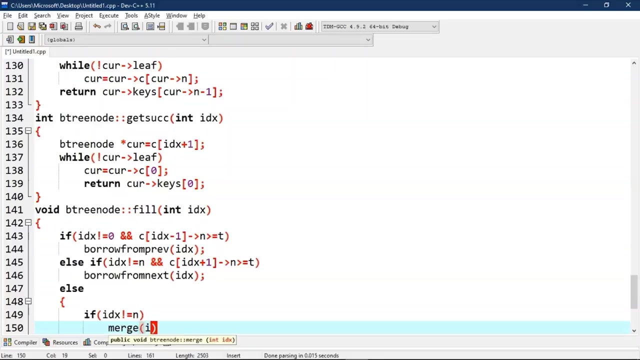 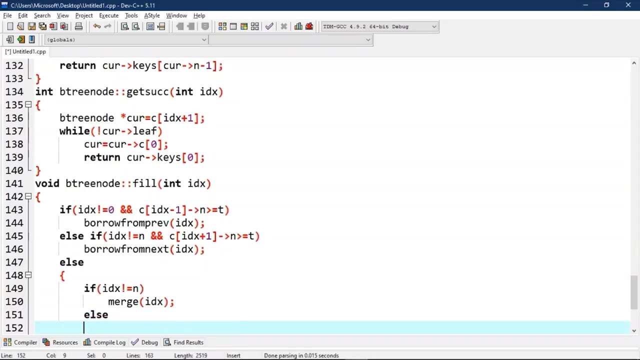 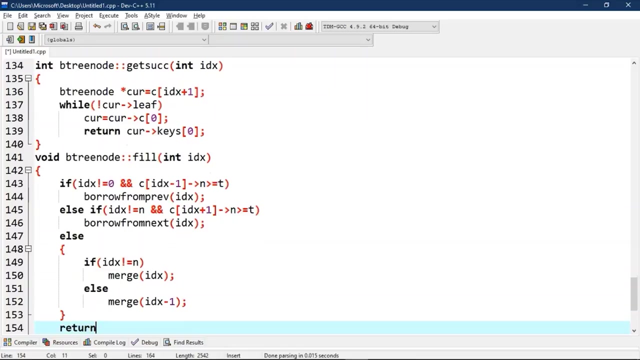 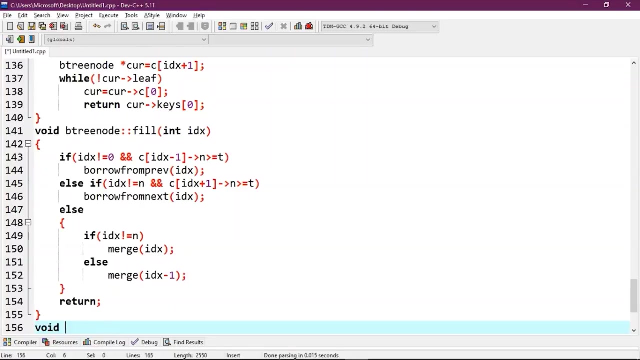 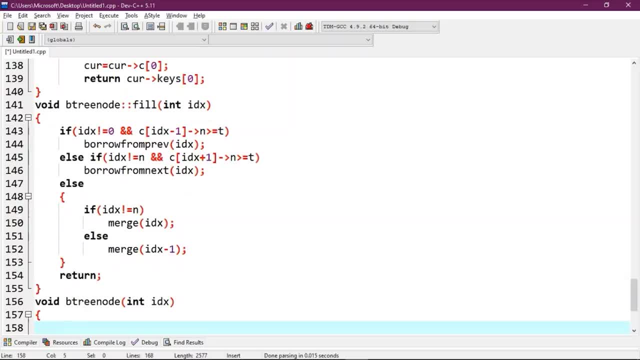 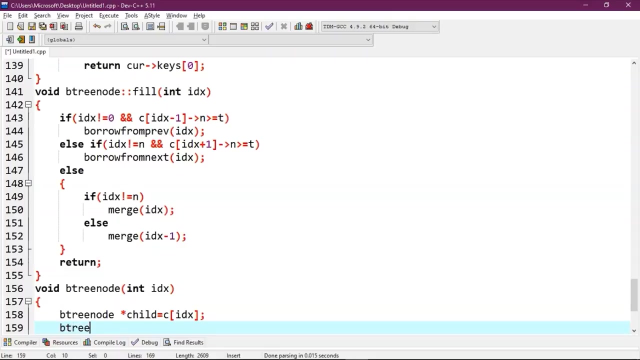 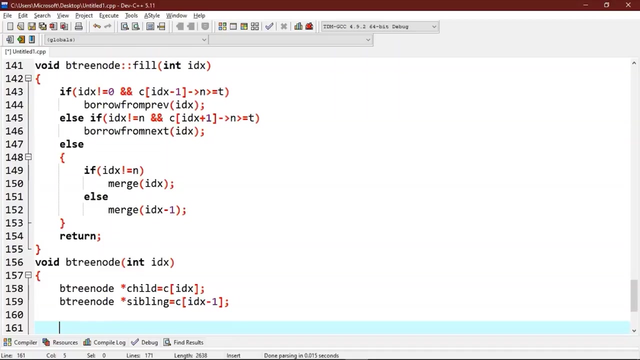 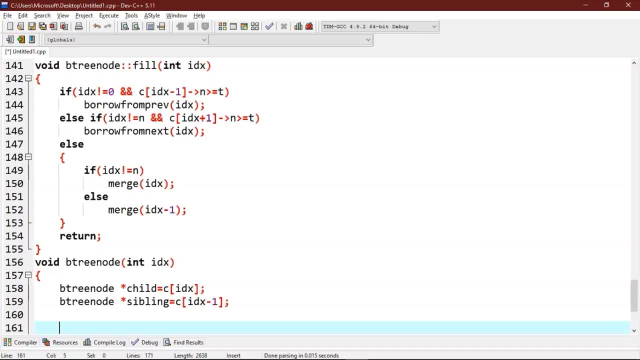 idx. idx inserted as the first key in CIDX. Thus the losses sibling one key and child gains one key, moving all keys in CIDX one step ahead. So for loop int. i is equals to child at n minus 1, i greater than or equals to 0 and i minus minus i. 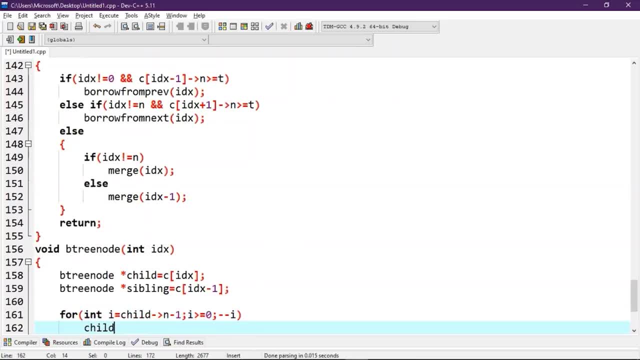 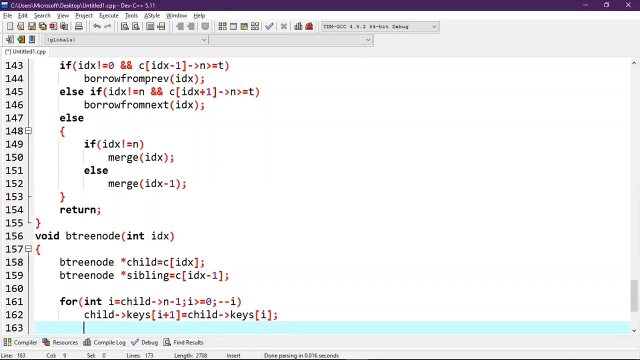 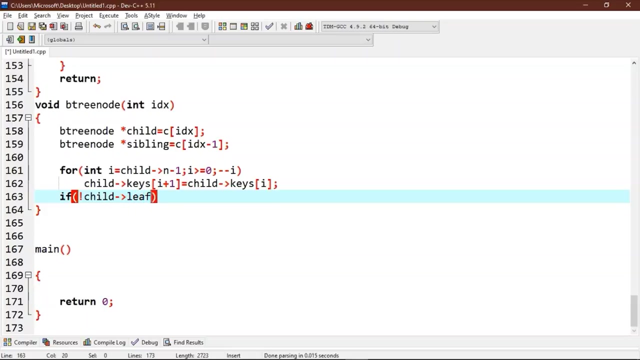 child calls keys at i plus 1. child calls keys at i plus 1. Now, if CIDX is not a leaf, then we'll move all its child pointers one step ahead. If underscore child calls leaf or int, i equals to child, then i greater than equals to zero. 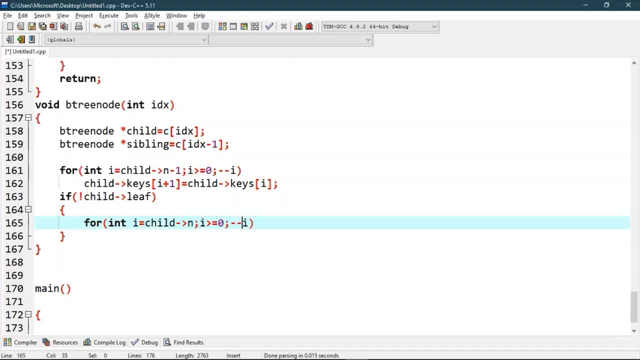 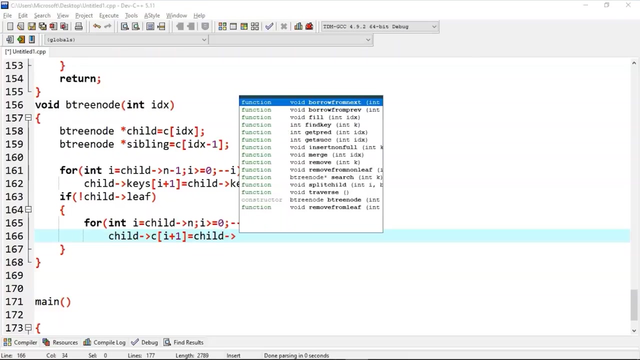 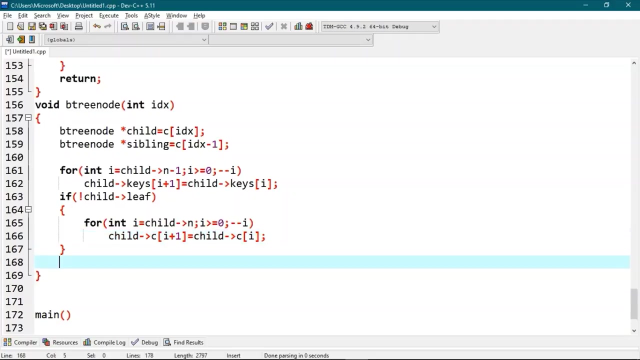 i minus minus i. child at C bracket i plus one equals to child C bracket i. Now we will set the child's first key equal to the key at IDX minus one from the current node. So child is at zero is equals to keys at IDX minus one. 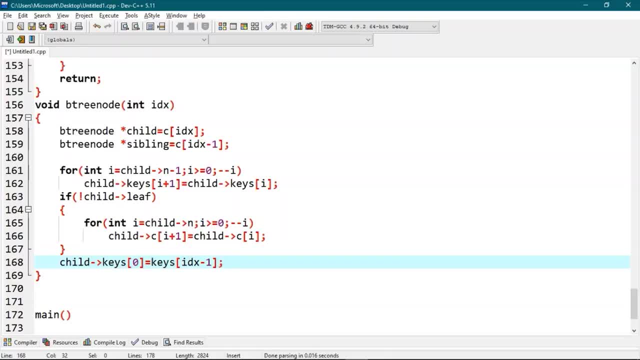 Now we will move sibling's last child as CIDX's first child. So if child is not leaf, then we will move child at C bracket i plus one from the current node. Now we will move child at C bracket i plus one from the current node. 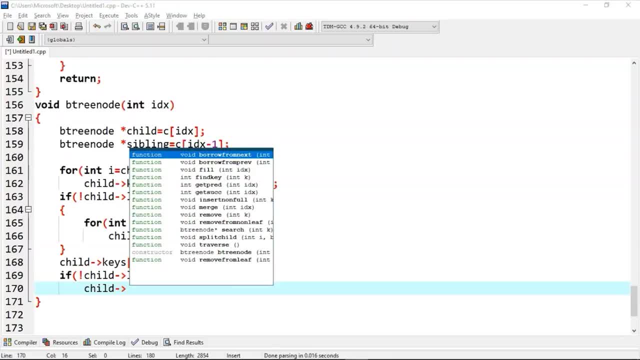 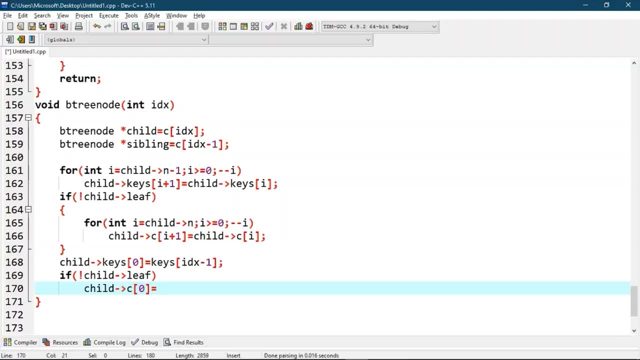 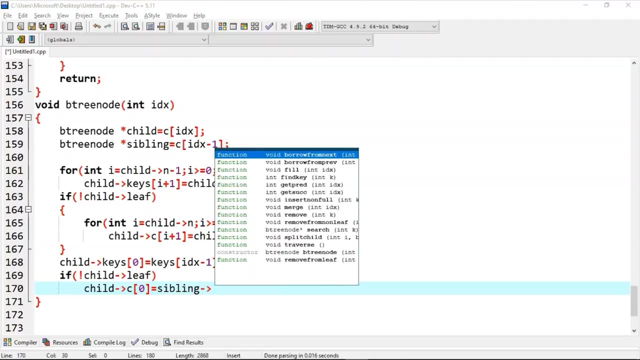 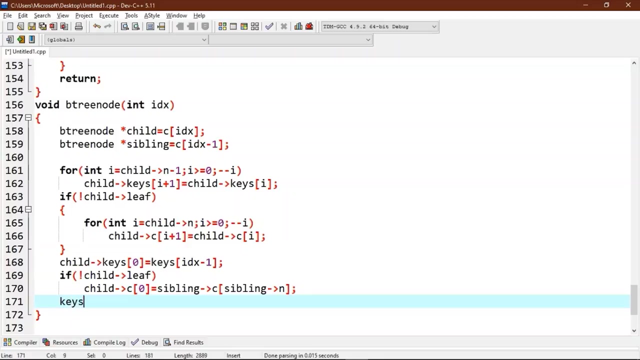 Now we will move child's first child as C bracket i child arrow. C bracket zero is equals to sibling at C. sibling calls N at C. sibling calls N. Thank you. Case at IDX minus 1 will be equals to sibling case. 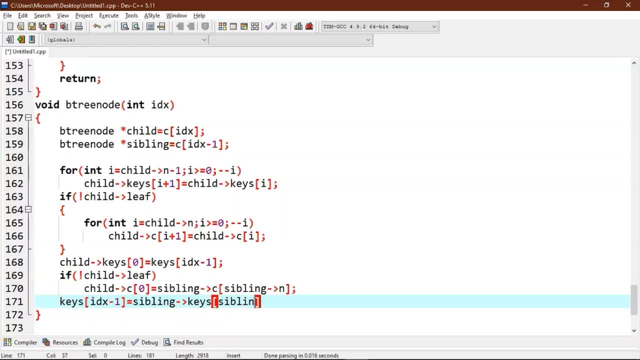 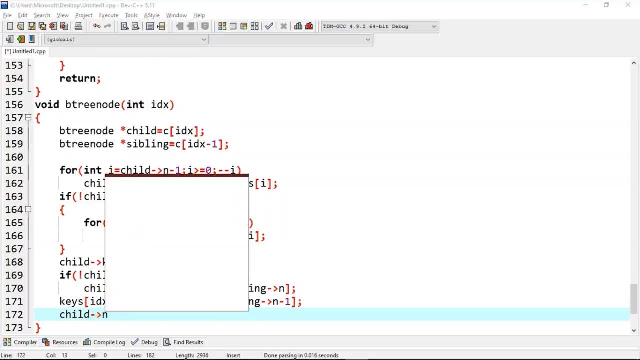 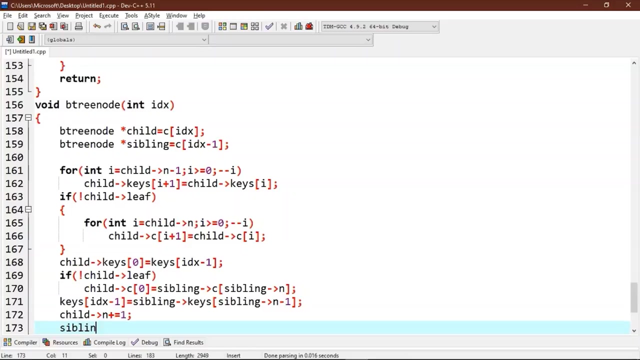 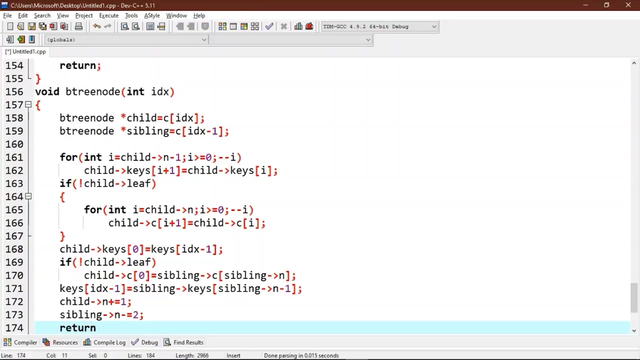 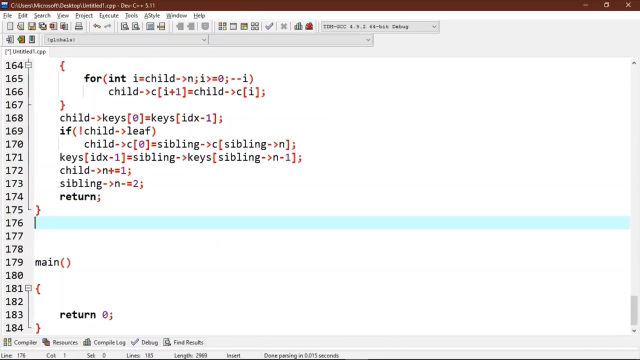 Sibling calls N minus 1.. Now, child at N will be plus equals to 1.. Sibling calls N minus 1.. Sibling calls N minus 1.. And sibling N will be equals to minus equals to 1.. Return void B3.. 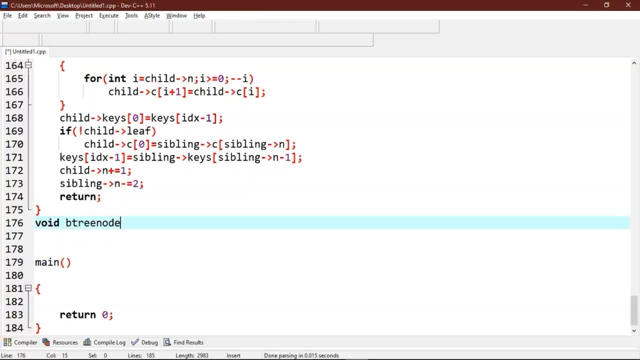 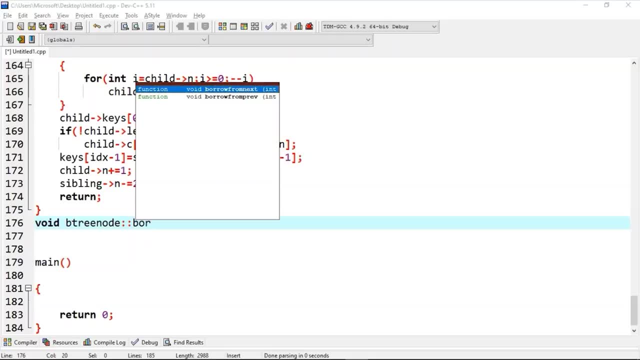 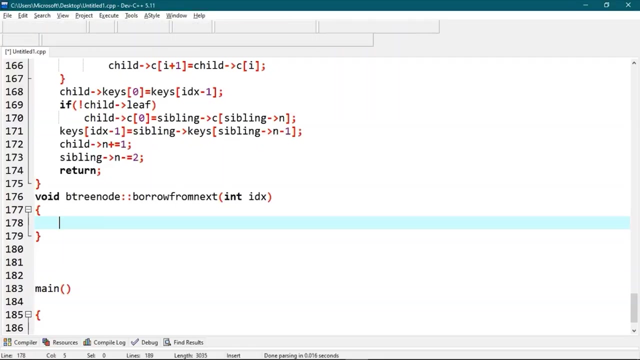 Return void B3.. Note Borrow from next: I am D IDX. Now we will start by B3, node child is equals to C at IDX And B3, node sibling. Return void B3. Is equals to C at IDX plus 1.. 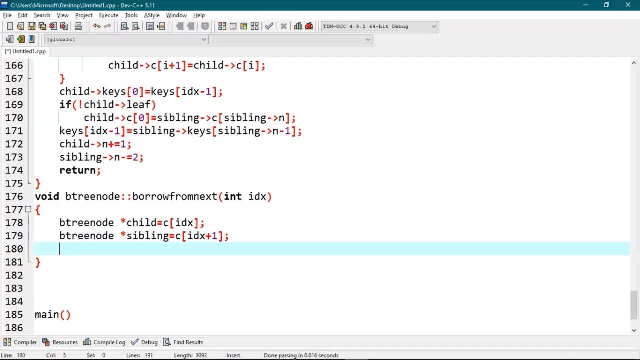 Now key IDX is inserted as the last key in the C IDX. So child Keys, Kids, Kids, Kids, Kids, Kids, Kids And And delays we are called will be under CEIC, Nevit Hartman. 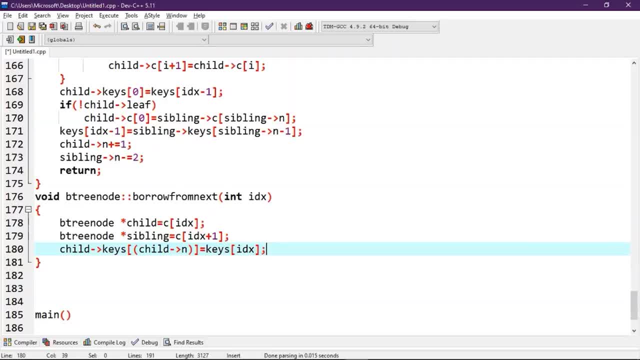 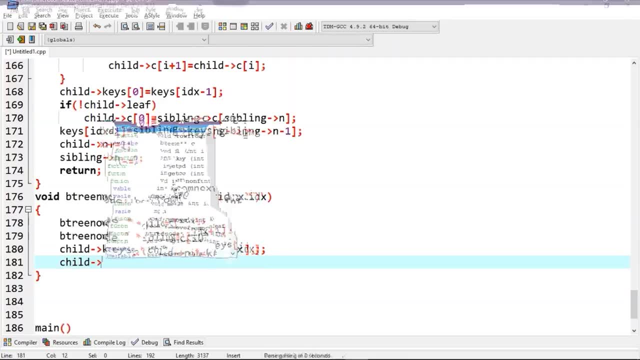 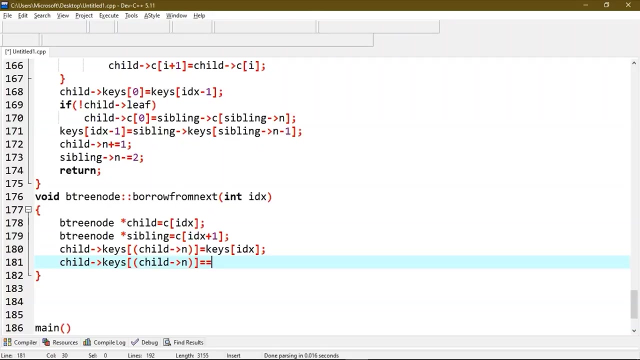 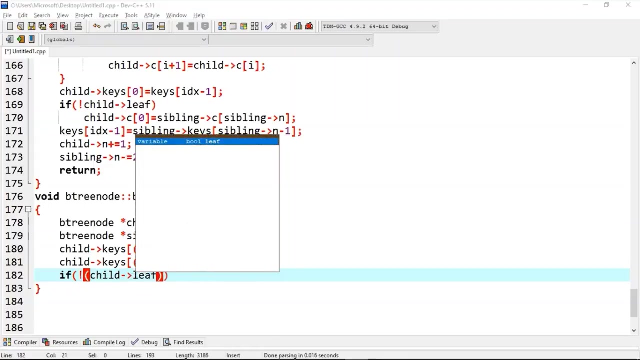 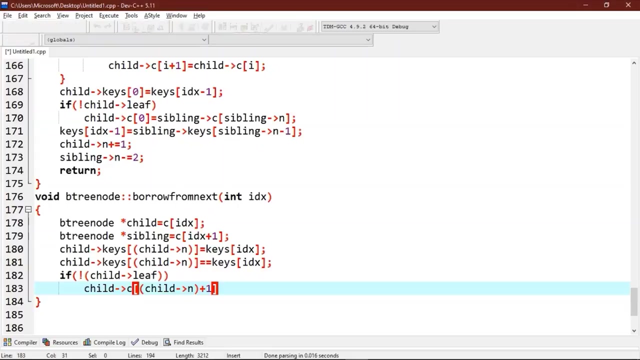 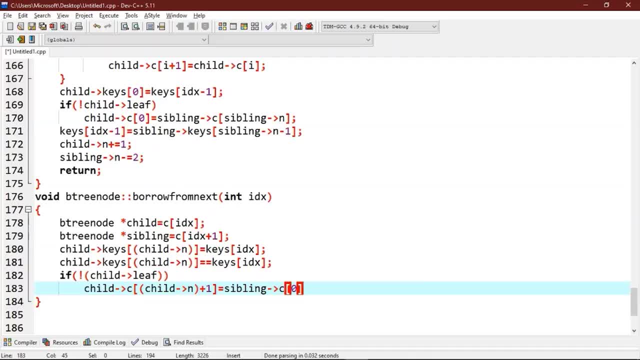 equals to sibling at c zero. now the first key from sibling is now the first key from sibling is now the first key from sibling is inserted into key idx. inserted into key idx. inserted into key idx. so key at idx, so key at idx. so key at idx is equals to: 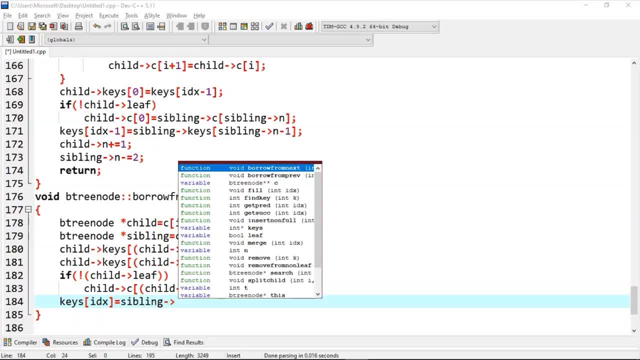 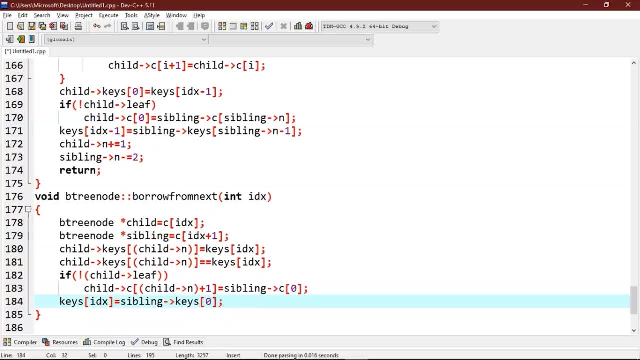 is equals to is equals to sibling keys: zero for loop and for loop and for loop. and i is equals to one. i is equals to one. i is equals to one. i less than i. less than i. less than sibling at n plus plus i sibling. i minus one, i minus one. 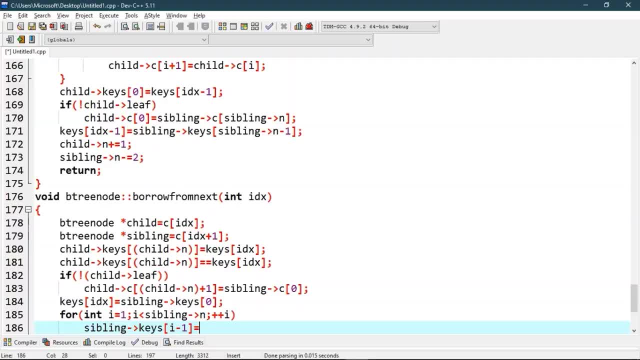 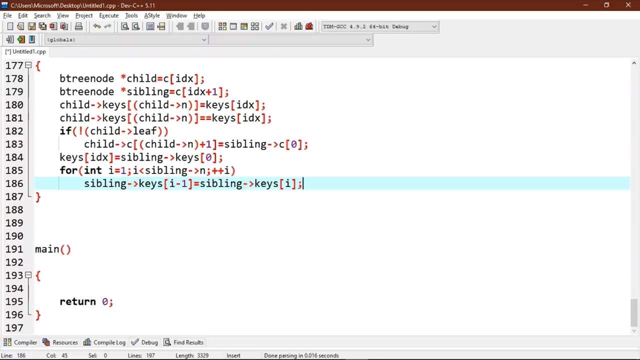 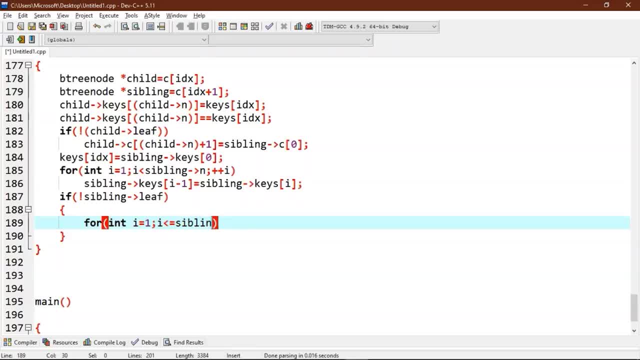 sibling calls and plus-plus I C at i-1 equals to sibling calls C at i. Now we will be increasing and decreasing the key count of C? idx and C? idx plus 1 respectively. 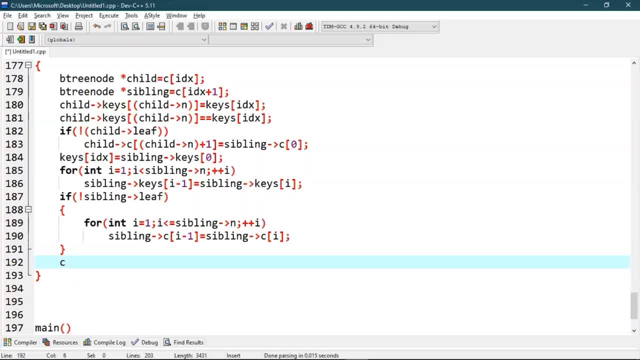 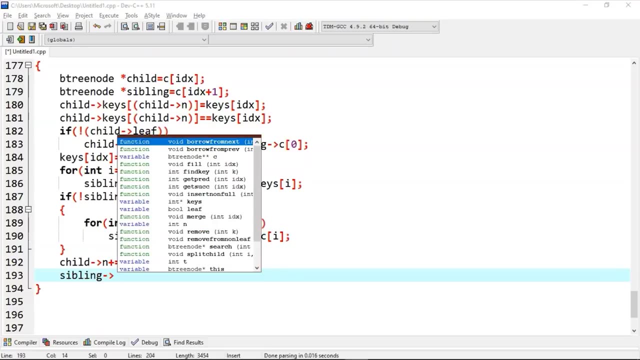 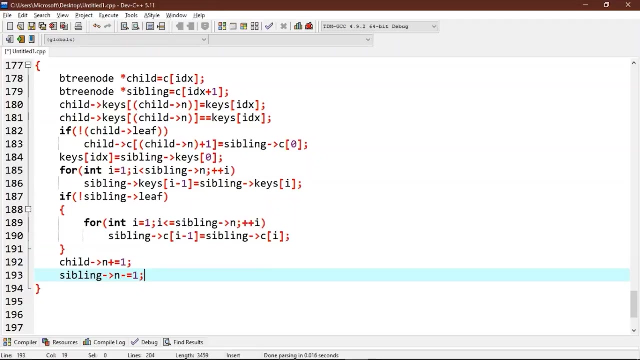 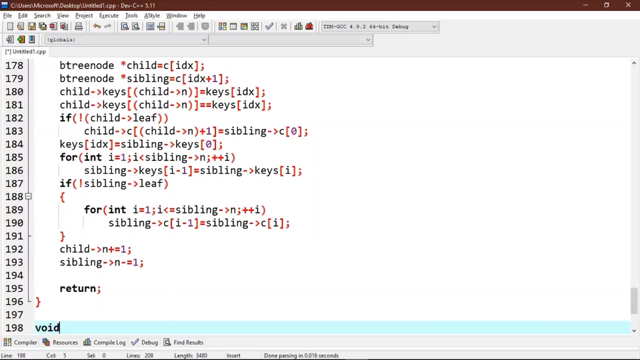 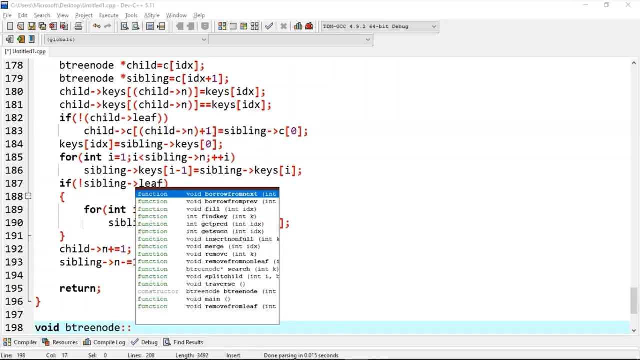 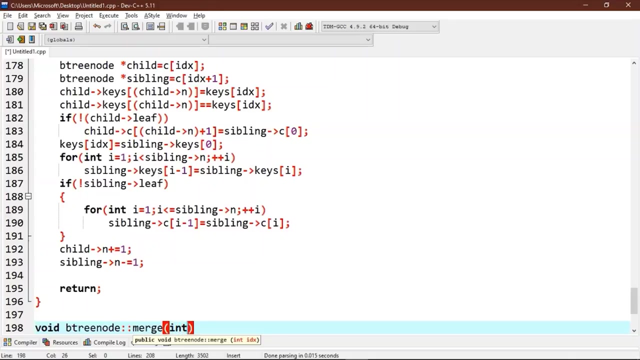 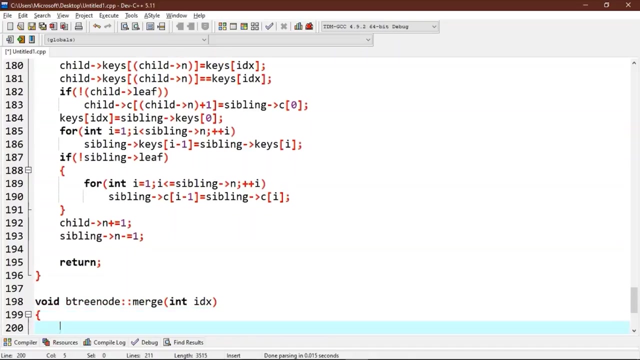 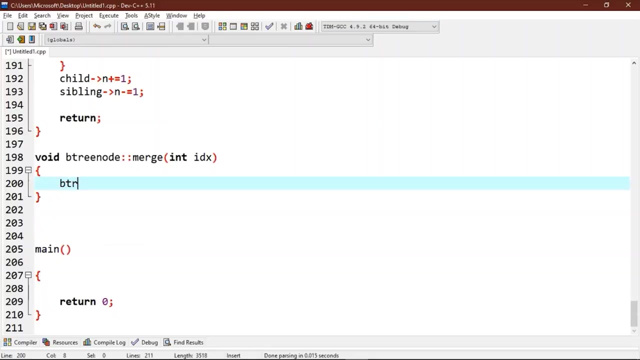 So child at n is plus equals to 1. Sibling calls n minus equals to 1. Return. Return Now void btree node merge with argument as int idx btree node star child is equals to C idx btree node, star sibling. 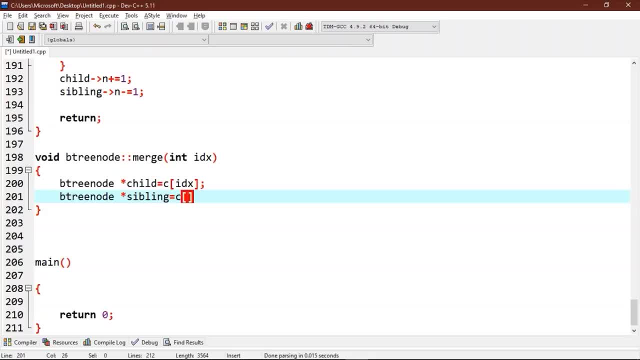 btree node, star sibling, is equal to c at idx plus 1.. Ok, now in this case we have d: 1 in addition to c at t-1.. Now we will be pulling a key from the key node and inserting it at t-1th position in C idx. 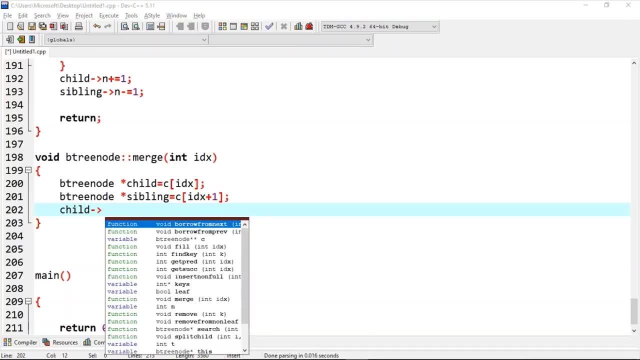 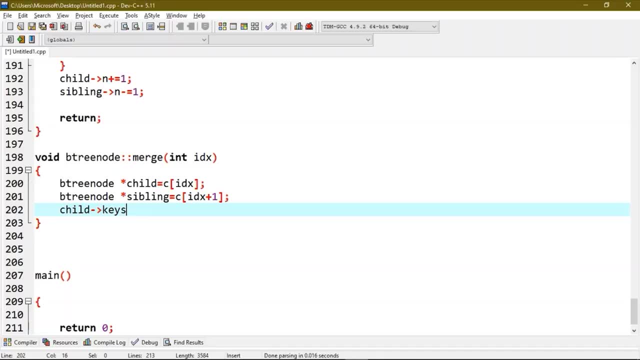 So child calls: keys at n minus equals to c, t-1 is equals to keys at idx. now we will be copying keys from cidx plus 1 to cidx at the end. so for int i is equals to 0, i less than sibling equals n and plus plus i. 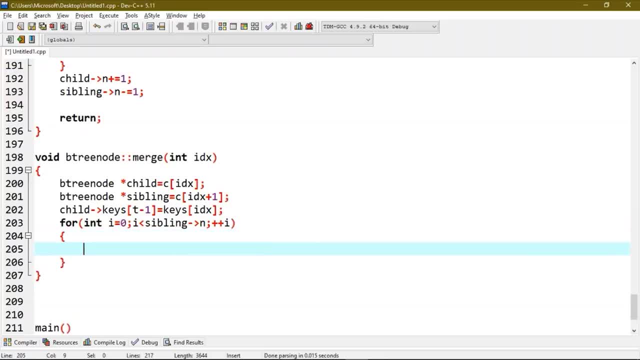 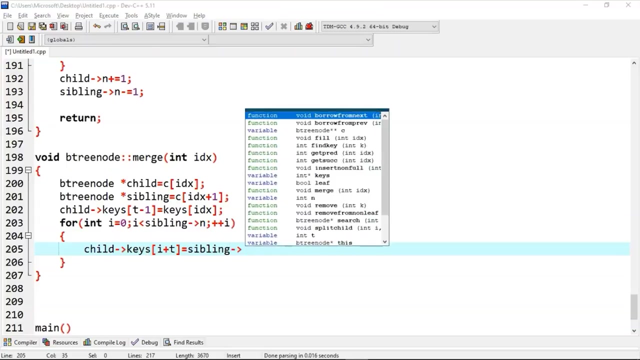 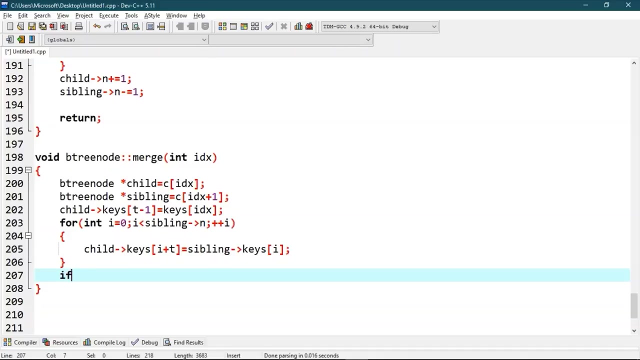 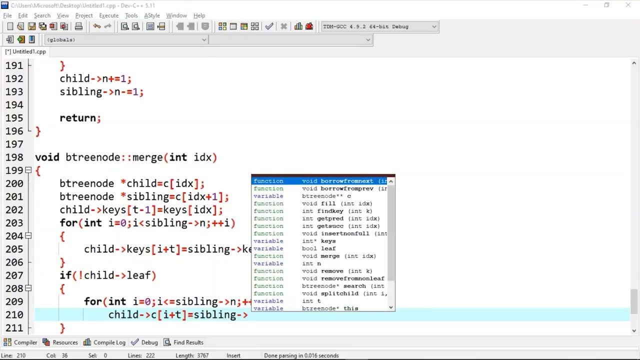 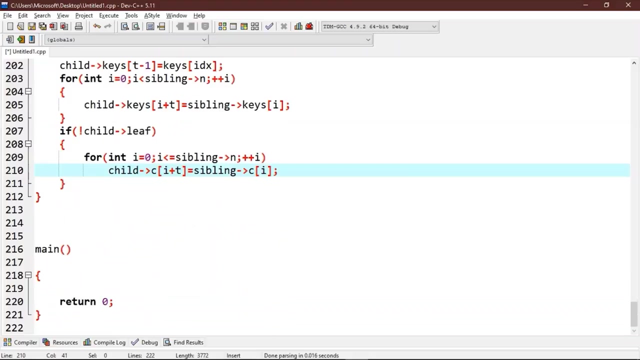 so child i plus t equals to sibling i. if our child calls leave for i, is equals to 0.. i less than equals to to sibling calls s plus i. child calls c bracket i plus t goes to sibling calls bracket i now for and is equals to ID x plus 1. 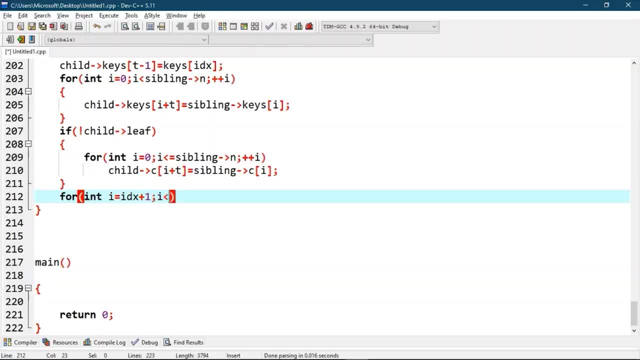 and is equals to ID x plus 1. and is equals to ID x plus 1. i less than n plus plus i. i minus 1 is equals to keys at i or int. I is equals to ID x plus 2. i less than equals to n. 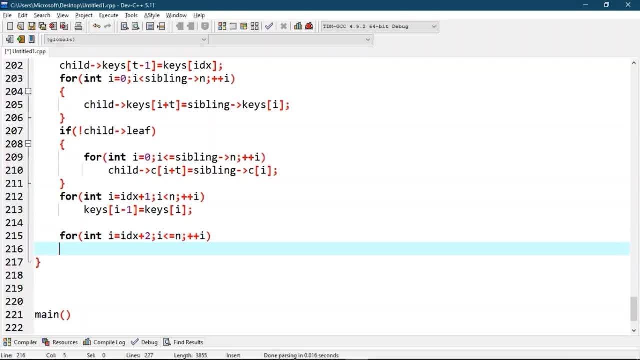 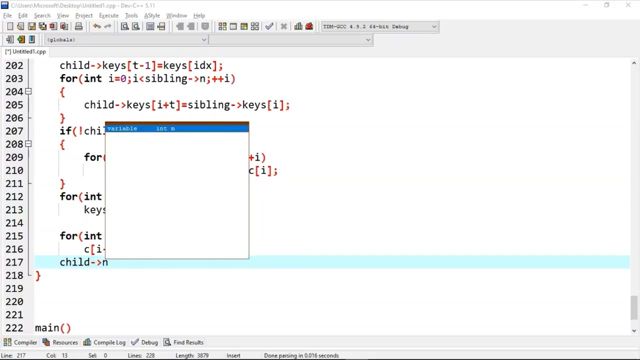 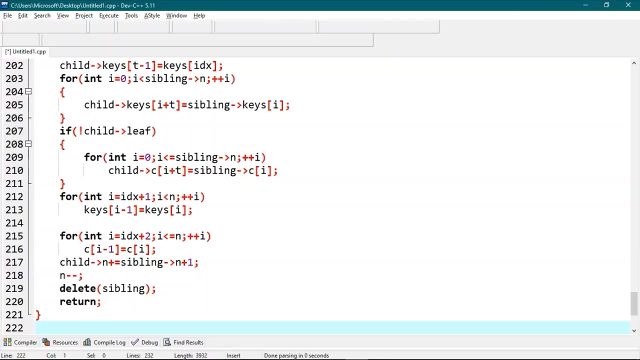 and plus plus i. c at i minus 1 is equals to c, is equals to c, c c at i at i in in n n plus n plus equals to n. plus equals to sibling, sibling n plus 1 plus 1. now we will write the main function that inserts a new key in this b-tree. 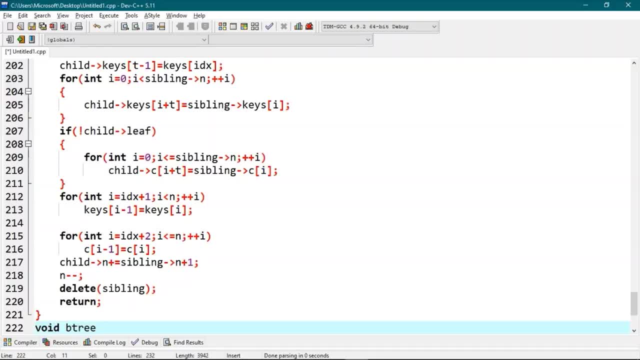 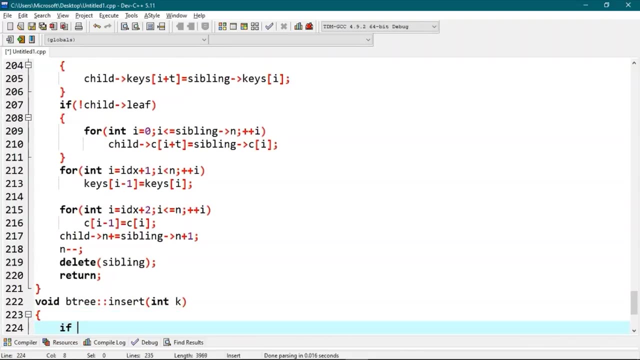 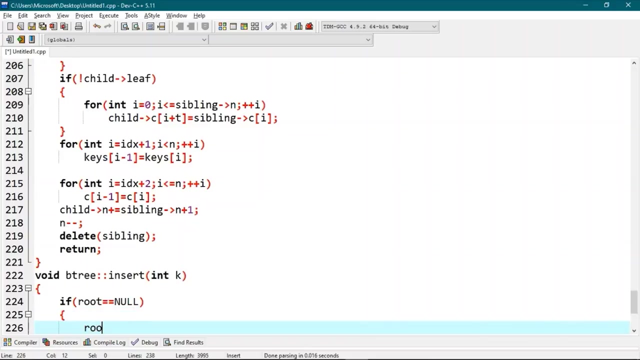 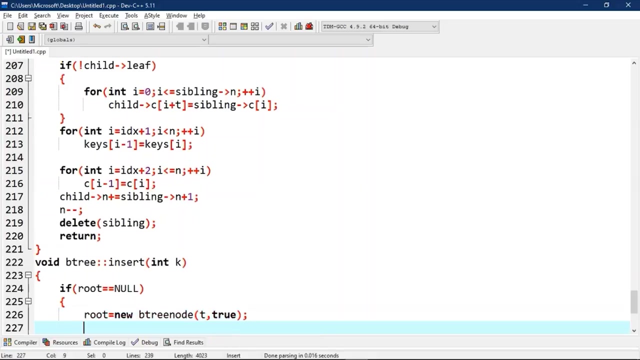 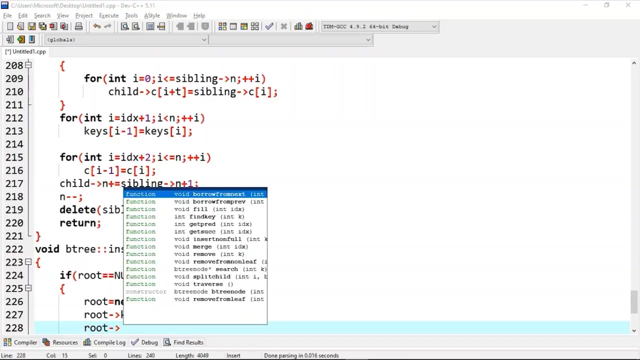 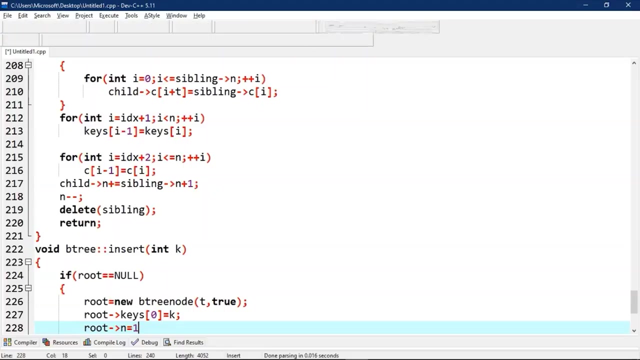 to void b-tree int k. if root is equals to null, then we will allocate memory to: root is equals to new b-tree node d comma. true root is equals to new b-tree node bracket. zero is equals to k and root at n is equals to one. 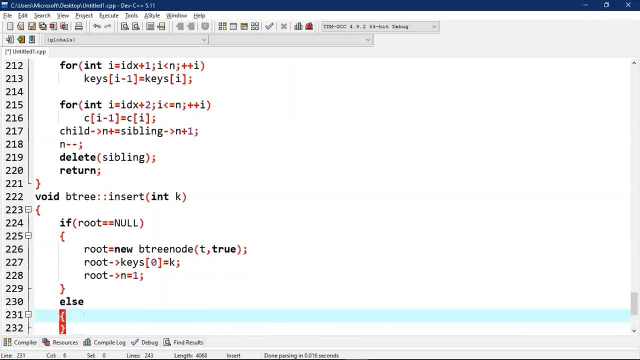 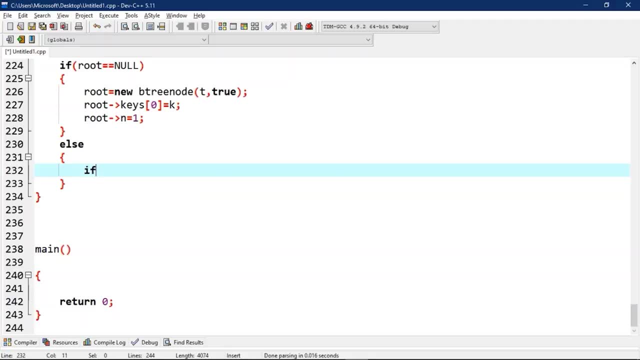 else, if root calls n is equals to star t minus one. so btree node star s is equals to new btree node e, comma false. now s c bracket zero is equals to root. s is equals to new btree node. s is equals to new btree node. 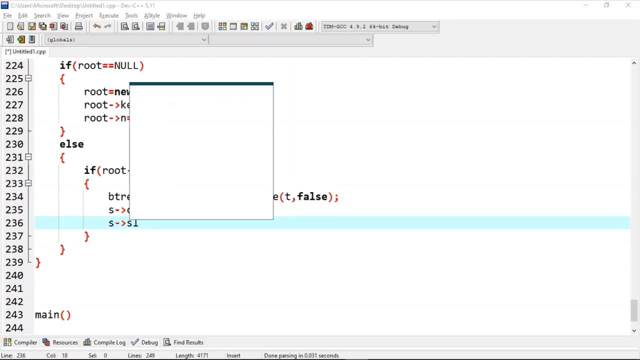 now s c bracket zero is equals to new btree node s s split child, child, child zero, comma zero. comma zero comma root, and, and and i is equal to zero. if, as as as as keys, keys, keys bracket 0 less than k, i plus plus s c. 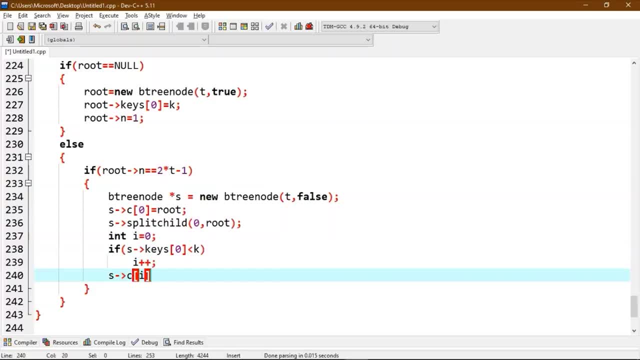 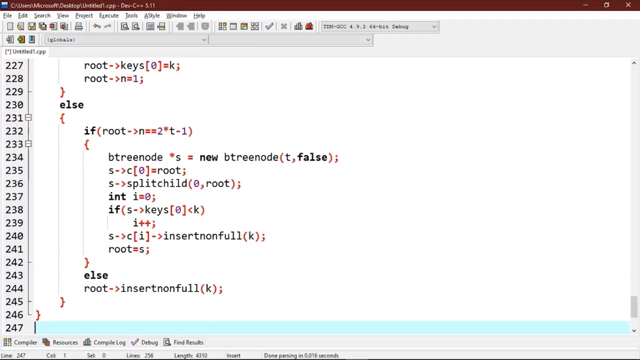 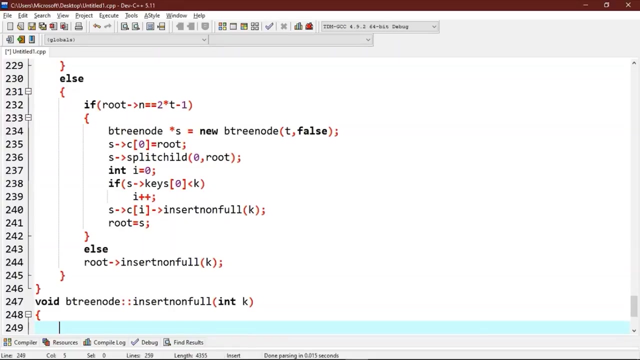 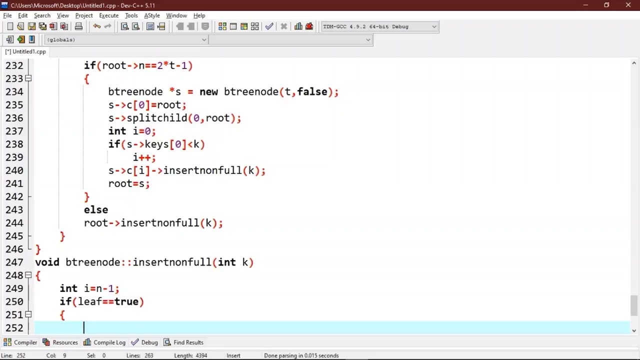 bracket i insert nonpol k. now we will change the root to s, else root calls insert non-full at k, a utility function to insert at non-full node. so int i is equals to n minus 1 if leaf equals to true. the following loop does two things: 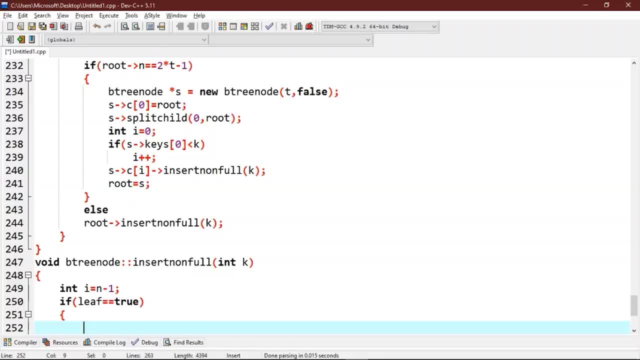 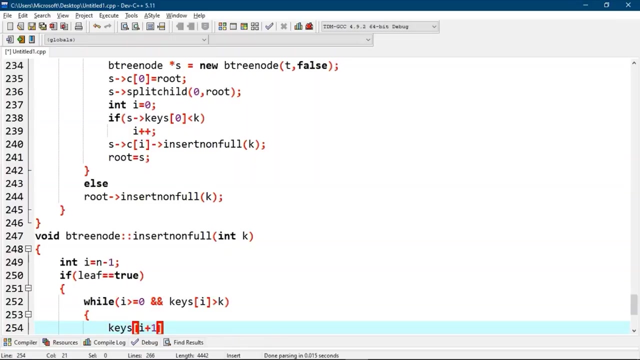 finds the location of key to be inserted or moves all greater key to one place ahead. so if leaf equals to true, the following loop does two things. so while i is greater than or equals to 0 and keys at i are greater than k, then keys at i plus one will be equal to keys at i. 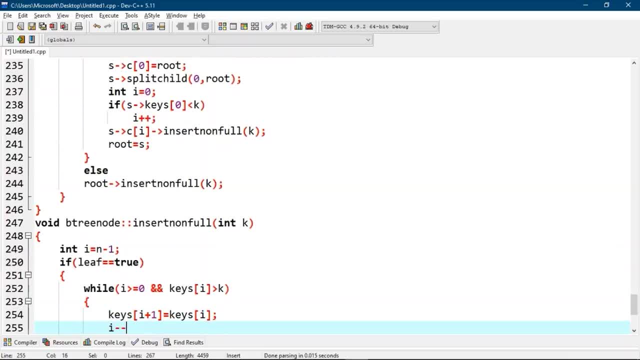 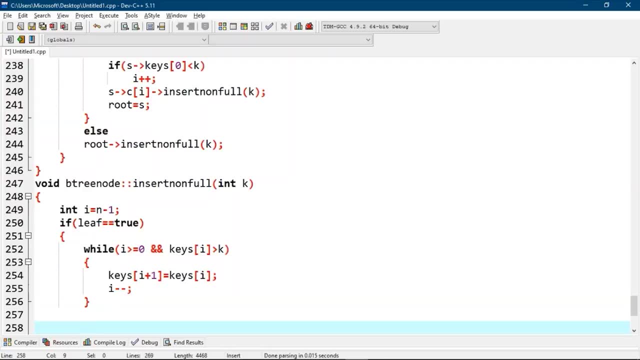 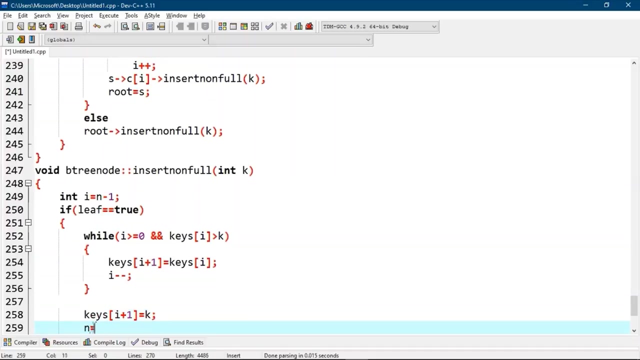 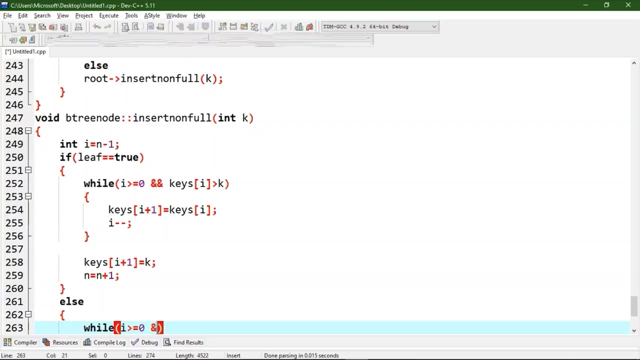 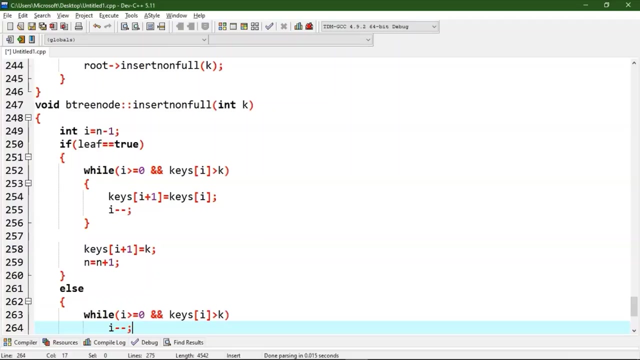 and I minus minus, Keys at I plus 1 will be equals to A and N will be equals to N plus 1.. Else, while I is greater than equals to 0 and keys at I is greater than K, I minus minus. If C bracket, I plus 1. 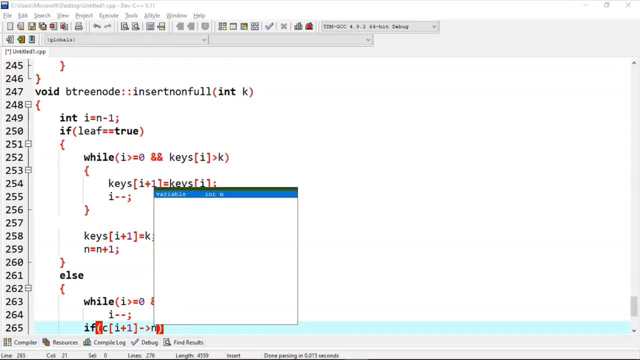 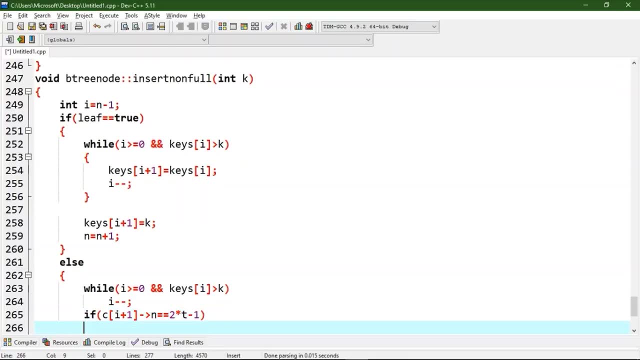 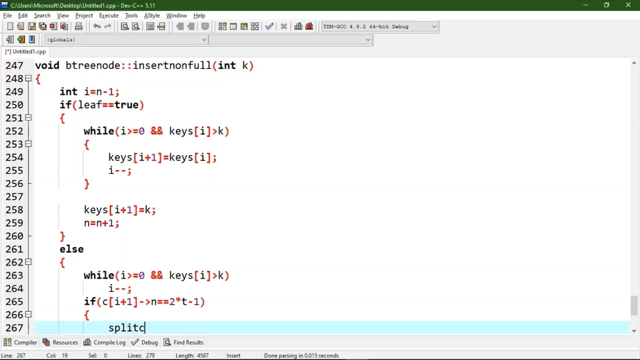 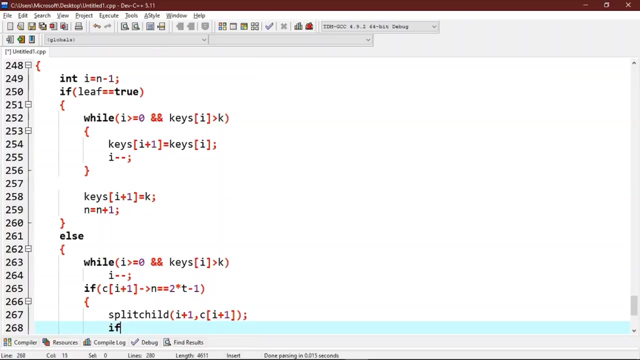 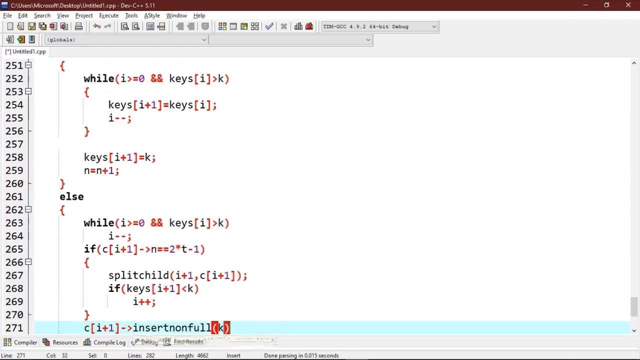 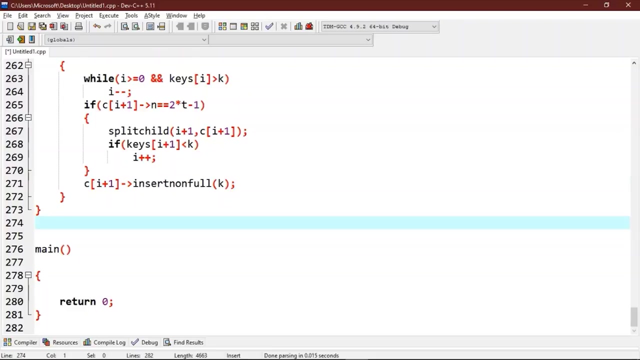 at N equals to 2 star T minus 1 at child I plus 1. comma C I plus 1. F is bracket I plus 1. K I plus plus C. bracket I plus 1. insert non-full K void B3 node int I comma. 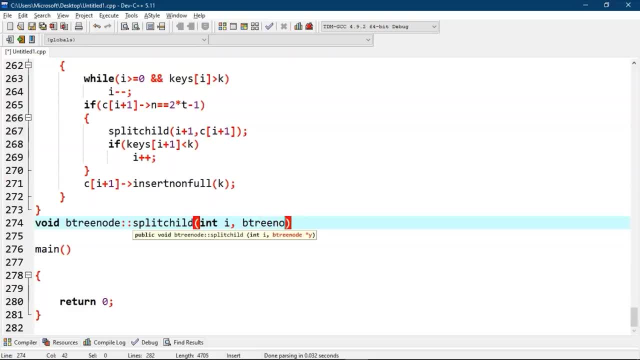 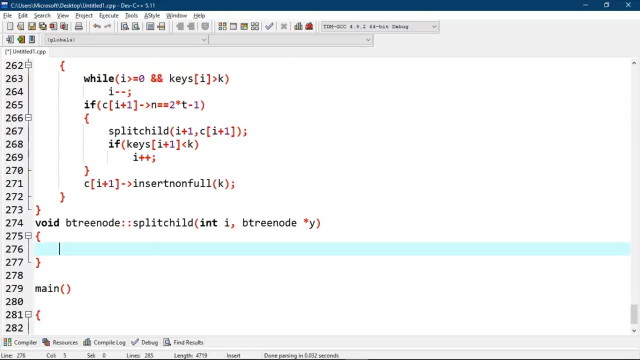 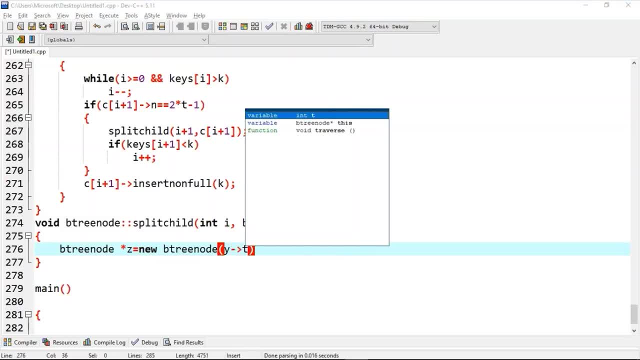 K. I plus 1 K. I plus 1 K, I minus 1. and y calls leave. now z calls n equals to t-1. now we will copy the last t-1 keys of y to z, so for loop. and j is equals to 0, j less than e minus 1, j plus. 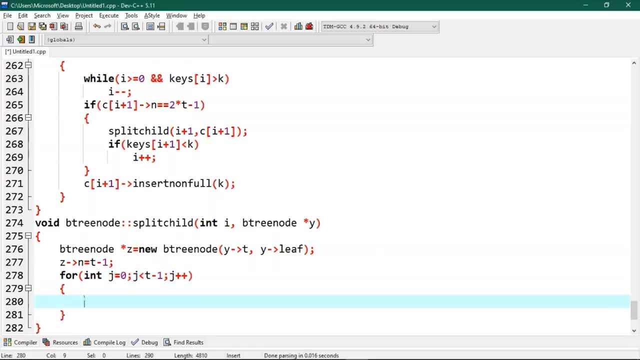 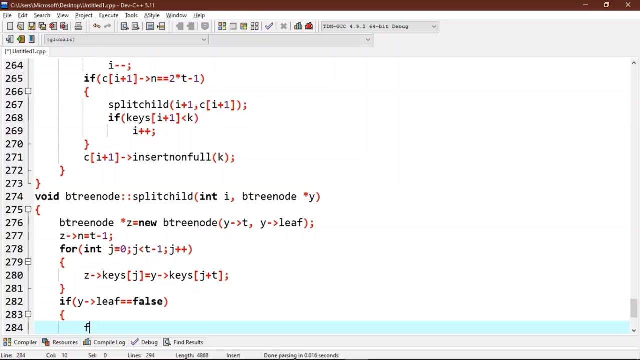 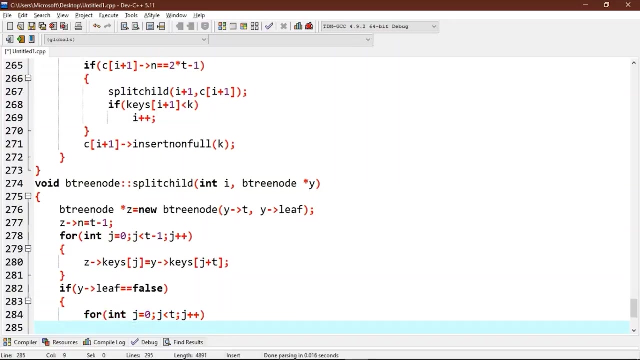 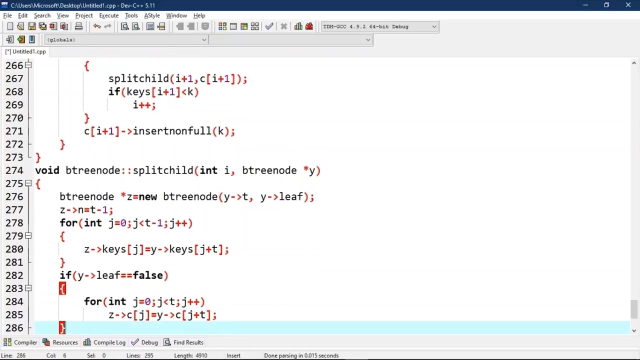 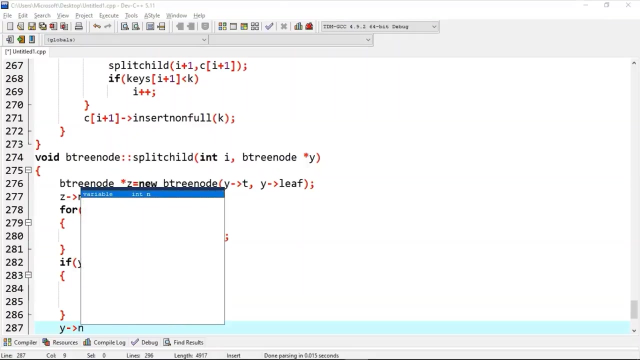 plus. so z keys a is equals to y at keys j plus t. so if y, if equals to false for int, j is equals to 0, j less than t, j plus plus j. c bracket i is equals to y, calls c bracket j plus e. now y calls n equals to t minus 1. 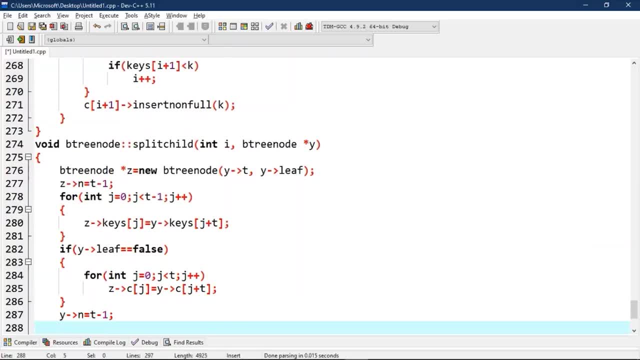 now, since this node is going to have a new child, we will create a new child and we will call it z. calls n equals to t-1 space for the new child. so for loop int j is equals to n, j greater than equals to i plus one. 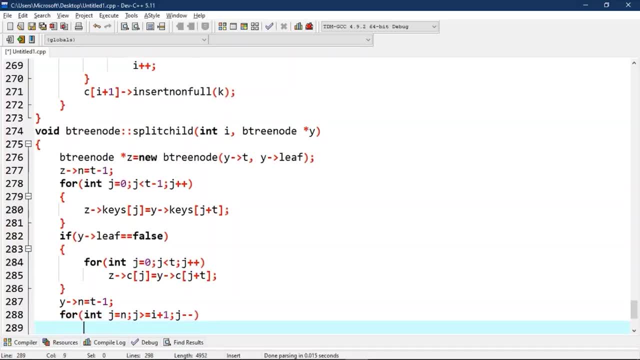 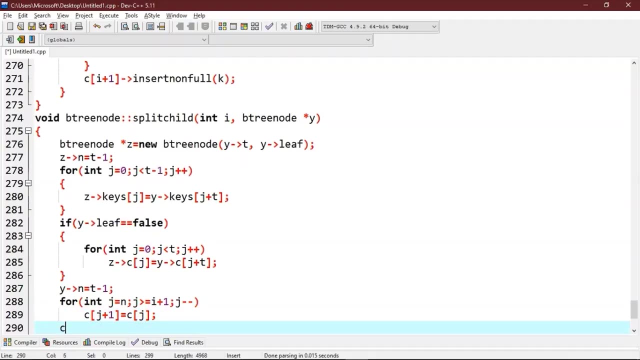 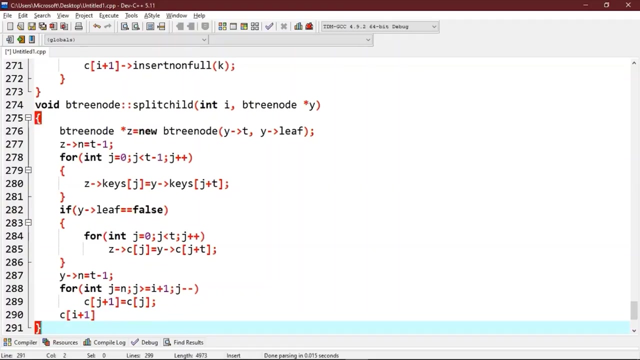 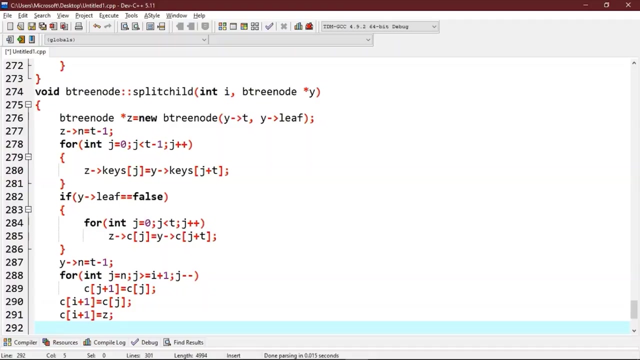 j minus minus c bracket j plus one equals to c bracket. J of C bracket I plus one is equals to C bracket J. C bracket I plus one is equals to Z. now for loop, and J is equals to N minus one. J greater than equals to I. J minus minus. 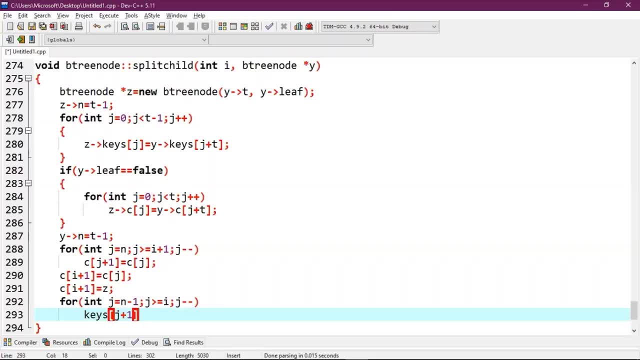 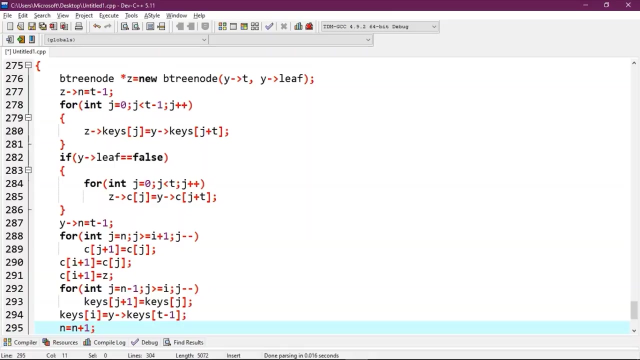 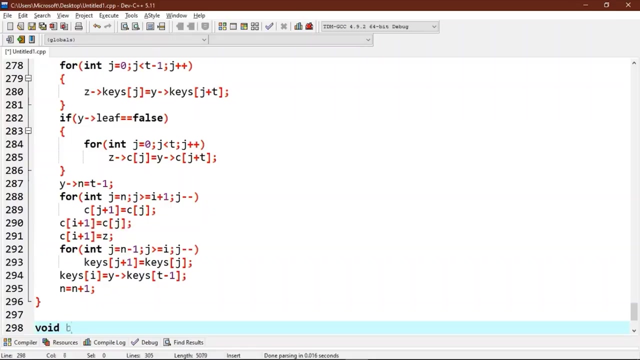 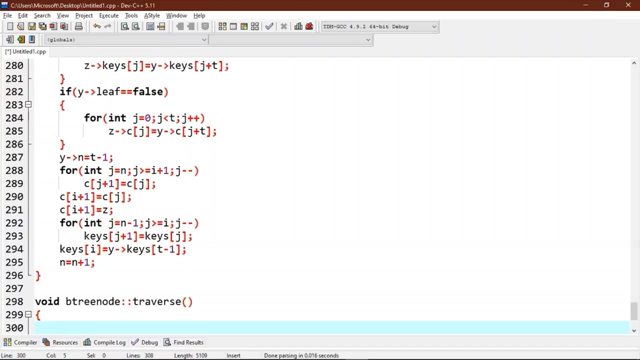 is record. J plus one equals to keys at J, J greater than equals to I, J minus minus is I equals to Y, is bracket T minus one and is equals to N plus one. now we will write function for traverse. so void B, tree, node, traverse and I. 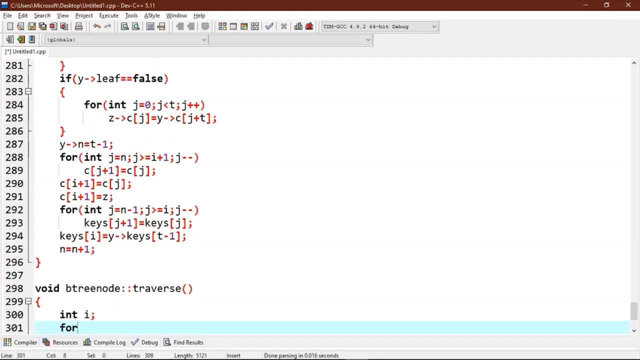 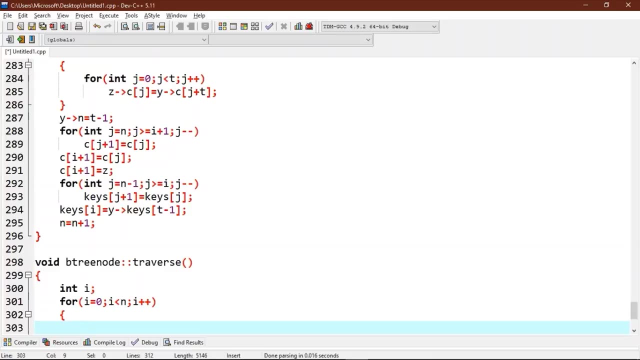 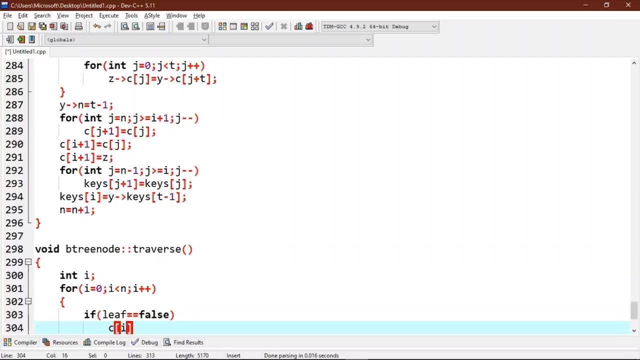 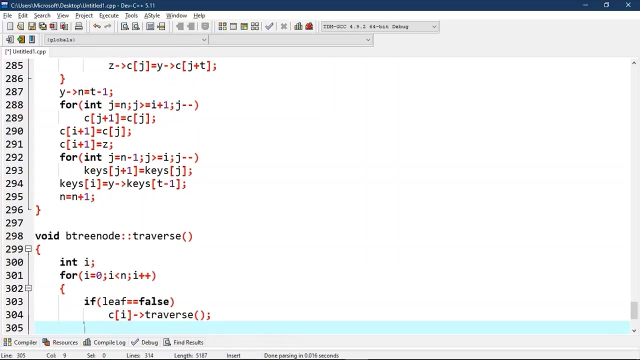 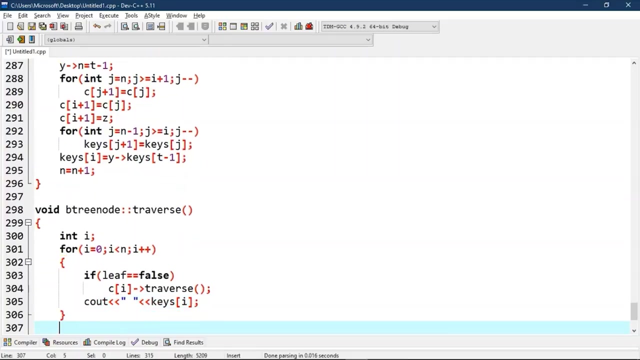 for loop: I is equals to zero and I is equals to zero. I less than N, I plus plus. if. leave equals to false and C bracket: I will traverse and I will traverse. will receive the falser. if, if, if. if is equals to is equals to false. 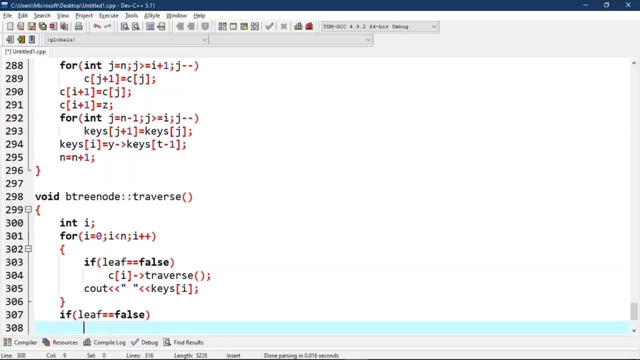 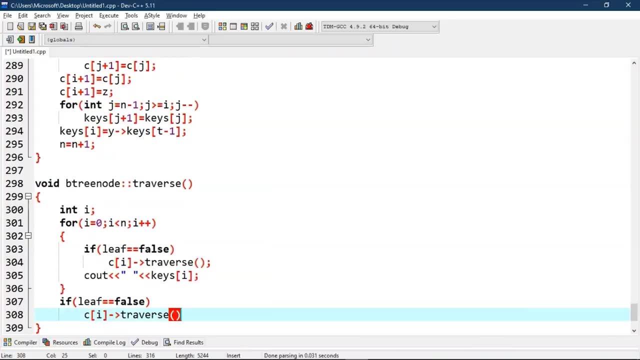 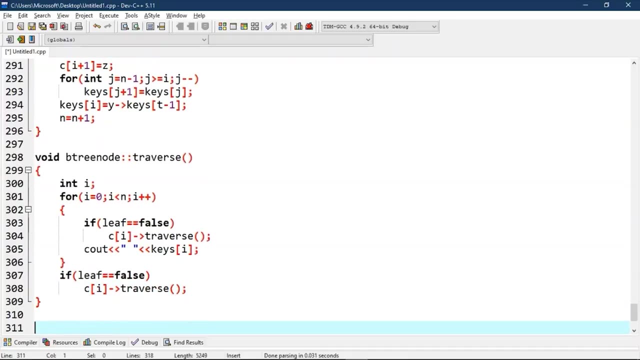 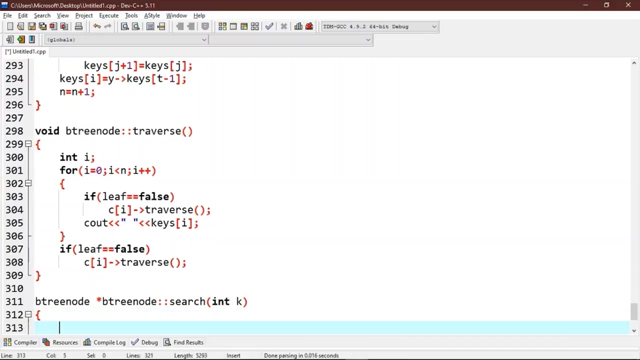 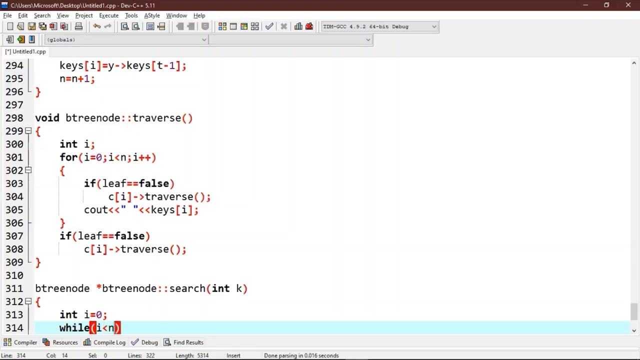 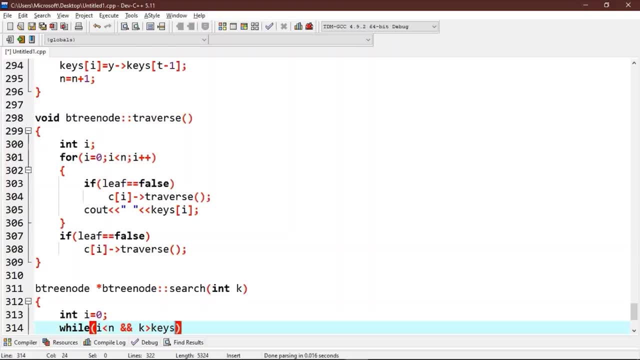 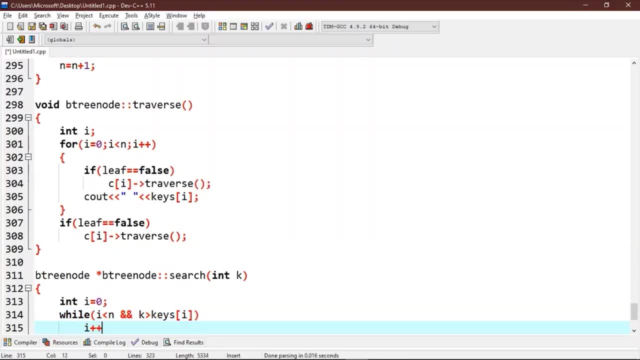 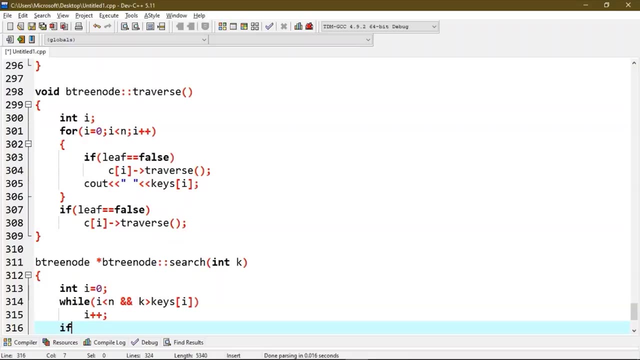 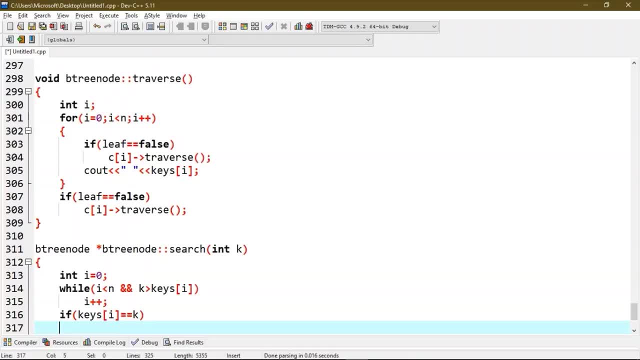 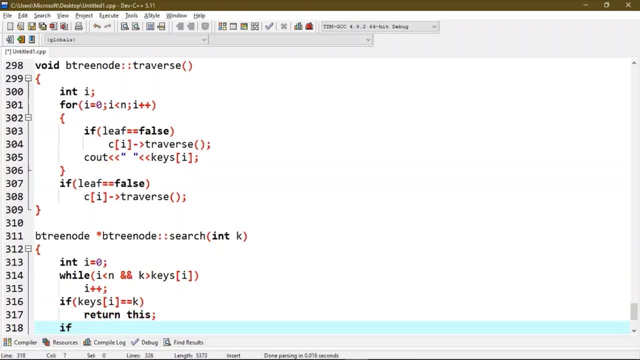 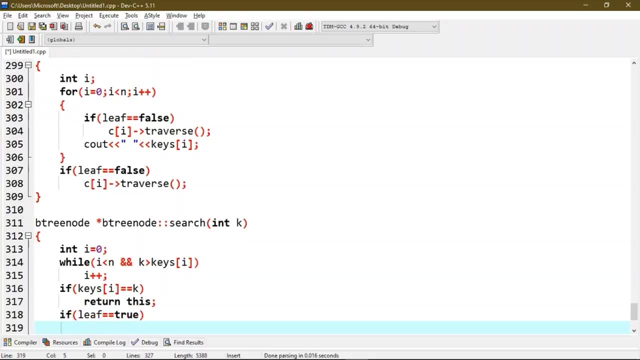 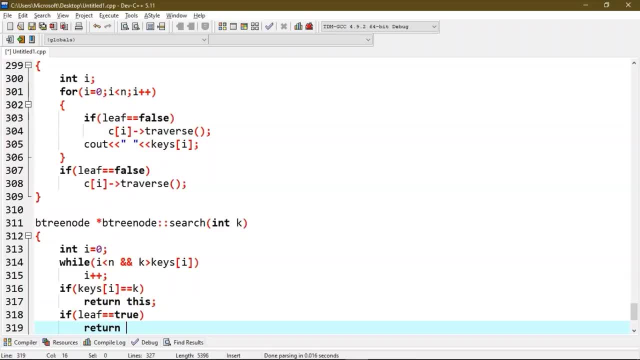 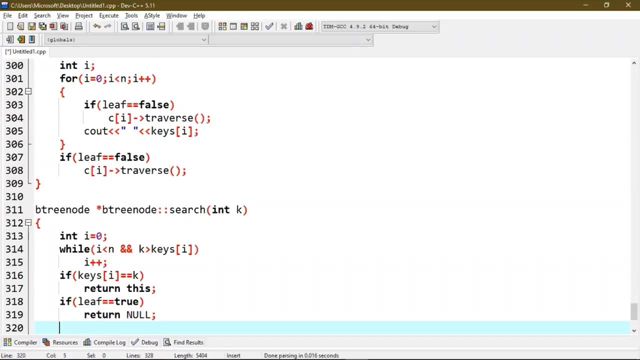 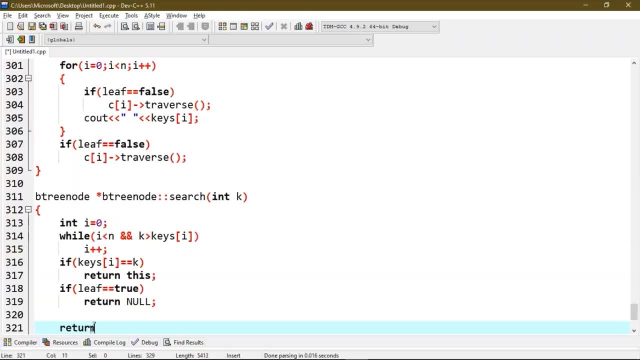 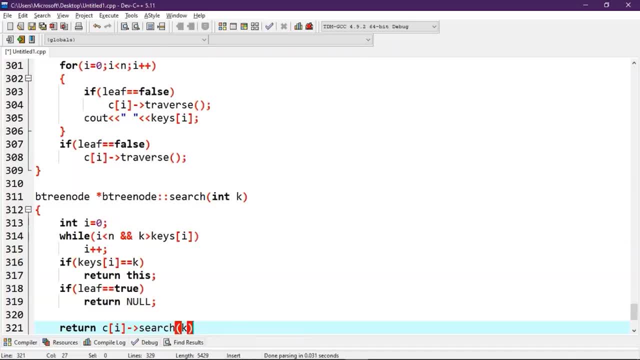 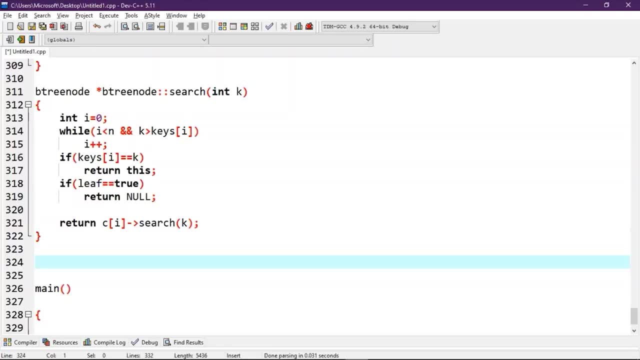 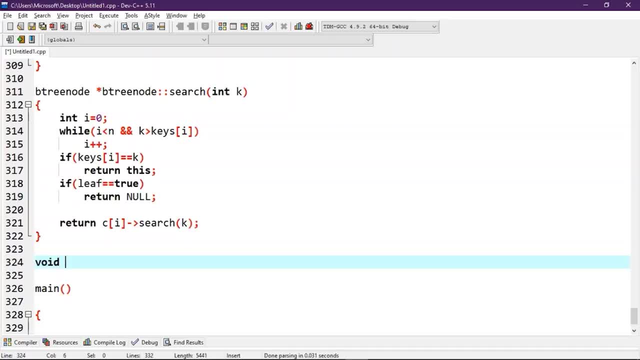 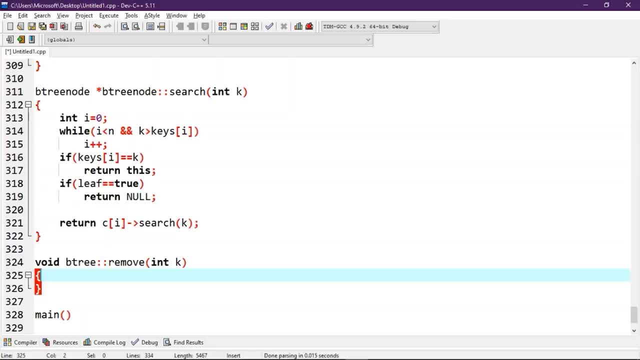 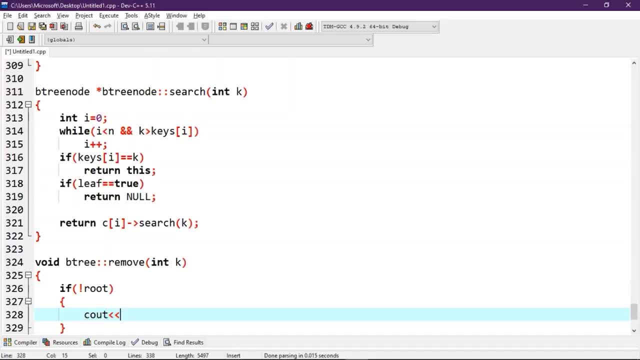 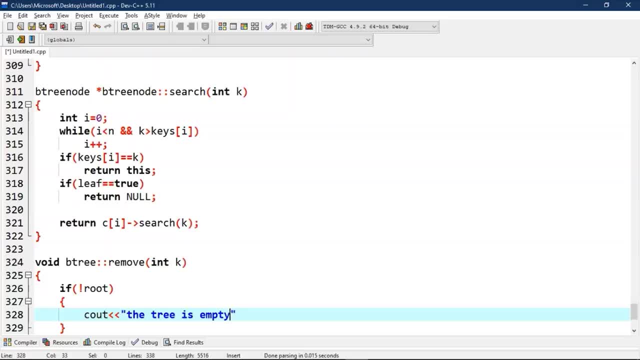 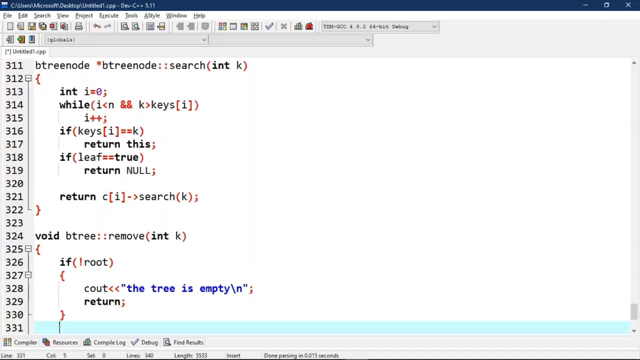 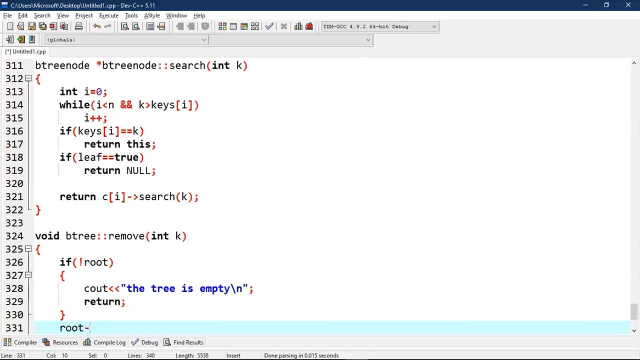 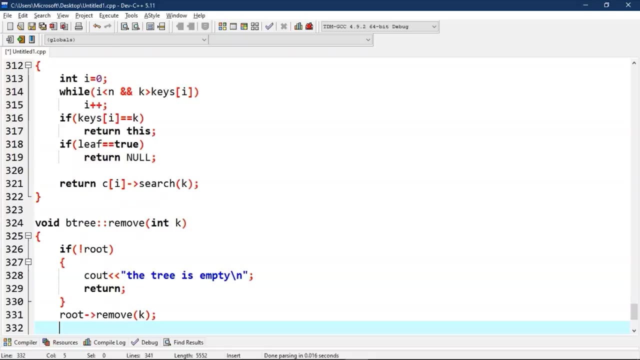 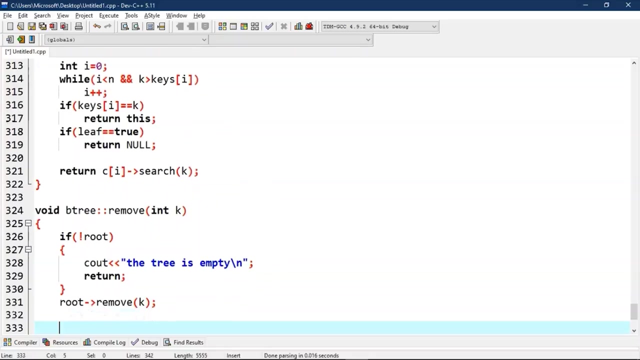 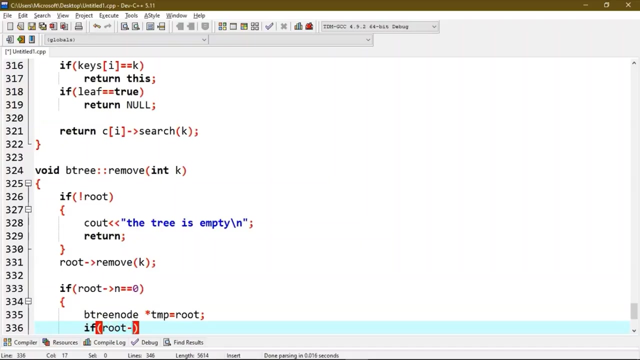 function for root. so root calls remove. okay now if root has zero keys then we will make its first child as a new root. if it has a child otherwise, set root as null. so if root n is equals to 0, can be tree node, star, DMP equals to root. if root, leave root. 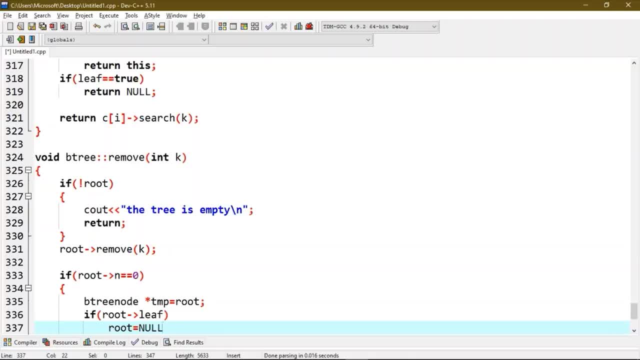 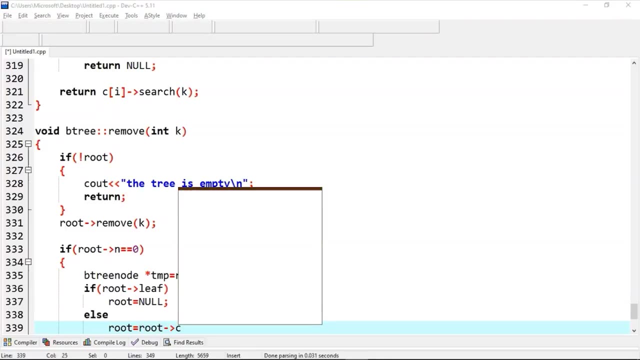 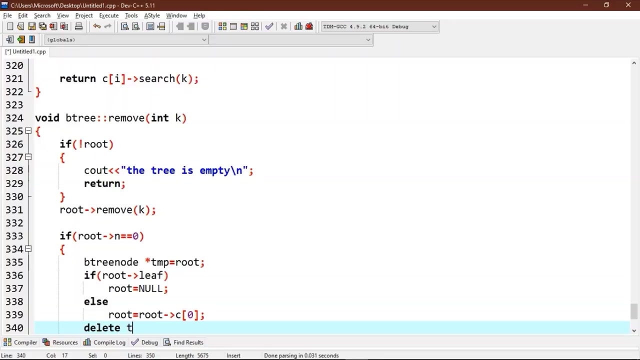 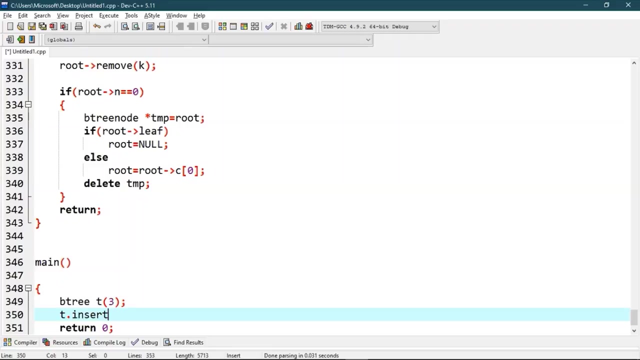 equals to null as root. equals to null as root. equals to root c. bracket 0. now delete DMP return. now we will write the code for the main block. we start with b tree of order 3. we start with b tree. we start with b tree. 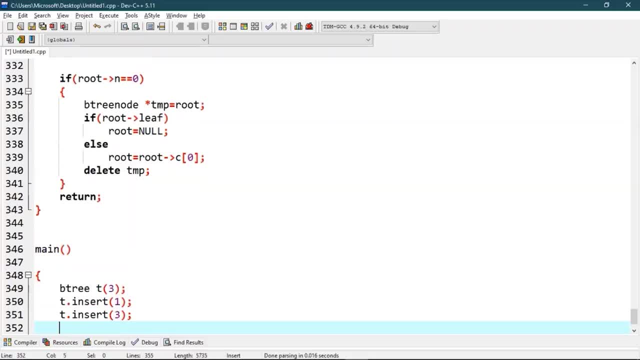 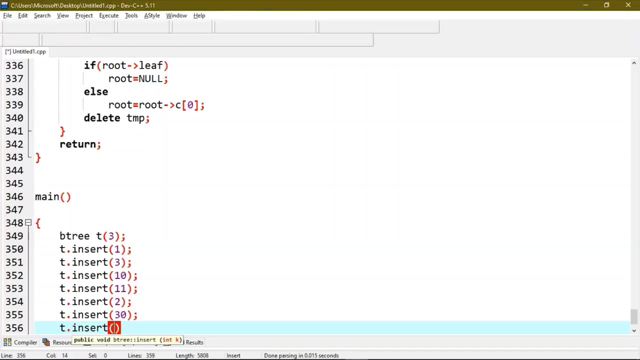 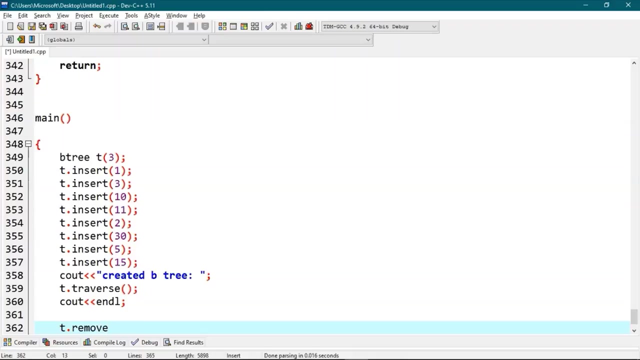 we start with b tree. so now did so, so, so, so now let's traverse this. created tree- see out, created tree out, see out. and now we will use t dot remove to remove five. now see out modified t tree after deleting five: t dot traverse. as you can see, we have. 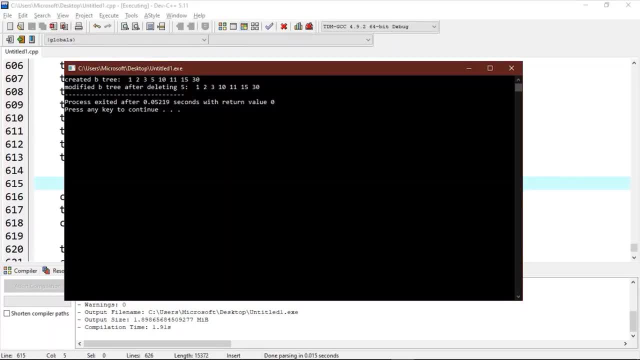 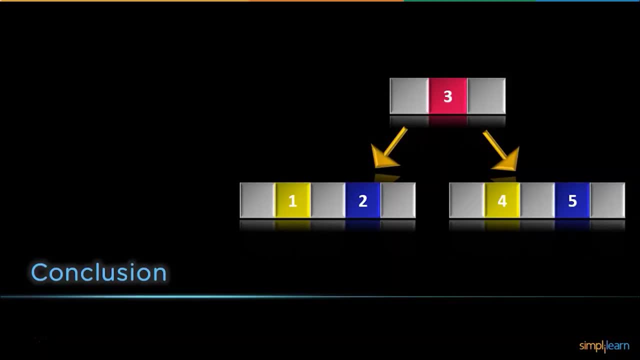 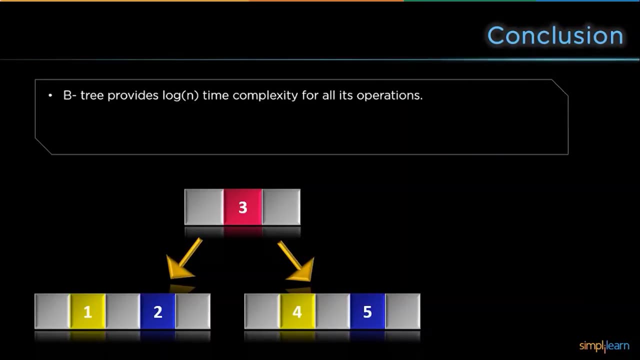 successfully deleted five from our B tree. let's get back to our slides at last. let's sum up what we have learned in this session. first up, all the operations on B tree have time. complexities of log n. next, all the leaves must be on the same level. next, elements of B tree are sorted.